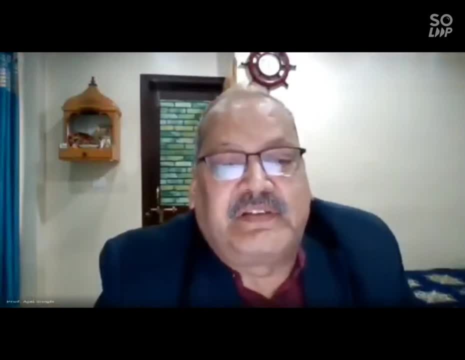 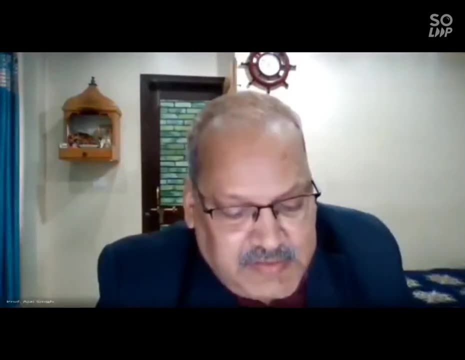 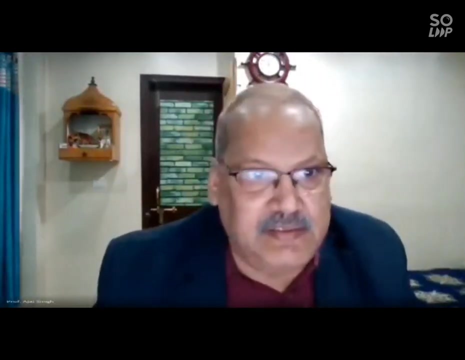 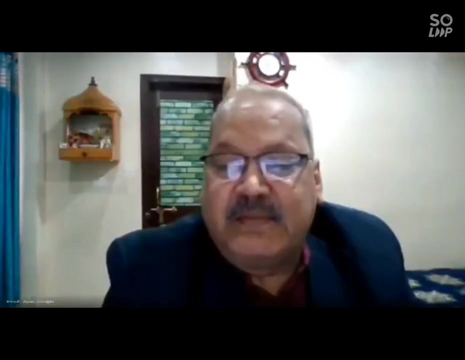 research and project officer in Center for Research and Environment, Energy and Water, and he has been working on a logical model and I thought that why not learn the experience of a person working in Nepal and how they people are doing in the area of a logical model and how they are managing the data and all those things, that what is the data limitation? and so that, keeping this in view, I thought that let us. 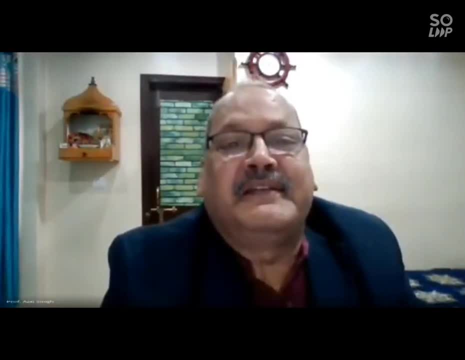 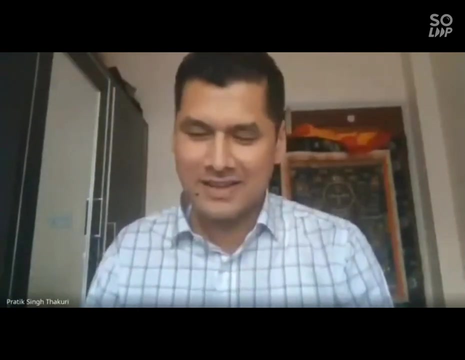 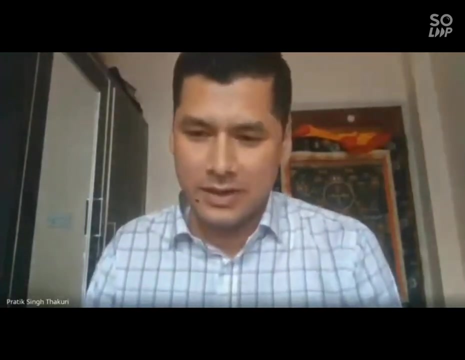 invite Mr Prateek Singh and listen to his experiences. So now the stage is yours, sir. You can start your presentation. Yeah, thank you. Thank you, Professor Ajay. Let me give more some of my information, my elaborated one. So I have recently joined in the academic field as an assistant professor in Nepal, engineering. 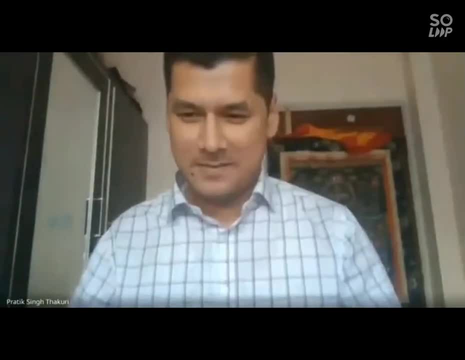 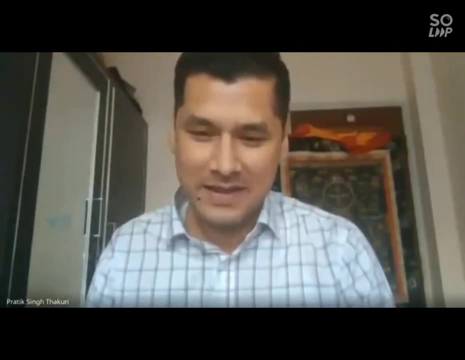 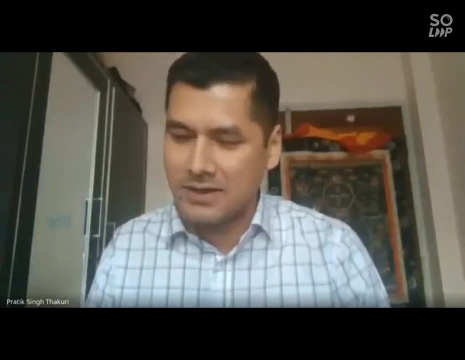 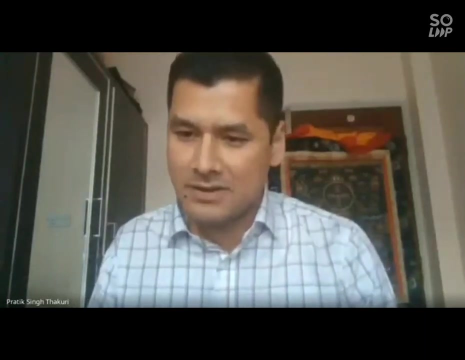 College. So, yeah, so I'm also in your club as a teacher or as a professor. Yeah, And talking about Nepalese context of hydrological modeling, data management is quite, quite similar to other South Asian countries, But the thing is in Nepal, the department of which take care of all these hydrological and metrological data are. 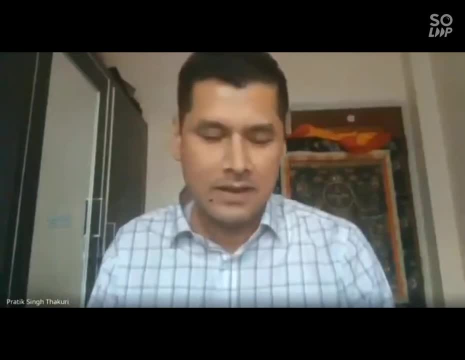 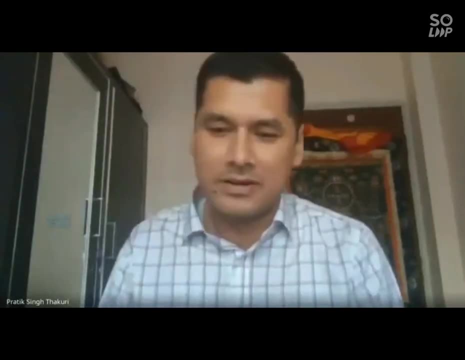 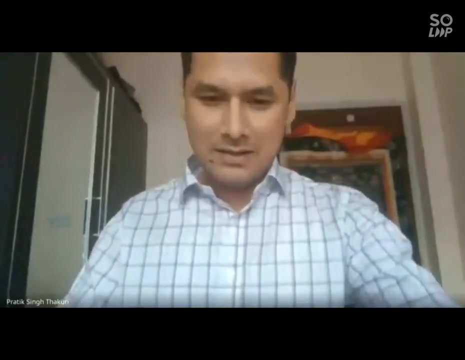 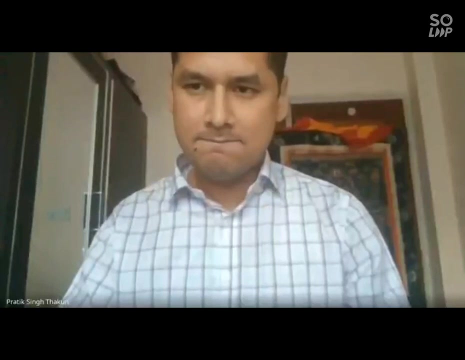 single data. I think in India and Sri Lanka and other countries they have metrological department and the hydrological data are taken care by other governmental institutions, But in Nepal it's a department of hydrology and metrology. They're integrated. Yeah, So I'll now go to my presentation. Is it visible? now my screen. 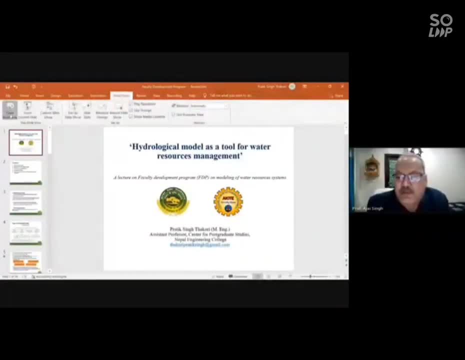 Yes, yes, You, you are clearly audible and your screen is visible. Now you can go to slideshow. Yeah, Yeah, thank you. So the topic given to me, or I've chosen the topic, was hydrological model as a tool for water resources management. So for this lecture on faculty development program on modeling of water resources system, and it's a great honor and I take it as a privilege, and thank Professor Ajay. 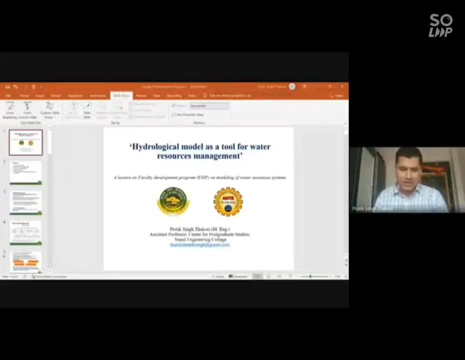 Thank you, Professor. Thank you, Professor Ajay, for giving me this chance to deliver a lecture in his esteemed institution. So my name is Pratik Singh Dhakuri and I have a master in engineering and water resources engineering from UNESCO Madanjit Singh Center for South Asia Water Management University of Morotoa, Sri Lanka, And I have completed my bachelor in technology from Kathmandu University. as an environmental engineer, I'm currently associated with Nepal's 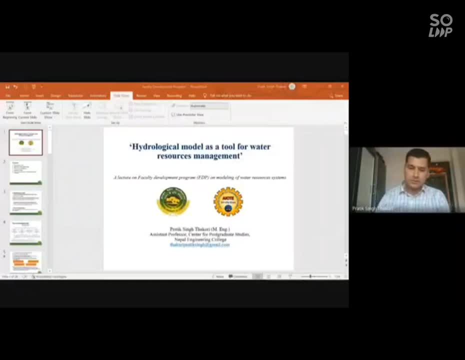 Engineering College Center for Postgraduate Studies as assistant professor. So today I'll be, you know, touching a few topics regarding hydrological models and how it should be selected and what are, you know, the important things to be considered while selecting models, you know, and then other things to be considered for a holistic and comprehensive hydrological modeling. What are the things to be considered? Yeah, I'll be touching all these topics. 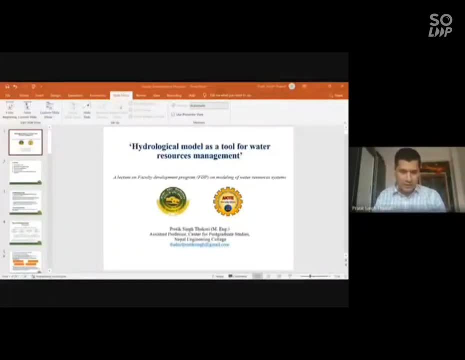 Not so much in detail, but, yeah, I'll give a quick overview and share some of the literatures I have found interesting, and I'll be sharing the references as well. Yeah, so I'll be talking about hydrological model and how hydrological models should be selected and what are the criteria for model selection. What are the objective function, What is the importance of objective function in hydrological modeling? And the fifth thing I've included here is the flow duration curve for models. 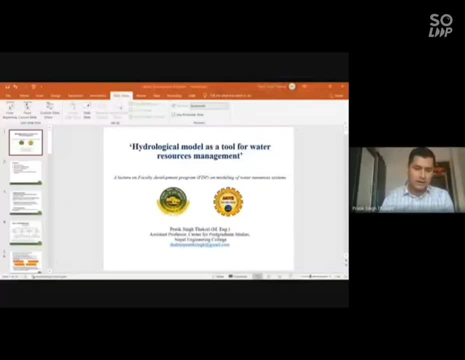 Calibration and validation, Why it is important. I'll be talking about that as well And, if you have time, I'll briefly share my spreadsheet of flow duration curve and how it can be utilized for model calibration and validation. Yeah, So yeah, I think Professor Ajay has touched all this topic in his initial presentation. I was also listening as a participant in that presentation. 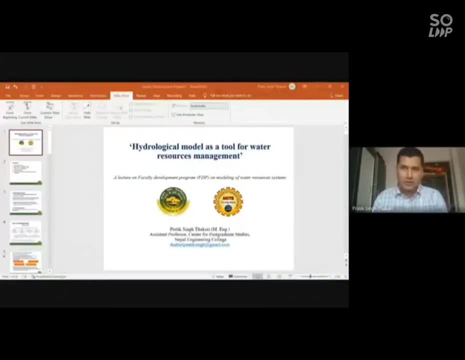 So you have touched on basically all these hydrological model theoretical concepts and you know the principles and everything, So I'll not dwell more in these areas. Yeah, but let me briefly summarize what is hydrological model and how hydrological model, what are their types and everything. 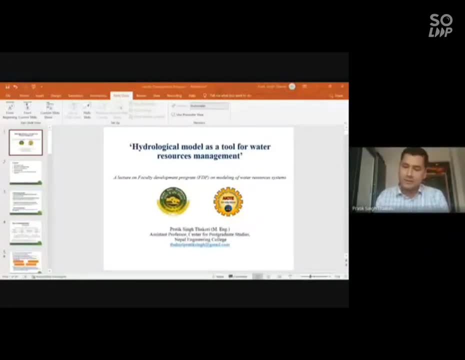 So hydrological model, or model itself, is a simplified representation of real world. It's a simplified representation of the real world. So no model is, you know, perfect. It is not that there are these. When one want a traditional three dimensional model, you can build a God concept in itself, It's just a representation of the real world. And what is hydrological model? 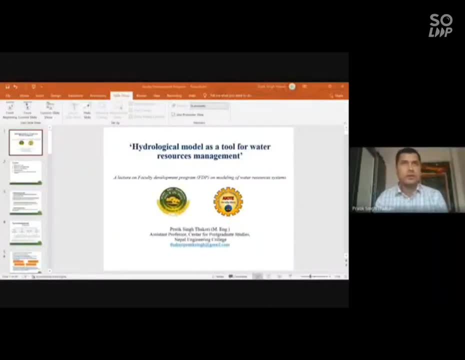 So hydrological model describes nonlinear and dynamic transformation of precipitation or indicators To run off through the process of, such as surface and surface flow in infiltration, interception, evaporation, transpiration, small melt and so on. So a hydrological model. they also say another: 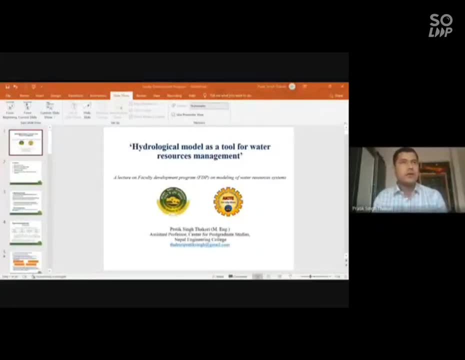 So hydrological model: ofducídate Highlychantable, Highlychmetic around the rainfall, runoff model. so how, how the the precipitation- either it is in the form of rainfall or a snow melt or something, so how it is converted to a runoff, and that there includes a. 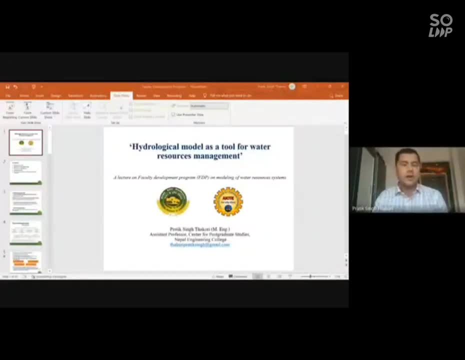 lot of other other processes, ideological processes in either, it be overland flow or surface flow, or infiltration, evaporation, transportation, snow melt and etc. so including all these processes and converting precipitation to run, runoff is mainly what a hydrological model does. so it comprises of a set of equation to estimate runoff, and those um equations are the function of 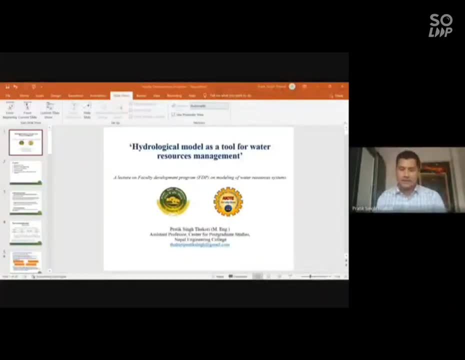 various parameters used to express the watershed characteristics, such as geography, geology, land use. so the, the equation of hydrological models are basically the function of the multiple parameters of describing the watershed characteristics: the geological condition, a geographical condition, their slope, their land use, their soil type or the. 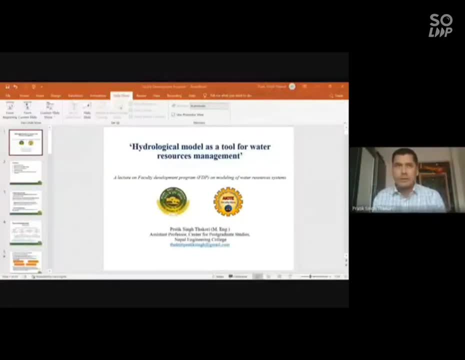 infiltration capacity, um, due to their uh, the peculiar soil type or anything, the, the specification or speciality of the watershed, uh are, you know, exhibited in the the function and those parameters. as a function of those parameters, those equations and those set of equations as a whole, uh works as a 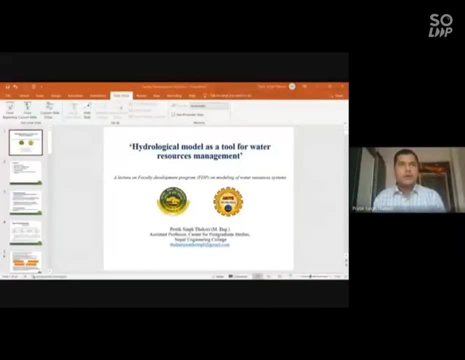 hydrological model. so so there comes a question. there are a lot of hydrological model existing in uh till date, but what is the? uh? you know, the best hydrological model. so the best hydrological model? uh, as per the definition? uh, there's nothing such called a best hydrological model, but the 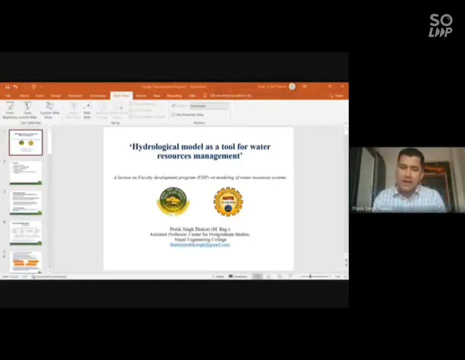 model which gives a result close to reality and use list parameter and model complexity is the best hydrological model. so there are types of hydrological model. i think professor has already touched this area, but i'll briefly go into it as well, because it will be- it will be- a warm-up session in the beginning, before 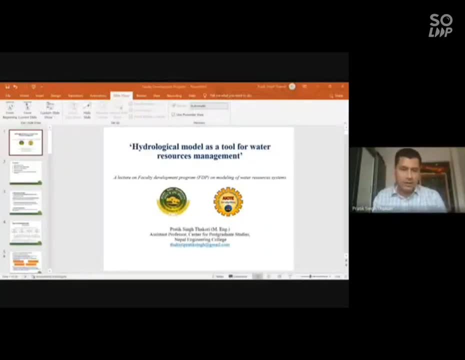 entering into the depth. yeah, so hydrological model can be classified into numerous, a number of types, but uh, i have, i have listed here a four type of hydrological model, based on representation, process representation, spatial representation, time representation and the aspect of randomness. so, on the basis of um process, it can be physical. 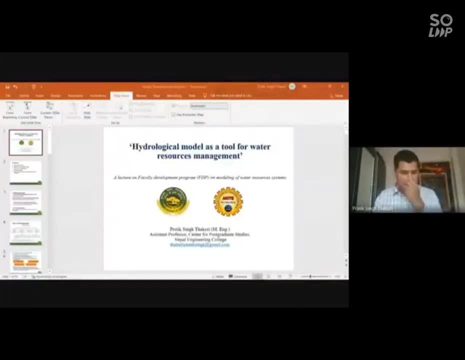 empirical or the conceptual. so i think, um, uh, i do not uh go into the definition of all these types of uh models. yeah, um, so, based on uh spatial representation, it can be semi-distributed, lumped or distributed, and based on uh time representation, it can be static or dynamic, and best, 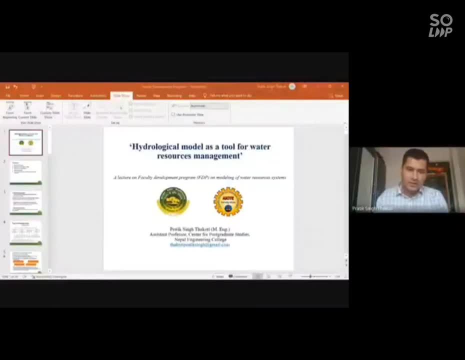 expected randomness. it can be stochastic and deterministic. so, yeah, there are different types of hydrological model and they can be classified into number of types, uh. so the question um arises here: what is the best high logical model for uh for for implementing in your watershed or your river? 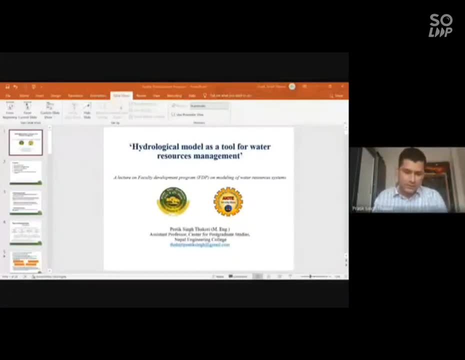 basin what would be the best hydrological model. so there are a lot of types of hydrological models there. they can be classified into numerous type, but when we use a hydrological model which would be the best one use, so it's just like um, you know, it's not just like a video game gimmick. you could choose there. 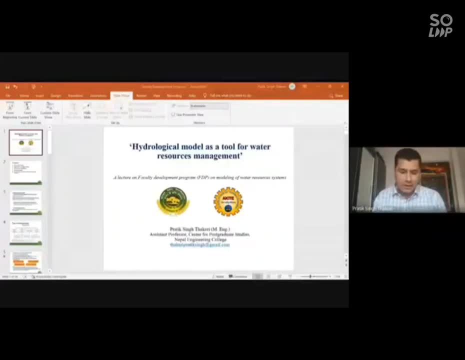 are a lot of speciality and specs and you uh choose the speciality from all this. but you have to. i mean in a scientific research or in an engineering process. your selection process should be rational or you should have a specific description or your justification why the model. 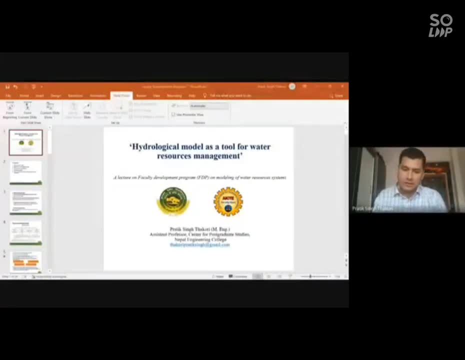 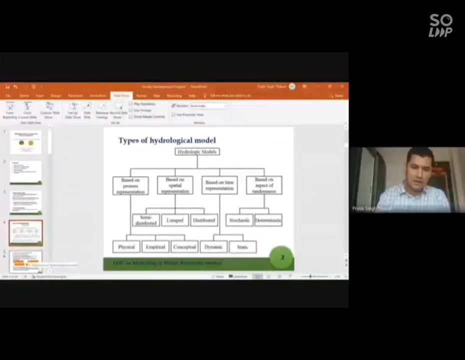 is, was selected for, uh, your study, your research. so i'll be talking about you. know how to rationalize the selection of model for um, for your research study? hello sir. yeah, sorry to disturb you, sir, your slide is not moving, just fast slide. is it just a flash? fast light? yes, sir, is it now visible? yes, it's now visible. yes, 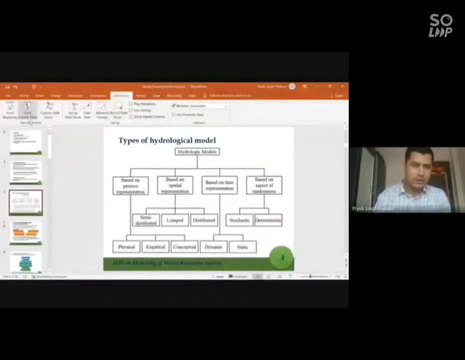 okay, so this? so in the okay, is it not visible? the types of biological model? i'm showing it in this screen? yes, sir, okay, yeah, the selection of hydrological model- yeah, i was talking about it- should be rational and justifications should be done. so, uh, it's not a process of the train that, if someone else has. 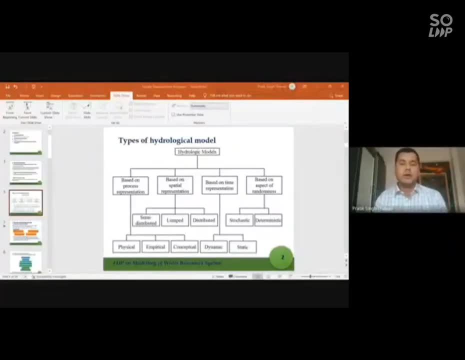 used the hydrologic model, that would be a best hydrological model for uh, your watershed, or for for for a researcher to conduct a research study. there are a lot of factors to be considered, a lot of criteria to be, you know, taken under consideration for ideological model selection. so 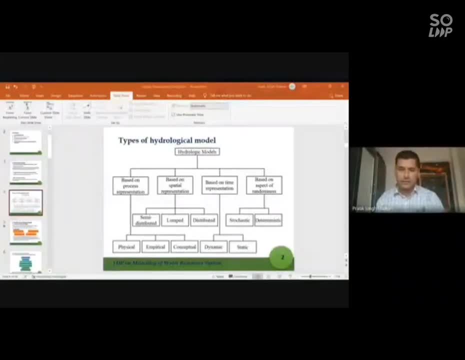 it's a crucial and subjective process- it's not a very objective but it's quite crucial and subjective process- of selection of ideological model and, and as i have already you know, told that no model can be identified as an ideal for all range of ideological condition. and 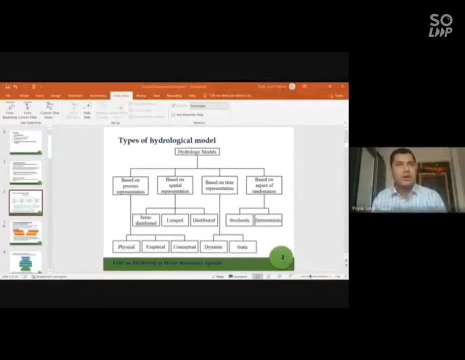 watershed characteristics. so so if, if a hydrological model was, you know, performing really good in the, in the tropical condition, it may not be very good for an arid condition, or it may not be very, you know, it may be completely absolute when it is trying to be used in the. 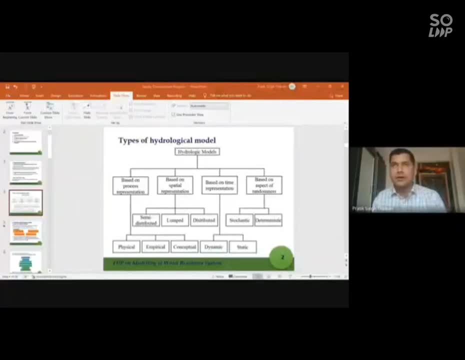 in the higher himalayan river basin, where the snow melt contribution in the watershed is predominant. yeah, so, so far, there is no, you know, model that can be identified, ideal for all hydrological condition, and what is it? characteristics so, so? so, while selecting hydrological model, it should not be, you know, supposed to be solely. 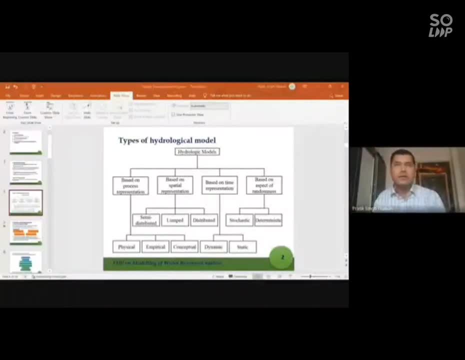 reliant on predictive uh performance. if, if, the, if you get a hydrological model which gives you you know uh best um performance in terms of your, your uh hydrograph simulation and the hydrograph matching and all these objective function and you know efficiency criteria, it is showing 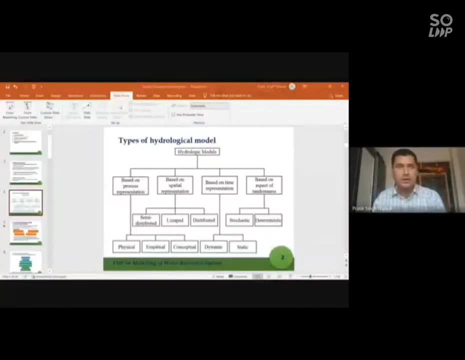 very good, but that is not, uh, what you should be should be solely reliant on. there are a lot of other factors that should be uh considered. so the first thing would be the model preferences, modeler preferences or familiarity to toward the model, so that should be also be considered as one. 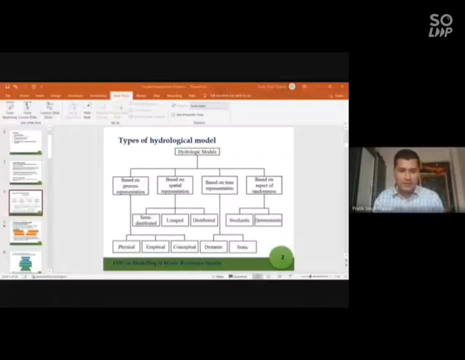 of the criteria for selecting the model. if the model modeler is not very familiar to that hydrological model, uh you know output uh of the model, even if it is really you know performing uh good in other watershed or other study, it may not give the result uh good in in that case, yeah. so another thing is the aim of 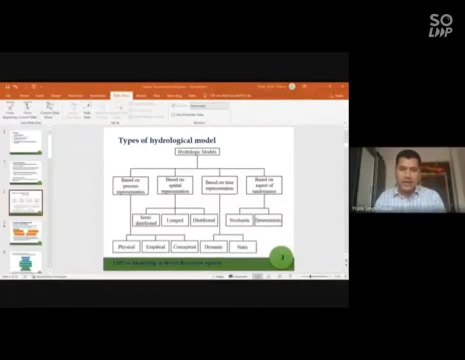 modeling task. uh, third thing is time, time and, above the time, ability to develop and apply the model. and the fourth is the level of accuracy needed. so, aim of the modeling task. so if the model is aimed for, you know, uh, you know, for agricultural, uh, water management, or the water resources management, or the drought, 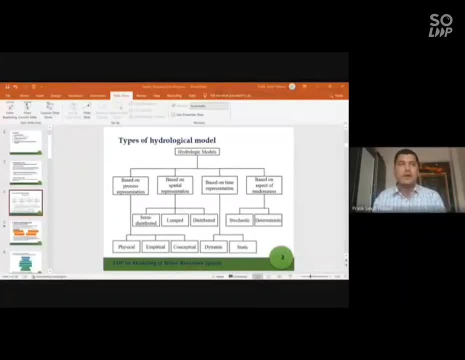 management cases. you know, in some some very uh, the area where the river has mostly low flows conditions, or it's a as a seasonal river or something like that. so, um, then the aim of modeling would be different than if, uh, then the like a flood management or disaster management in. 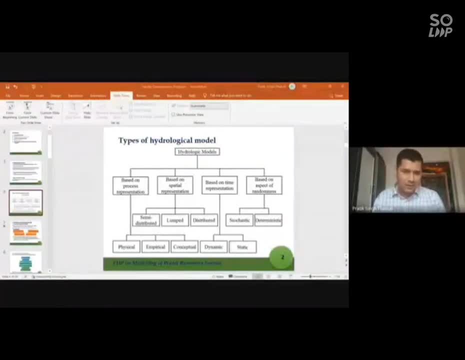 the case. similarly, uh, what is the time available for modeler to, you know, develop the model and apply the model? that would uh be also a very crucial thing to be considered. you know, if you have, uh, if you are going through a rapid, you know- assessment of a watershed, you need a there has. 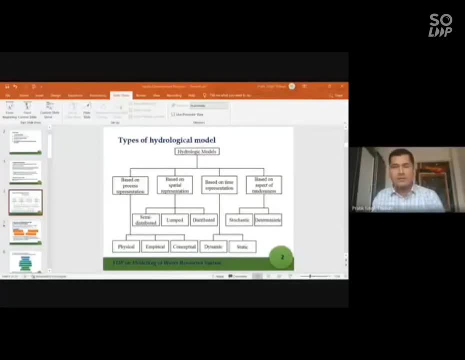 been a flood and you, you, you are given an assignment to assess the condition of the watershed and everything with the hydrological model. you are not going to perform a good job of modeling, which takes a really big time and effort, and you know, uh, such kind of thing you. 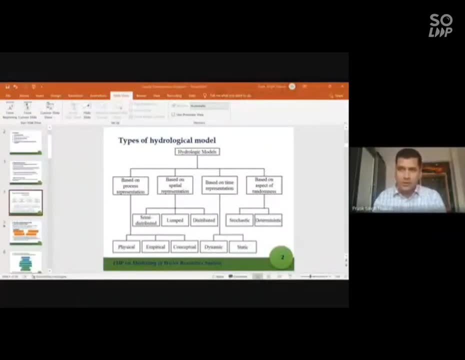 you'll go. you'd rather go for a model whiskey of you know, a quick outlook of the watershed or some picture of the watershed. you can depict some picture of watershed and you can get some ideas from the model. that would be fine. so the third thing is: 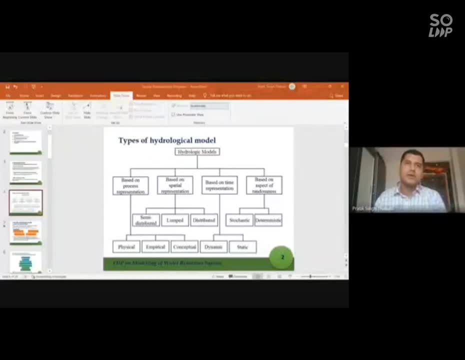 the level of accuracy needed. like i have said, like in some research you really need, you really try for result in the your study. but in some studies, just like I have mentioned before, in the rapidest case study or or anything like you know you're performing, so you may not need on the higher and accuracy of the model. so in that cases 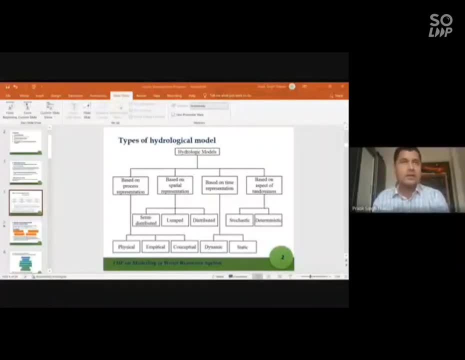 you know, the preferences of the selection of model can be different. so the basis of the selection of model, as I have already told, maybe you know, different as per many criteria. so I have listed some basis of selection of model like purpose of this study: nature of the watershed if it is a ruler watershed of. 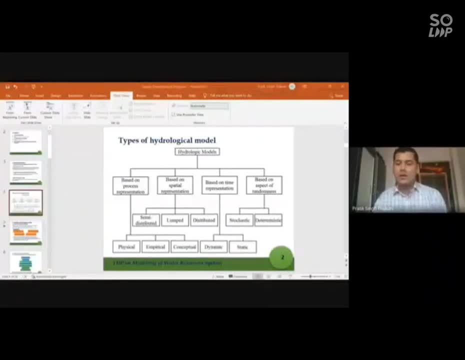 the urban watershed, the selection of model would be different. what is the data available in your watershed? if there is very less data available and you are trying to use a model like short or something like other model that requires heavy amount of data, then the model would be. 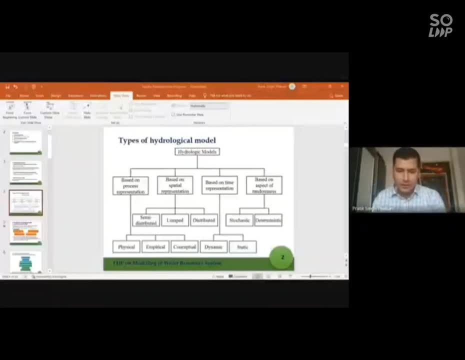 considered as an inappropriate and something and another, basically adequate knowledge on model parameters. you know, if the model model developer claims it, his model is the very good performing model, but the parameters and are not, you know, already estimated in other watershed, validated on other watershed. in such cases you know the modeler. 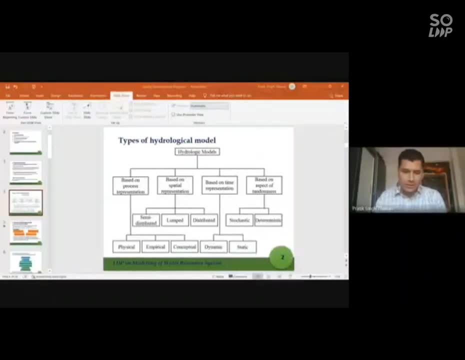 initiator will face a lot of difficulty on in estimating parameters and everything. and it will be a huge, huge task for our modeler, to you know, starting from scratch. and since another thing is the knowledge of model processes and estate, you know the modeler should have a depth, in depth, knowledge of the 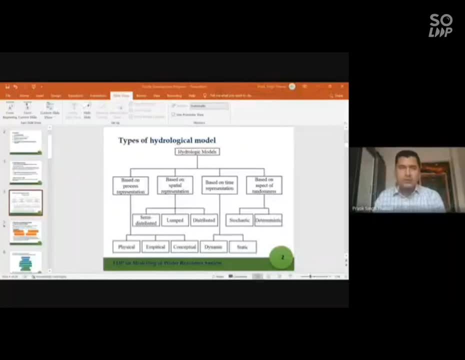 processes and estate, although else the model developers would have, you know, given the appropriate reference manual, user manual of the model. otherwise the model itself would be more complex and all the models have in line equations and underlying theories and hypothesis and assumptions. so that should be, you know, considered, that should be. that would be a very important criteria to 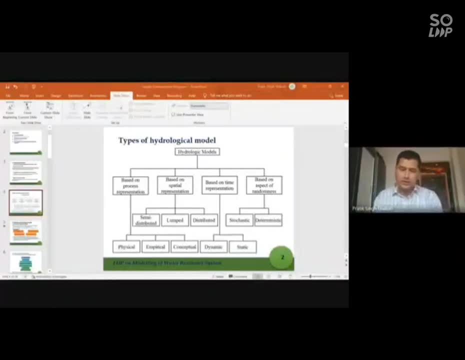 select the model. and the third thing is the complexity of model and lastly, the cost and availability of models. so all the models are not in the public domain, in a free to use. there's models which are exclusive and there are some models which are, you know. 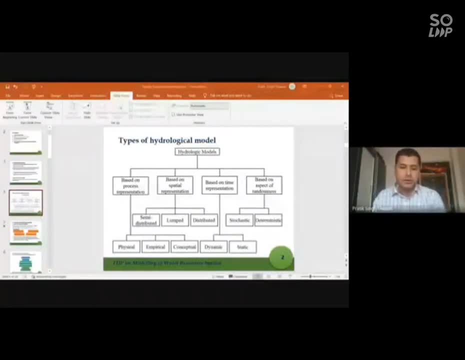 uh, you need to pay for it, so. so if, if you're, if you are in the limited fund or if you don't have any, any budget for to for your study in purchasing the hydrological model, so you'd rather go for the free domain model, the models available in freedom and whatever, if it's a. 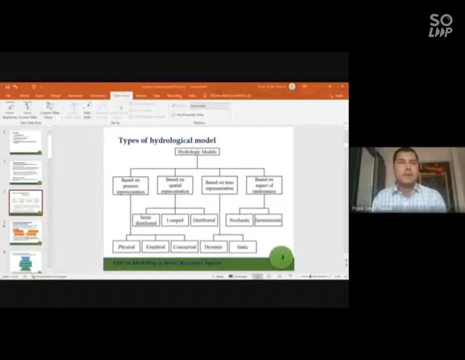 drawbacks. you would rather choose the um, the model available in the free domain. so there are a lot of factors that should be considered while selecting the model. so, yeah, so i have talked in a broader spectrum of selection, selection model, but now i'll be, you know, pointing out it in the bullet form. 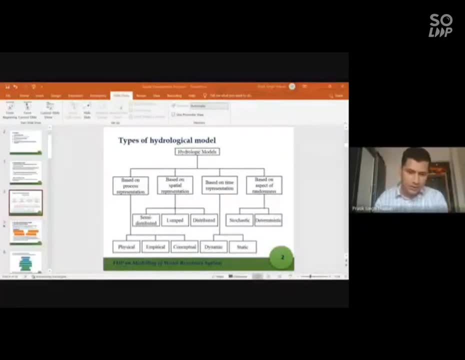 so criteria for selecting hydrological model, yeah, it is not limited to these seven criteria, but uh, you can, you can suggest me, or you can, you can, when you are doing your study on your own, you can add other other criteria for selecting models and other evaluation. uh, you know the framework. you can develop it on your own, but i'm just sharing my 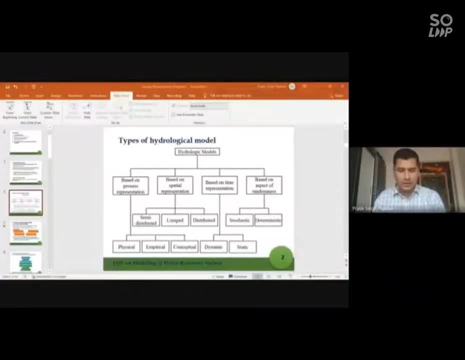 criteria um on selecting the high classical model, and i have also published a paper on selecting hydrological model on journal of water engineering management, where professor aza is a chief editor. so i'll give the reference of my paper as well in this presentation. so there are. 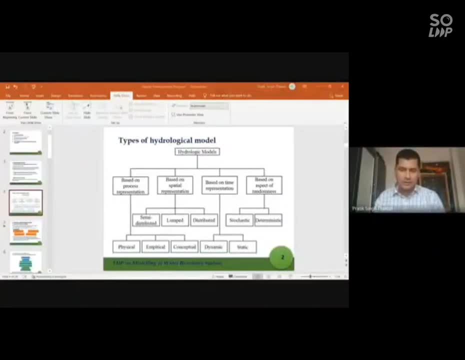 you know i have listed seven points, uh, seven criteria for selecting hydrology model. so criteria number one is temporal scales, the criteria number two spatial scale, three hydrological processes, four: documentation, support, resource requirement, user interface and model acquisition cost. there could be other other criteria as well, but for my study 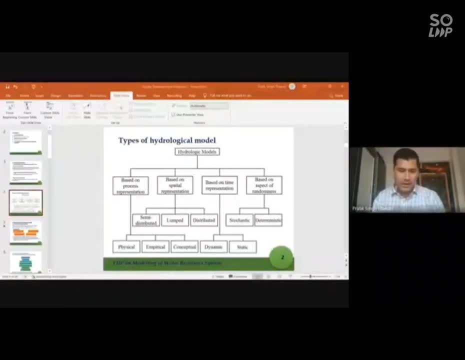 I have considered these seven criteria. you know, for me model acquisition cost if it is, you know, exclusive and if you have to pay for it, the even the model is performing really good in all this criteria that the model which have, which is exclusive, would get obsolete and get zero value in my criteria evaluation. 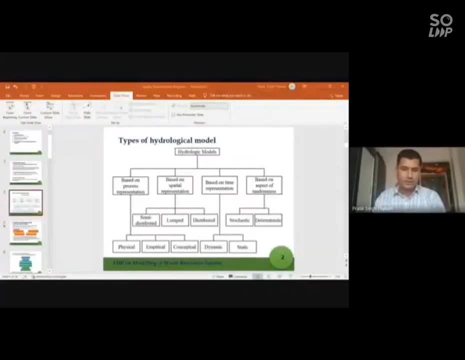 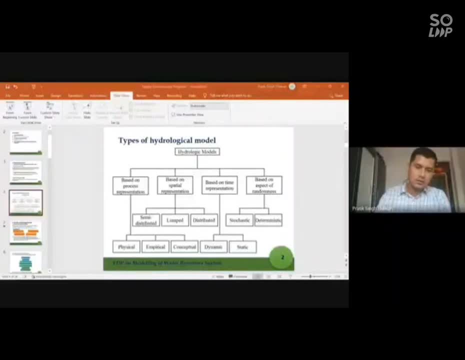 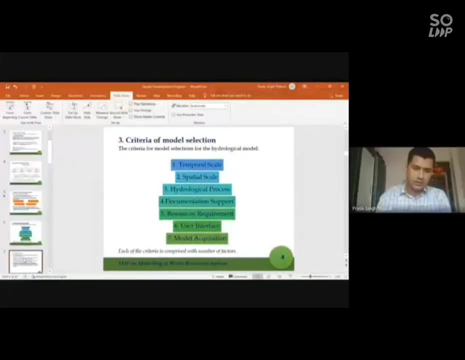 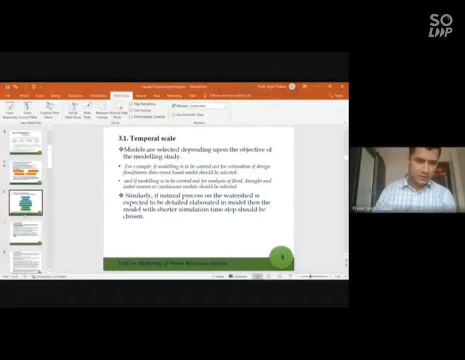 so i'll, i'll be sharing here in, so i'll. i'll be sharing here in, so i'll, i'll. i'll be sharing here in the normal mode rather than presentation. the normal mode rather than presentation. the normal mode rather than presentation mode. i think the presentation mode. 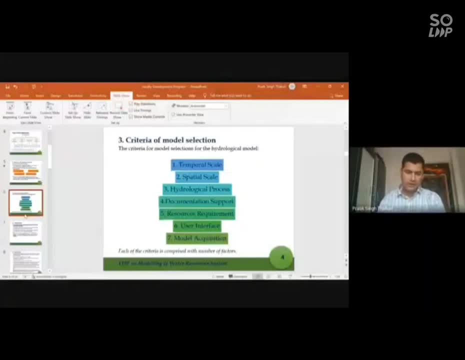 mode. i think the presentation mode mode, i think the presentation mode, slide share mode is having some problem. slide share mode is having some problem. slide share mode is having some problem in my computer. i don't know in my computer, i don't know in my computer, i don't know. so yeah, so for for someone, um, who have 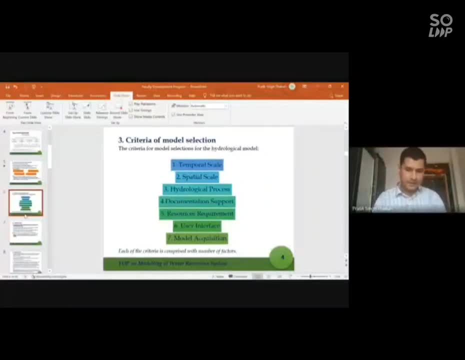 so yeah, so for for someone, um who have. so yeah, so for for someone, um who have very, very, very less data, or less data, or less data, or working in the watershed with the with working in the watershed with the with working in the watershed with the with the data scarcity or data scary. 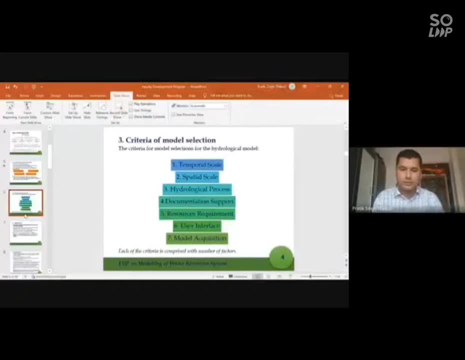 the data scarcity or data scary, the data scarcity or data scary environment? uh for for them. the data environment, uh for for them. the data environment. uh for for them. the data requirement and other things would be a requirement, and other things would be a requirement and other things would be a special criteria for model selection. so 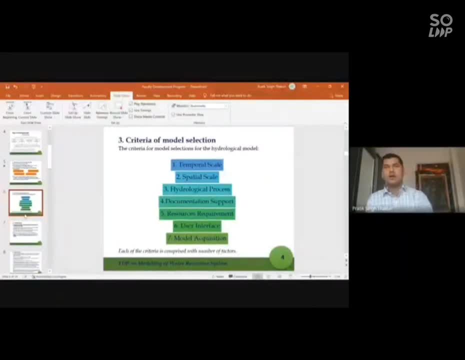 special criteria for model selection, so special criteria for model selection. so likewise you can, you can, you can list: likewise, you can, you can, you can list: likewise, you can, you can, you can list out your criteria for model selection as out your criteria for model selection, as out your criteria for model selection as well. 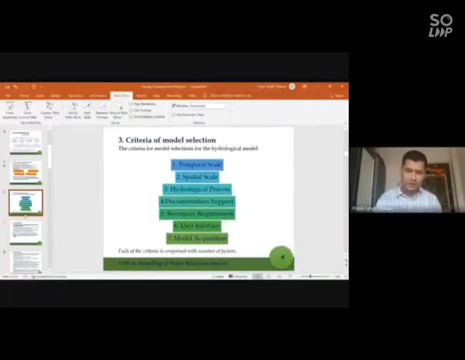 well, well, but yeah, i'll be talking about these, but yeah, i'll be talking about these, but yeah, i'll be talking about these. seven uh model. seven uh model. seven uh model model selection criteria, um and would be model selection criteria um and would be model selection criteria um and would be, would expect, uh, you all. 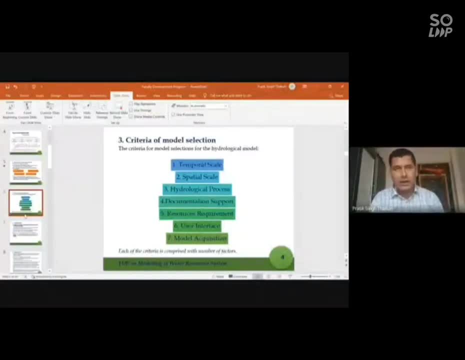 would expect, uh, you all would expect, uh, you all to give you know, to give you know, to give you know feedback. what else uh could be the feedback? what else uh could be the feedback? what else uh could be the criteria for some model selection, criteria for some model selection. 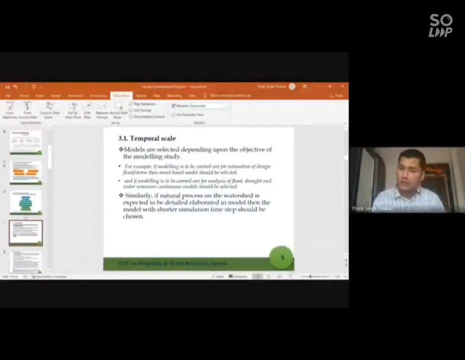 criteria for some model selection. so temporal scale, so temporal scale, so temporal scale, uh so model are selected depending on the uh so model. are selected depending on the uh so model. are selected depending on the objective of model study, objective of model study, objective of model study. so, for example, if you have, if you have, 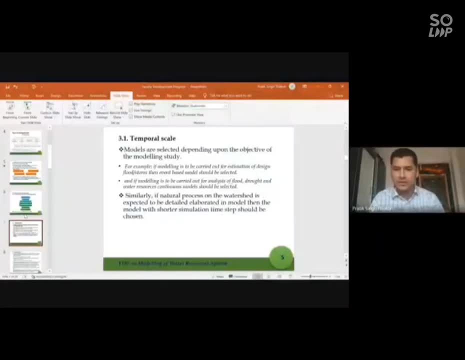 so, for example, if you have, if you have. so, for example, if you have, if you have, this model is uh to be carried out, for this model is uh to be carried out, for this model is uh to be carried out for the estimation of ideological flood: you. 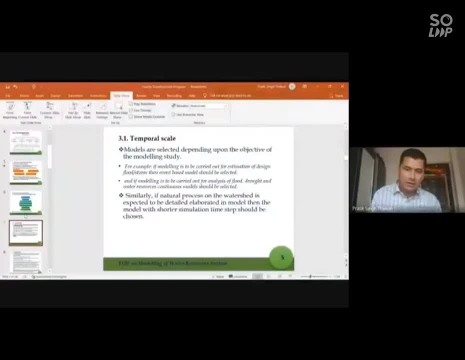 the estimation of ideological flood. you the estimation of ideological flood. you know the design estimation of the design. know the design estimation of the design. know the design estimation of the design. flood or storm, then event bus model. flood or storm, then event bus model. flood or storm, then event bus model would be. 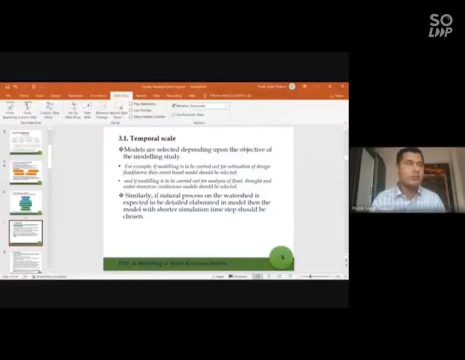 would be, would be, you know suitable to select it, if you, you know suitable to select it, if you, you know suitable to select it, if you just want, just want, just want to design a culvert, uh and uh, you know to design a culvert, uh and uh, you know. 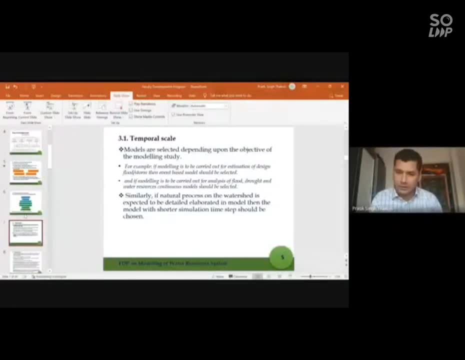 to design a culvert, uh and uh, you know, or, or, or, a strong event. so the event bus model, a strong event. so the event bus model, a strong event. so the event bus model would be suitable to, would be suitable to, would be suitable to, um, for those purpose, but if you, if you. 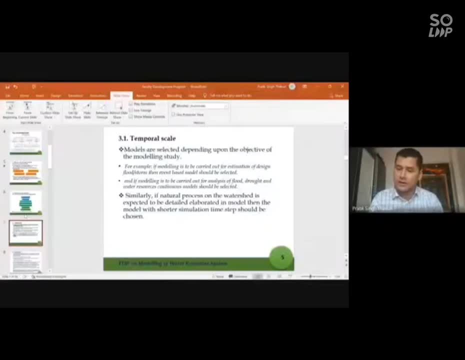 um for those purpose. but if you, if you um for those purpose, but if you, if you want, want, want a modeling to be carried out for the, a modeling to be carried out for the analysis of flood, analysis of flood, analysis of flood, you know drought or water resources, then 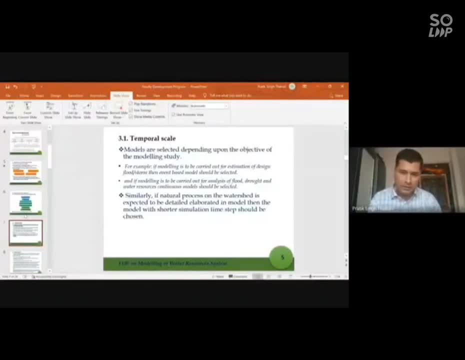 you know drought or water resources, then you know drought or water resources, then the continuous model, the continuous model, the continuous model, should be selected. so based on this, should be selected. so based on this, should be selected. so based on this: temporal scale, the event best, or temporal scale, the event best, or. 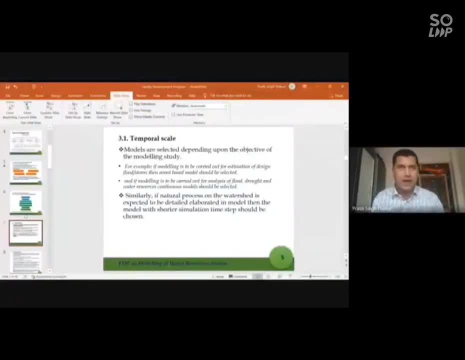 temporal scale. the event best or continuous, the. the rational of selection should be the. the rational of selection should be the. the rational of selection should be clear and the purpose clear and the purpose clear and the purpose of the study should be clear. similarly, if, if the natural process of 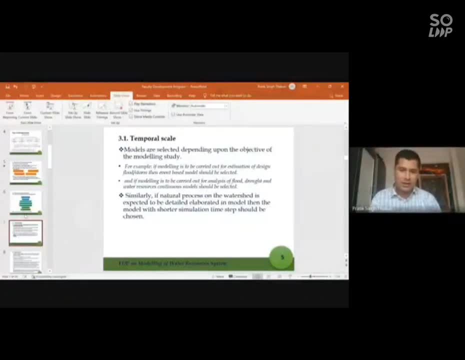 similarly, if, if the natural process of similarly, if, if the natural process of the watershed is expected to be, the watershed is expected to be the watershed is expected to be detailed, elaborated in the model. detailed, elaborated in the model. detailed, elaborated in the model. then the model with shorter simulation. 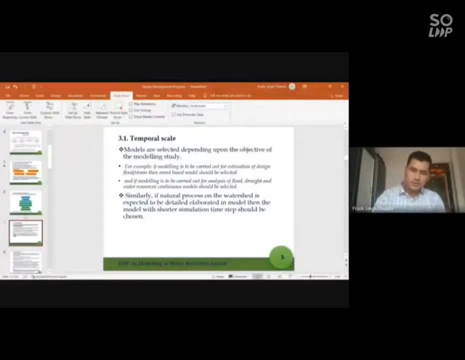 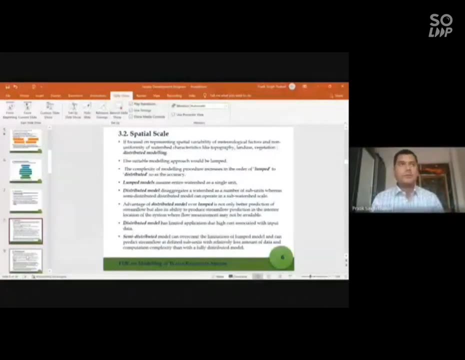 then the model with shorter simulation, then the model with shorter simulation time, step time, step time step should be chosen. secondly, the specialist skill um if um. secondly, the specialist skill um if um. secondly, the specialist skill um if um, if. uh, you know the model want to focus. 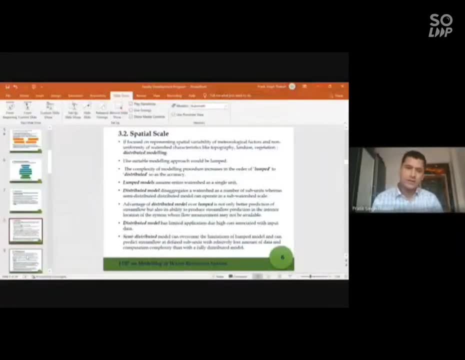 if uh you know the model want to focus. if uh you know the model want to focus on special uh variability of on special uh variability of on special uh variability of metallurgical factors- uh non-human metallurgical factors. uh non-human metallurgical factors- uh non-human uniformity of. 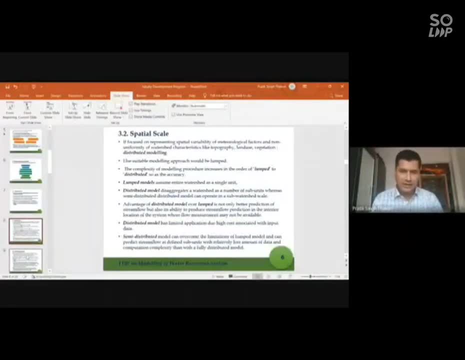 uniformity, of uniformity of the watershed characteristics or the the watershed characteristics or the the watershed characteristics, or the heterogeneity of the water sector. heterogeneity of the water sector. heterogeneity of the water sector characteristic like topography land use. characteristic like topography land use. 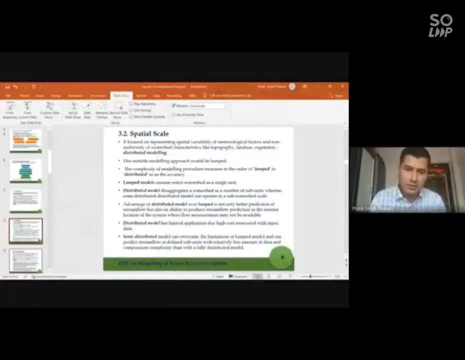 characteristic, like topography, land use, vegetation. you know uh in detail, then vegetation. you know uh in detail, then vegetation. you know uh in detail then distribution, uh distributed modeling. distribution, uh distributed modeling. distribution, uh distributed modeling is suitable. one is suitable. one is suitable. one um else the suitable modeling approach. 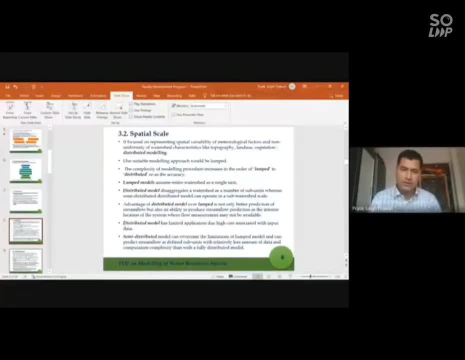 um else the suitable modeling approach, um else the suitable modeling approach would be lumped. but if you really want, would be lumped. but if you really want, would be lumped. but if you really want to, you know, represent the special, to, you know, represent the special. 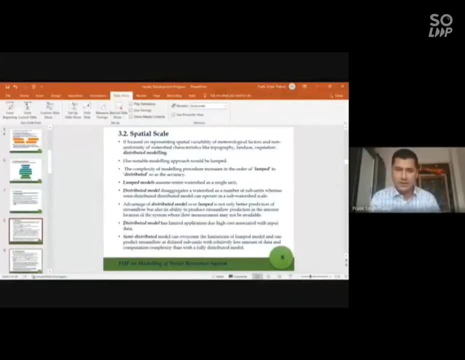 to. you know represent the special variability of the um. you know variability of the um. you know variability of the um. you know metallurgical factors and the metallurgical factors and the metallurgical factors and the heterogeneity of uh, heterogeneity of uh, heterogeneity of uh, the watershed conditions and everything. 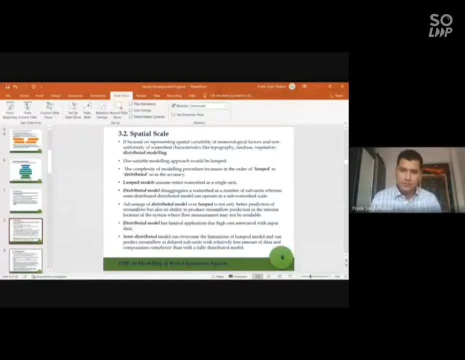 the watershed conditions and everything, the watershed conditions and everything. then then, then the distributed model would be suitable, the distributed model would be suitable, the distributed model would be suitable, but you know the complexity of the model, but you know the complexity of the model, but you know the complexity of the model processor. and 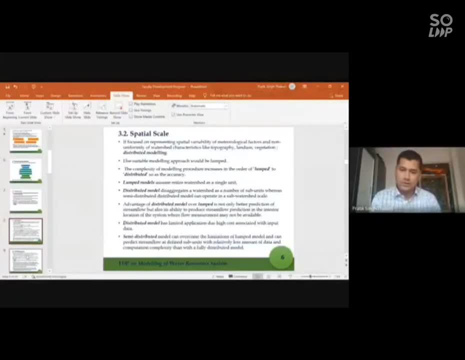 processor and processor and, uh, you know the the data requirement, uh, you know the the data requirement, uh, you know the the data requirement, and everything and everything and everything would thoroughly, you know increase, if you would thoroughly you know increase, if you would thoroughly you know increase if you go from lump to distributed, you know the. 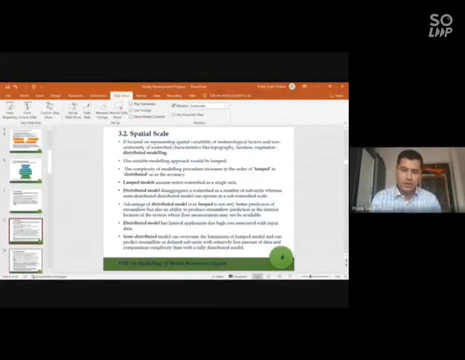 go from lump to distributed. you know the go from lump to distributed. you know the distributed model. distributed model, distributed model, is less complex compared to what uh is, less complex compared to what uh is less complex compared to what uh. you know the dump model is. you know the dump model is. 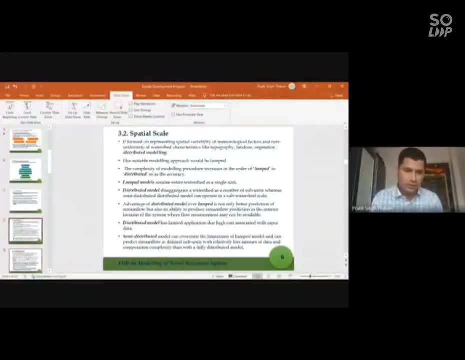 you know, the dump model is very less, you know, complex compared to distributed one. so the complexity of model distributed one, so the complexity of model distributed one, so the complexity of model, um, um, um, you know, is another factor in the in the. you know, is another factor in the in the. 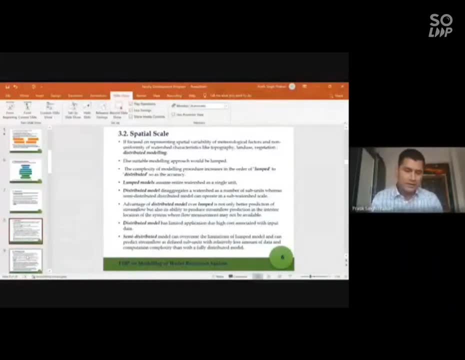 you know, is another factor in the, in the selection of model, selection of model, selection of model. so, so, what is the complexity you would so, so, what is the complexity you would so, so, what is the complexity you would like to deal with, like to deal with, like to deal with what? um, what is the level of data you? 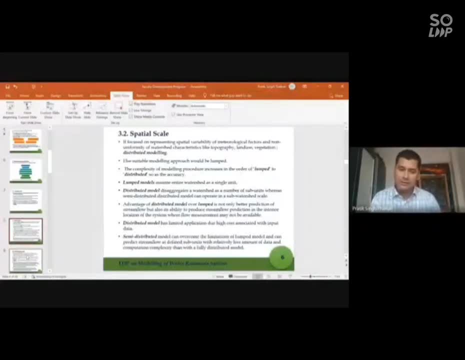 what um? what is the level of data? you, what um? what is the level of data you have available? have available? have available, um, that would be another factor. so if um, that would be another factor. so if um, that would be another factor. so if you have very less amount of data or you. 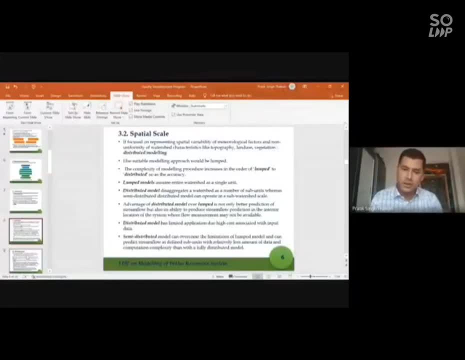 you have very less amount of data, or you you have very less amount of data, or you have very uh. you know less amount of have very uh, you know less amount of have very uh, you know less amount of time and knowledge to deal with time and knowledge to deal with. 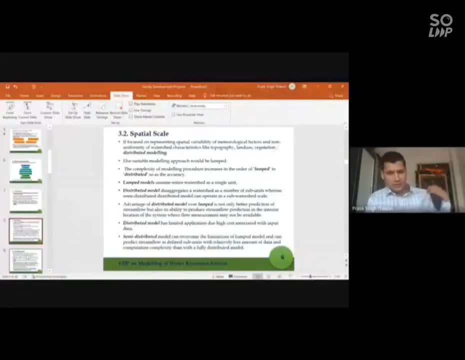 time and knowledge to deal with uh in the hydrological modeling, then uh in the hydrological modeling, then uh in the hydrological modeling, then it is not advisable to go to the, it is not advisable to go to the, it is not advisable to go to the distributed modeling. it is really uh it. 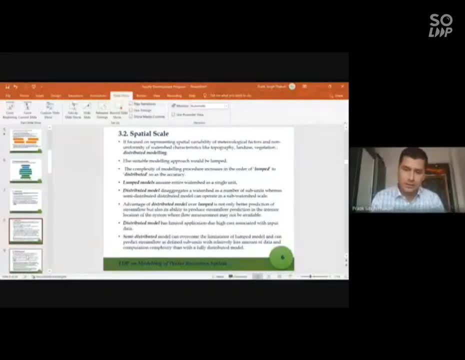 distributed modeling. it is really uh, it. distributed modeling, it is really uh, it demands higher amount of data and uh, you demands higher amount of data and uh, you demands higher amount of data. and uh, you know, know, know use time. you know even even your use time. you know even even your. 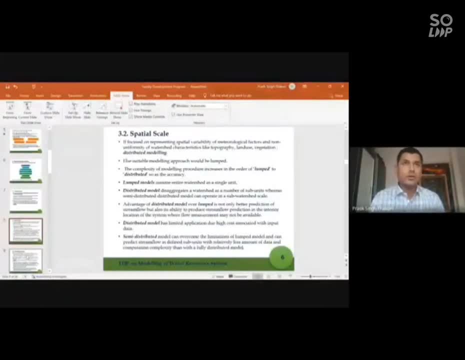 use time. you know, even even your computer model, computer, computer model, computer, computer model, computer specification requirement would go high, specification requirement would go high, specification requirement would go high. so similarly, so, similarly, so, similarly. you know, the lump model is just uh you. you know, the lump model is just uh you. 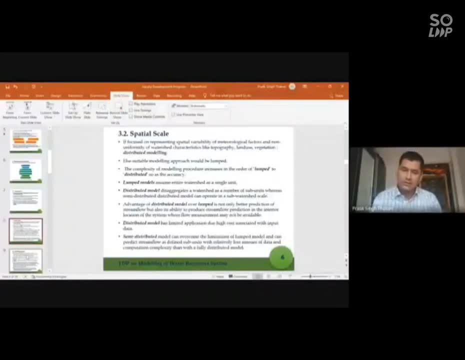 you know, the lump model is just, uh, you know, know, know. assumes whole watershed as a single unit. assumes whole watershed as a single unit. assumes whole watershed as a single unit, whereas a distributed model, whereas a distributed model, whereas a distributed model, disaggregates a watershed into a number. 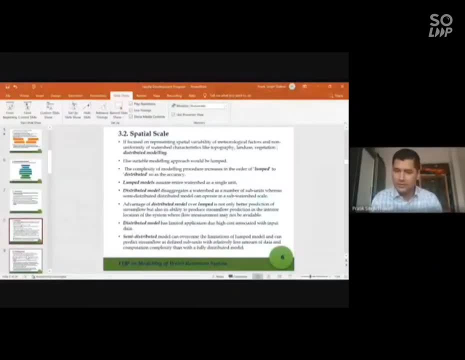 disaggregates a watershed into a number. disaggregates a watershed into a number of sub units. where of sub units? where of sub units? where semi-distributed models can operate in? semi-distributed models can operate in. semi-distributed models can operate in this. this. 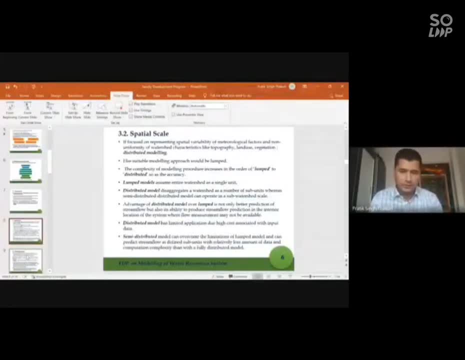 this sub water status scale. so there is a sub water status scale. so there is a sub water status scale. so there is a third model, um third model, um third model, um type that is called semi-distributed or type that is called semi-distributed or type that is called semi-distributed or pseudo-distributed model. where it is it. 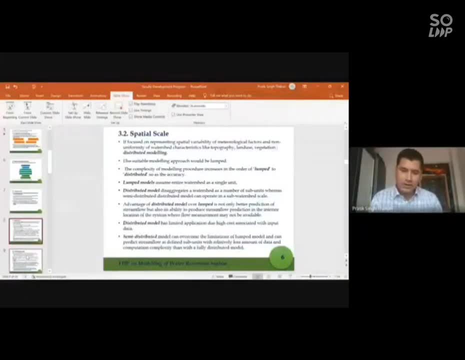 pseudo-distributed model where it is it pseudo-distributed model where it is. it is a compromise between: is a compromise between: is a compromise between: lumped and distributed model. uh in lump. lumped and distributed model: uh in lump. lumped and distributed model. uh in lump model it. 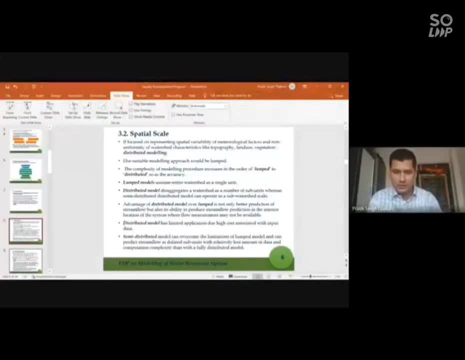 model it, model it. you know the, you know the, you know the model assumes whole water watershed as model. assumes whole water watershed as model. assumes whole water watershed as a single unit in a, whereas in the a single unit in a, whereas in the, a single unit in a, whereas in the distributed model. 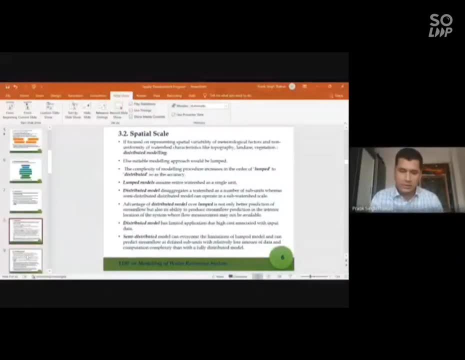 distributed model. distributed model: the model disaggregates watershed into the model. disaggregates watershed into the model. disaggregates watershed into numbers of sub units. whereas in the numbers of sub units. whereas in the numbers of sub units. whereas in the semi-distributed model model are: 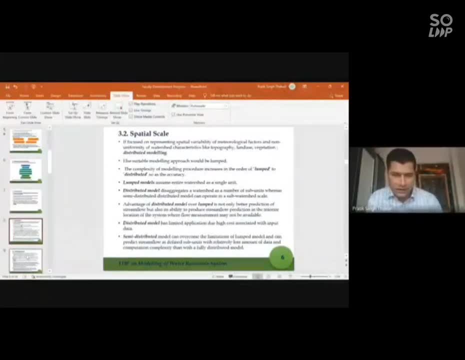 semi-distributed model model are semi-distributed model model. are disaggregated in the smaller sub water. disaggregated in the smaller sub water. disaggregated in the smaller sub water status scale. so the another avenue of status scale. so the another avenue of status scale, so the another avenue of the uh. 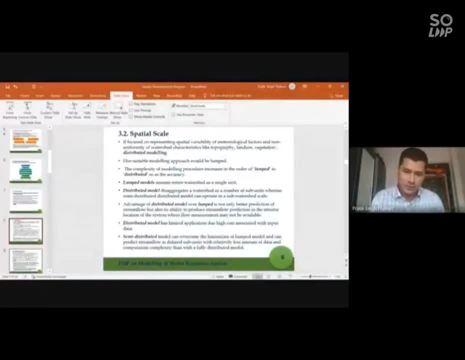 the uh, the uh watershed modeling or hydrological watershed modeling, or hydrological watershed modeling or hydrological modeling. uh was a semi-distributed modeling. uh was a semi-distributed modeling. uh was a semi-distributed model and which is uh model and which is uh model and which is uh getting quite. 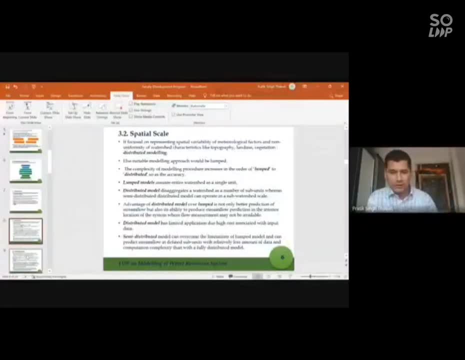 getting quite, getting quite popularity these days, yeah. so advantage of popularity these days? yeah so advantage of popularity these days, yeah. so advantage of distributed model. our lump model is not distributed model. our lump model is not distributed model. our lump model is not, uh, better prediction of streamflow, not. 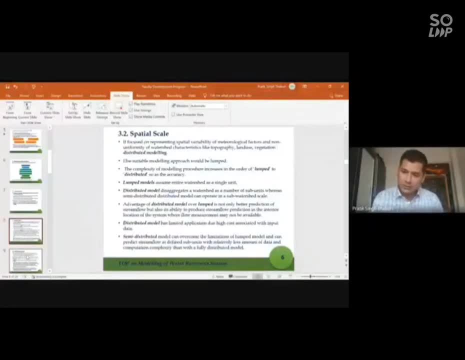 uh, better prediction of streamflow, not uh, better prediction of streamflow, not just a better prediction of streamflow, just a better prediction of streamflow, just a better prediction of streamflow, but also the ability to produce, but also the ability to produce, but also the ability to produce streamflow prediction in the interior. 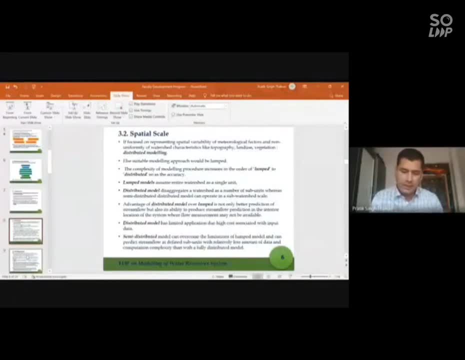 streamflow prediction in the interior streamflow prediction in the interior location of the system. where flow location of the system, where flow location of the system, where flow measurements are not available, so in the measurements are not available, so in the measurements are not available, so in the in the lump model uh, the 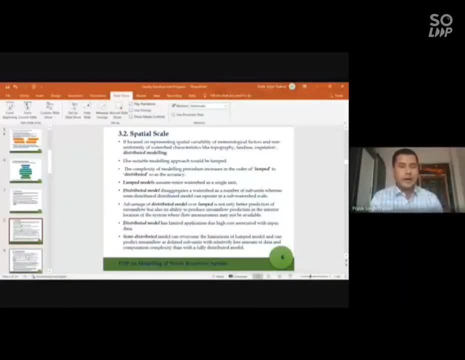 in the lump model uh, the. in the lump model uh, the streamflow are predicted at the outlet of streamflow. are predicted at the outlet of streamflow. are predicted at the outlet of the, the the hydrological um you know the watershed. hydrological um you know the watershed. 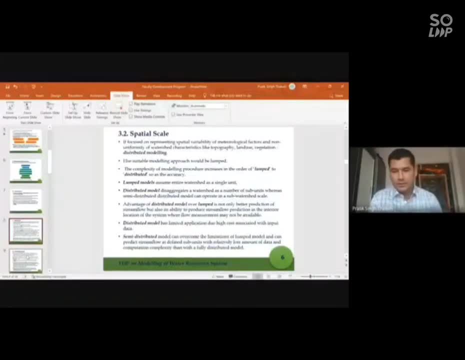 hydrological, um you know the watershed, but uh in the distributed model, um you. but uh in the distributed model, um you. but uh, in the distributed model, um you can predict the hydro, can predict the hydro, can predict the hydro graph. or you know the discharge graph, or you know the discharge. 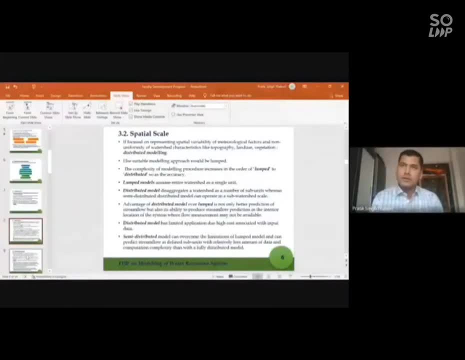 graph, or, you know, the discharge float in the float, in the float, in the in the interior of the watershed as well, in the interior of the watershed as well, in the interior of the watershed as well. so distributed model, as i've already. so distributed model, as i've already. 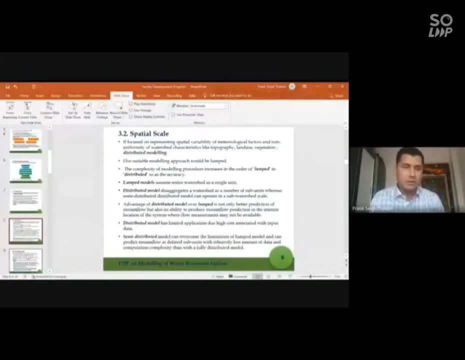 so distributed model, as i've already said that it is said that it is said that it is- has- has more advantage and a lot of drawbacks, or more advantage and a lot of drawbacks, or more advantage and a lot of drawbacks, or demerits as well, demerits as well. 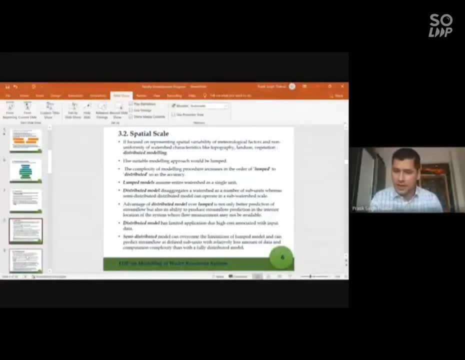 demerits as well that that that can be a limitation. uh due to the high can be a limitation. uh due to the high can be a limitation. uh due to the high cost. cost cost associated with its uh. the input data associated with its uh: the input data. 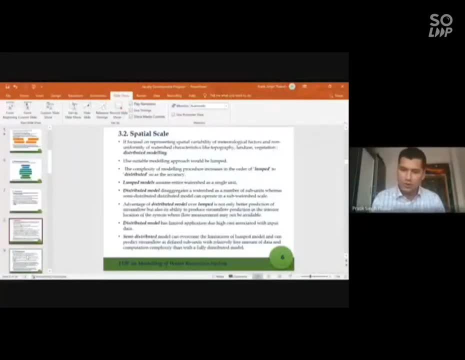 associated with its uh, the input data. similarly uh the semi-distributed model. similarly uh, the semi-distributed model. similarly uh, the semi-distributed model. you know, you know, you know that can overcome the limitation of the, that can overcome the limitation of the, that can overcome the limitation of the, both lump model and the distributed. 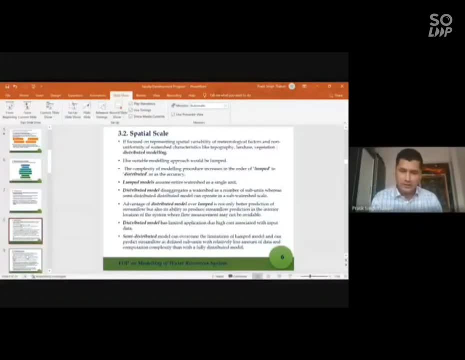 both lump model and the distributed, both lump model and the distributed model model model. uh, you know, uh, you know. and can predict the streamflow at the. and can predict the streamflow at the and can predict the streamflow at the defined sub watershed unit. defined sub watershed unit. 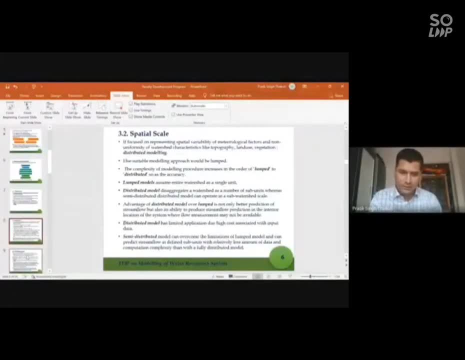 defined sub watershed unit and really with relatively very less, and really with relatively very less and really with relatively very less amount of data and computation, amount of data and computation, amount of data and computation. complexity um complexity, um complexity. um than fully distributed models, so so that, than fully distributed models, so so that. 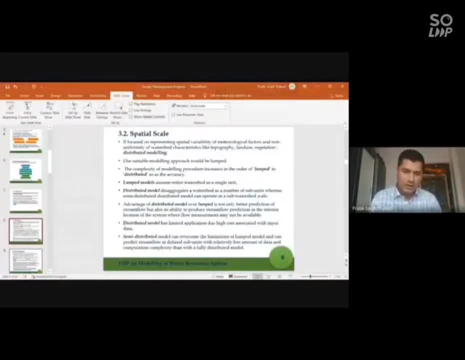 than fully distributed models. so so that there are drawbacks of the, there are drawbacks of the, there are drawbacks of the log model and there are advantages of log model and there are advantages of log model and there are advantages of the, the, the uh distributed model and both the 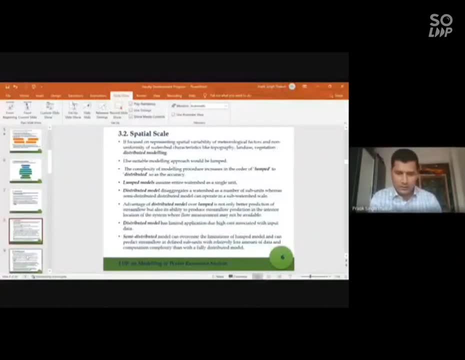 uh distributed model and both the uh distributed model and both the drawbacks of the distribution model as drawbacks of the distribution model, as drawbacks of the distribution model as well. so there is a compromise between well. so there is a compromise between well. so there is a compromise between lumped and distributed model. the. 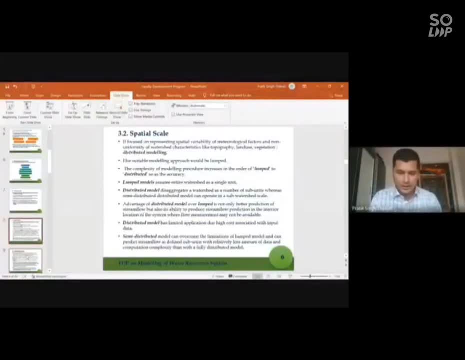 lumped and distributed model. the lumped and distributed model. the semi-distributed model. semi-distributed model. semi-distributed model. um, you know that, that uh, um, you know that, that uh, um, you know that, that uh. overcome the limitation of both um. overcome the limitation of both um. 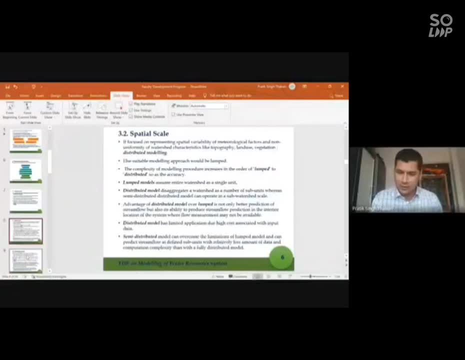 overcome the limitation of both um lumped and distributed model um and lumped and distributed model um and lumped and distributed model um, and can predict the streamflow at the. can predict the streamflow at the. can predict the streamflow at the sub watershed level. and. 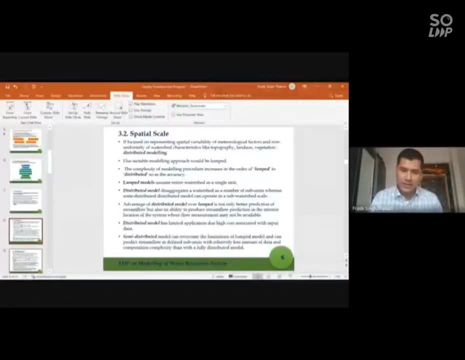 sub watershed level and sub watershed level and demands comparatively, comparatively. demands comparatively comparatively. demands comparatively comparatively: less amount of data compared to less amount of data compared to less amount of data compared to the distributed model. so the distributed model, so the distributed model. so what is the purpose of your study? what? 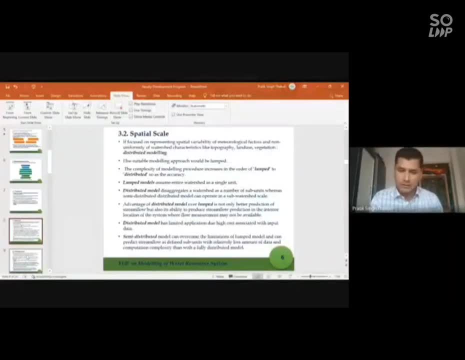 what is the purpose of your study? what? what is the purpose of your study? what amount of time you have, what amount of amount of time you have, what amount of amount of time you have, what amount of data you have? that would be very data you have. that would be very. 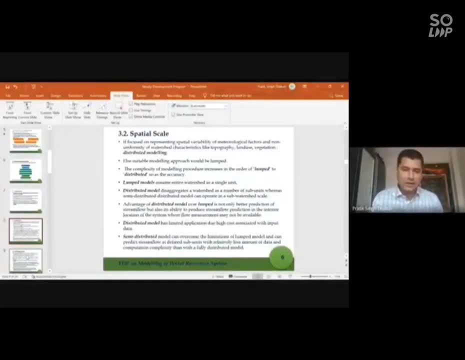 data you have. that would be very important, while important, while important, while selecting the spatial scale, uh dealing selecting the spatial scale, uh dealing selecting the spatial scale, uh dealing with the spatial scale of the, with the spatial scale of the, with the spatial scale of the hydrological model, 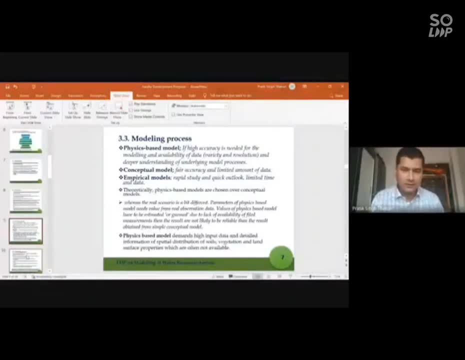 the third thing is the modeling processes. the third thing is the modeling processes. the third thing is the modeling processes. it is the physics best model conceptual. it is the physics best model conceptual. it is the physics best model conceptual model. empirical model model. empirical model conceptual. yeah, i'll go with the empirical to. 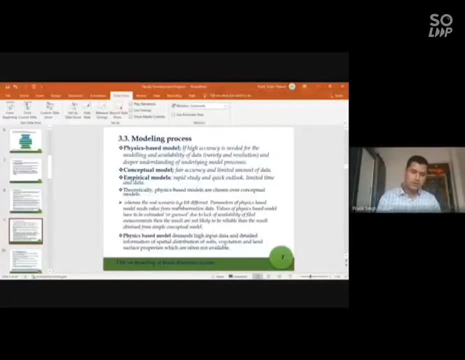 yeah, i'll go with the empirical to- yeah, i'll go with the empirical to the physical best model, the physical best model, the physical best model. so the empirical models, so the empirical models. so the empirical models are you know, they are, you know they are, you know they are used for rapid study, and you know. 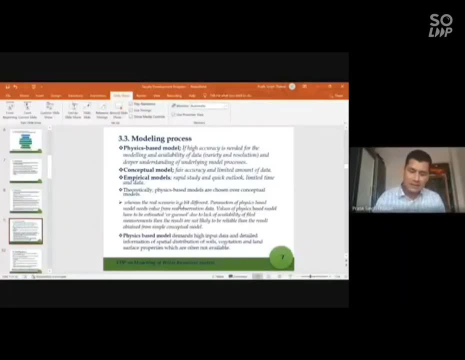 are used for rapid study and you know are used for rapid study and you know like a quick outlook and if you have like a quick outlook and if you have like a quick outlook and if you have limited time and data, just like limited time and data, just like. 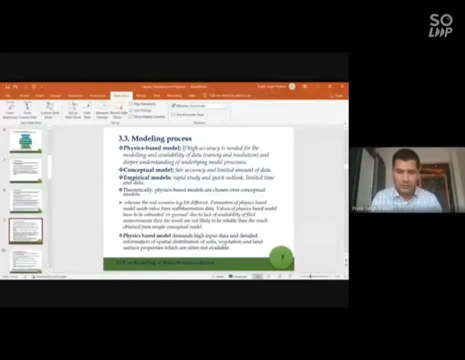 limited time and data, just like i have told um about the, i have told um about the, i have told um about the lump model, if you have really lump model, if you have really lump model, if you have really limited data and you know you are going limited data and you know you are going. 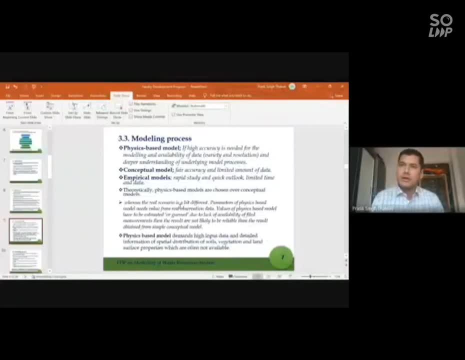 limited data and you know you are going to use the empirical models. just like to use the empirical models, just like to use the empirical models, just like they are rational formula, or, or they are rational formula, or, or they are rational formula, or, or something like unit hydrograph model. you. 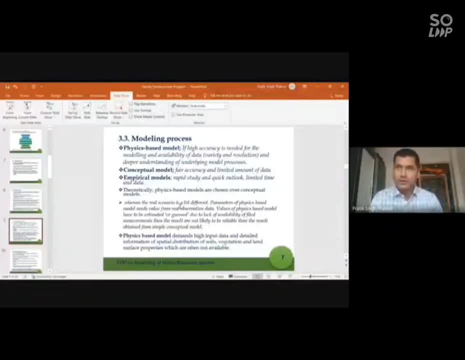 something like unit hydrograph model. you, something like unit hydrograph model, you just go for it and just go for it and just go for it and estimate the flow hydrograph of the estimate, the flow hydrograph of the estimate, the flow hydrograph of the watershed. 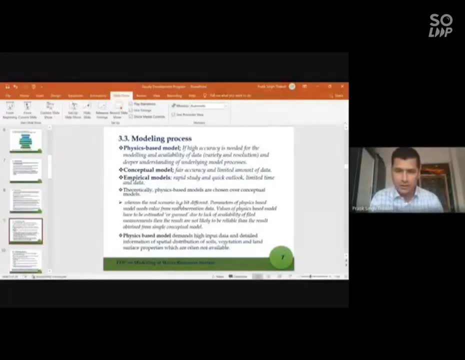 watershed, watershed. but. but if you, if you really demand but, but if you, if you really demand, but, but if you, if you really demand high accuracy of the model and you if high accuracy of the model and you if high accuracy of the model and you if you really have a high 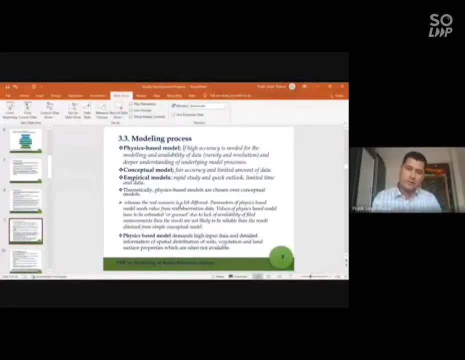 you really have a high. you really have a high. you know availability of the data and also you know availability of the data and also you know availability of the data and also um, um, um, but it demands high data. you know the um and the, but it demands high data. you know the um and the. 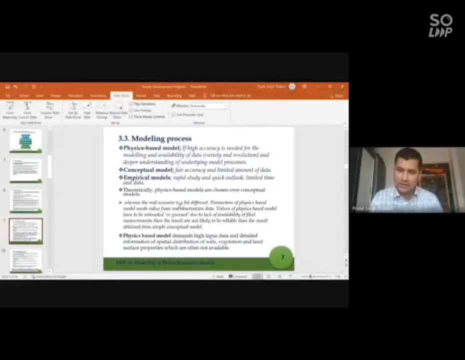 but it demands high data. you know the um and the modeler also, modeler also, modeler also. should have a very deeper understanding of, should have a very deeper understanding of, should have a very deeper understanding of the hydrological processor, the hydrological processor, the hydrological processor, uh. whereas the conceptual model has a 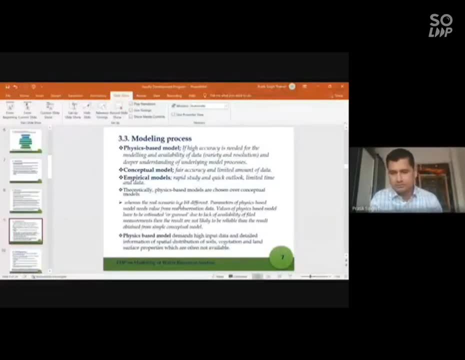 uh, whereas the conceptual model has a uh, whereas the conceptual model has a fear. accuracy unlimited. you know and fear. accuracy unlimited, you know and fear. accuracy unlimited, you know. and the, the, the, the amount of data. uh is also the amount of data. uh is also the amount of data. uh is also comparatively less um, the data demand is. 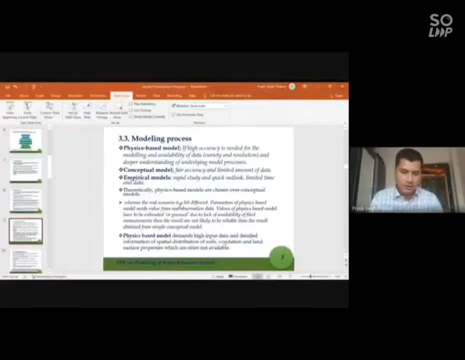 comparatively less um. the data demand is comparatively less um the data demand is also comparative, less compared to the. also comparative, less compared to the. also comparative, less compared to the physics-based model. so so, physics-based model, so so, physics-based model, so so, like uh, semi-distributed model, that the 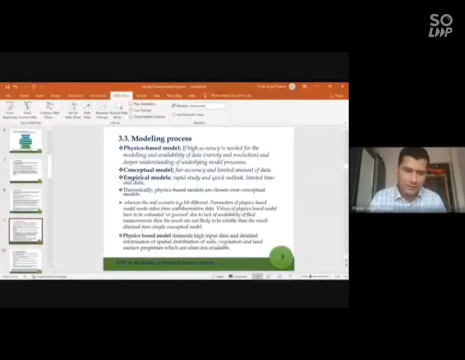 like uh semi-distributed model that the like uh semi-distributed model. that the, the, the, the conceptual model. overcome the drawbacks conceptual model. overcome the drawbacks conceptual model. overcome the drawbacks of empirical model and the physics-based of empirical model and the physics-based of empirical model and the physics-based model as well. but 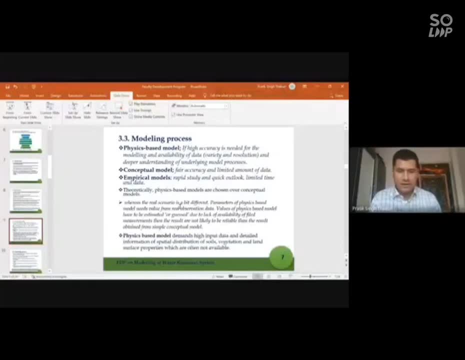 model as well, but model as well, but, as i've already told that, as i've already told that, as i've already told that, there are, you know, there are, you know, there are, you know. the models are selected based on the. the models are selected based on the. 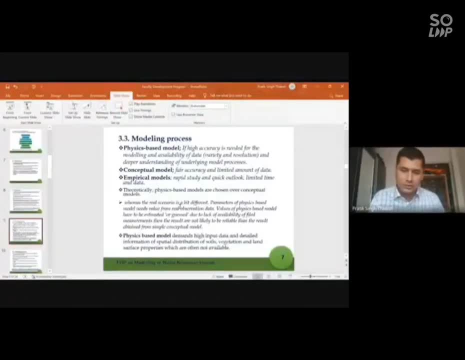 the models are selected based on the models requirement, their, their, the models requirement, their, their, the models requirement, their, their, the purpose of the modeling. so that would purpose of the modeling, so that would purpose of the modeling, so that would be. that is the important factor. be that is the important factor. 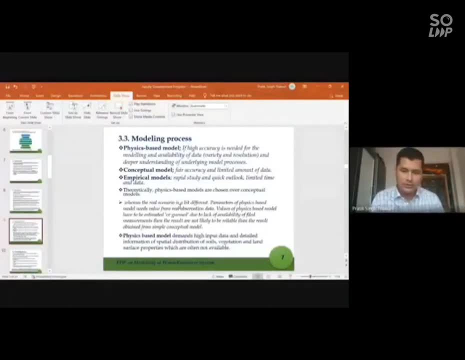 be. that is the important factor: what, where, what and where you should go. what, where, what and where you should go. what, where, what and where you should go? and uh, how should you choose the and uh, how should you choose the and uh, how should you choose the model? so, um, 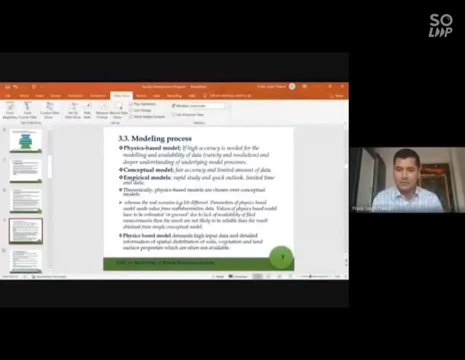 model so um model so um looking at the modeling criteria, you looking at the modeling criteria. you looking at the modeling criteria, you should you should go. if you have um should, you should go. if you have um should, you should go. if you have um deeper understanding of the watershed. 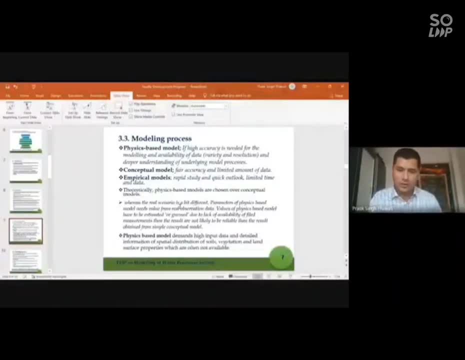 deeper understanding of the watershed, deeper understanding of the watershed processes and high amount of data then processes and high amount of data then processes and high amount of data, then the physics-based model would be really the physics-based model would be really the physics-based model would be really good. 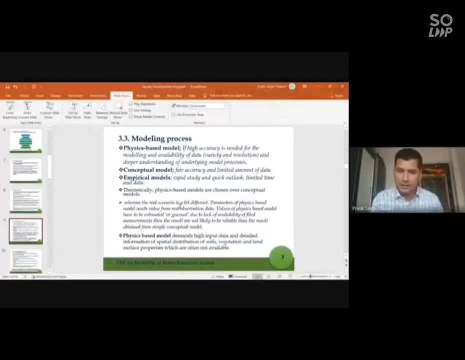 good, good uh else, you know if you have uh. if you uh else, you know if you have uh. if you uh else, you know if you have uh. if you are going for a rapid case study, you are going for a rapid case study. you are going for a rapid case study. you just go for the empirical model. so 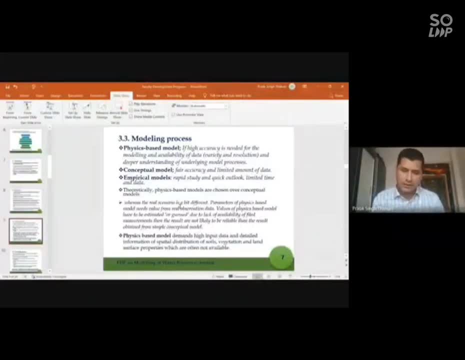 just go for the empirical model. so just go for the empirical model. so you cannot say that this model is the. you cannot say that this model is the, you cannot say that this model is the best and ideal or perfect model. so best and ideal or perfect model. so 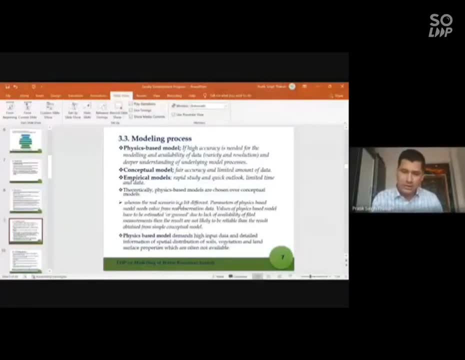 best and ideal or perfect model. so, and the real scenario is quite different and the real scenario is quite different and the real scenario is quite different. you know, you know, you know uh physics-based model. uh are generally uh physics-based model. uh are generally uh physics-based model. uh are generally selected over conceptual model. but 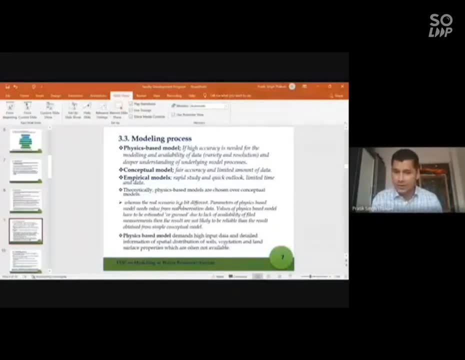 selected over conceptual model, but selected over conceptual model. but parameters of physics-based model needs a parameters of physics-based model needs a parameters of physics-based model needs a value from real observation data and value from real observation data and value from real observation data and values of real object model have 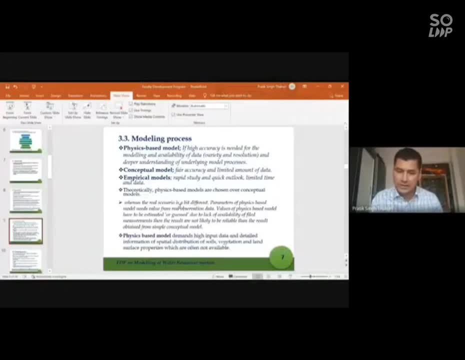 values of real object model have. values of real object model have. if the values of real physics model, if the values of real physics model, if the values of real physics model have to be stimulated or guessed due to have to be stimulated or guessed due to have to be stimulated or guessed due to lack of ability of. 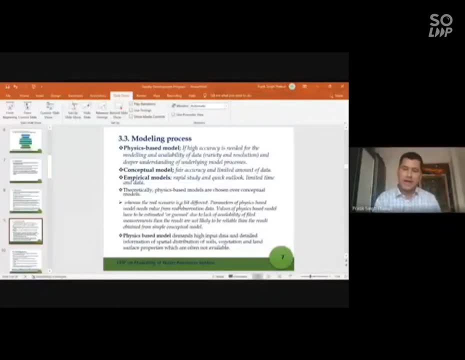 lack of ability, of lack of ability of um you know field measurement, then the um you know field measurement, then the um you know field measurement, then the result is not likely to be reliable. uh result is not likely to be reliable. uh result is not likely to be reliable uh than the result obtained from the simple. 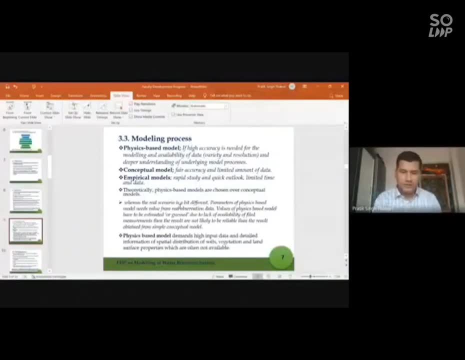 than the result obtained from the simple, than the result obtained from the simple. conceptual model, conceptual model, conceptual model: so yeah, so the physics-based model? so yeah, so the physics-based model. so yeah, so the physics-based model. often require the data from the. often require the data from the. 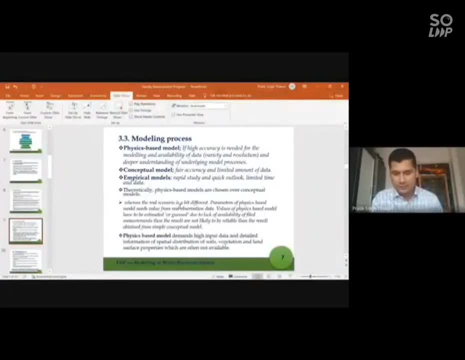 often require the data from the. you know from the real observation data. you know from the real observation data. you know from the real observation data and if, in the absence of, and if in the absence of, and if in the absence of real observation data, if you guess or? 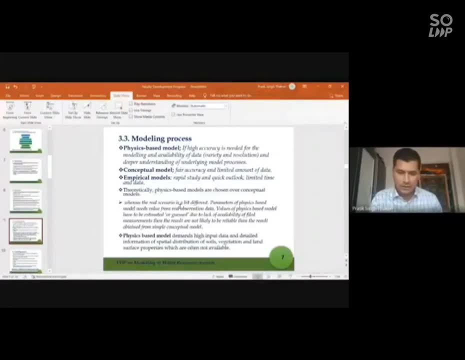 real observation data. if you guess, or real observation data, if you guess or estimate those data. and estimate those data and estimate those data and enter it in the model, then the result enter it in the model. then the result enter it in the model. then the result are likely to be: 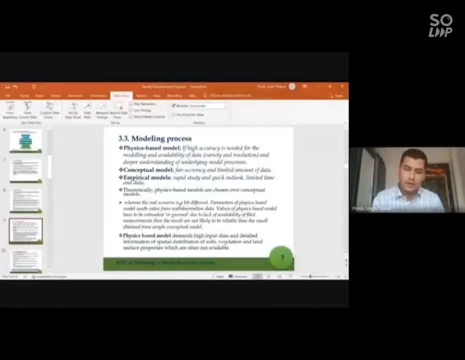 are likely to be, are likely to be, less reliable than the result obtained, less reliable than the result obtained, less reliable than the result obtained from the conceptual model, so um from the conceptual model, so um from the conceptual model, so um, so, so so. conceptual model in, so so so. conceptual model in. 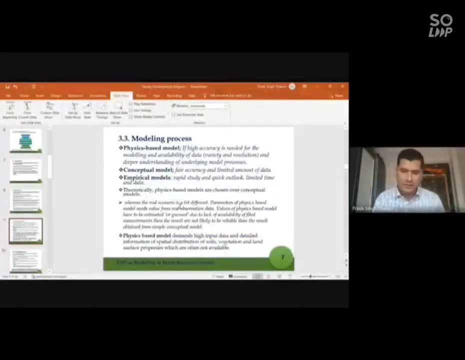 so, so, so, conceptual model in, you know, you know, you know so, so. so, in the absence or in the absence of, in the absence or in the absence of, in the absence or in the absence of real observation data, you should you, real observation data, you should you. 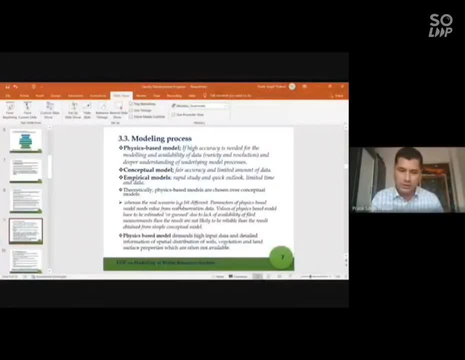 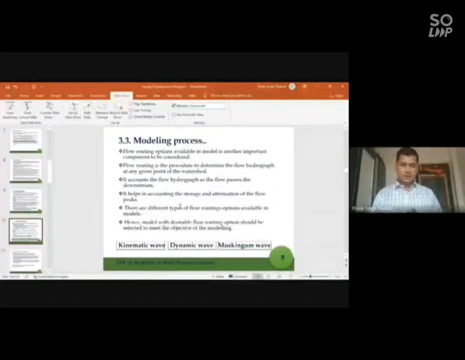 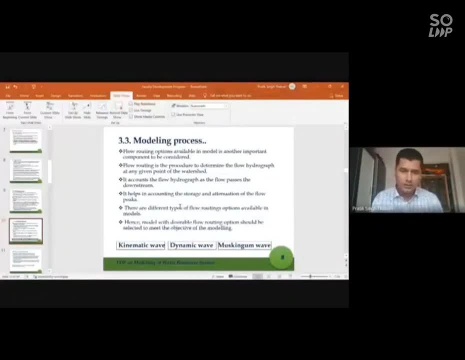 thing, another component in the model thing, another component in the model: processes would be flow routing. you know processes would be flow routing. you know processes would be flow routing. you know the flow routing, the flow routing, the flow routing processes available in the model, so flow processes available in the model, so flow. 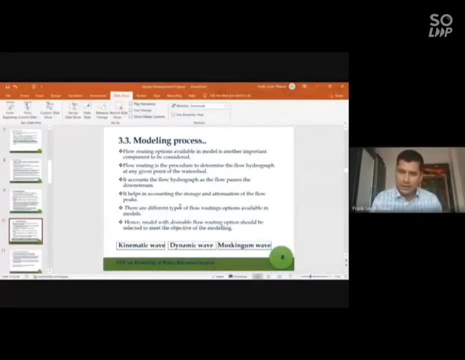 processes available in the model. so flow routing option available are available, routing option available are available, routing option available are available in the model in, in the model in in. there's another important, there's another important, there's another important component to be considered, component to be considered. 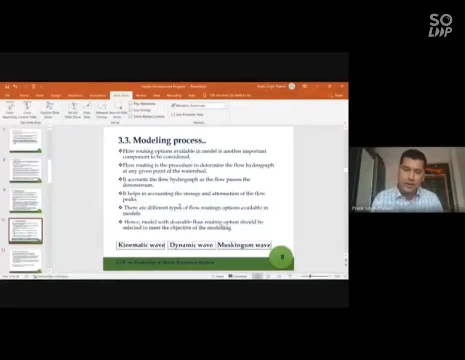 component to be considered. so flow routing is the processor to so flow routing is the processor to so flow routing is the processor to determine flow hydrograph at any given determine flow hydrograph at any given determine flow hydrograph at any given point of the watershed. it accounts the point of the watershed. it accounts the point of the watershed, it accounts the flow, flow flow hydrograph as a flow passes, the downstream hydrograph as a flow passes the downstream hydrograph as a flow passes the downstream. and it helps in the accounting the. and it helps in the accounting the. 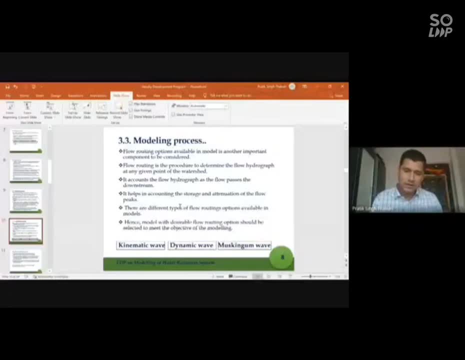 and it helps in the accounting. the stories and attenuation of the flow picks. stories and attenuation of the flow picks. stories and attenuation of the flow picks. similarly, there are different type of. similarly, there are different type of. similarly, there are different type of flow routing option available in the. 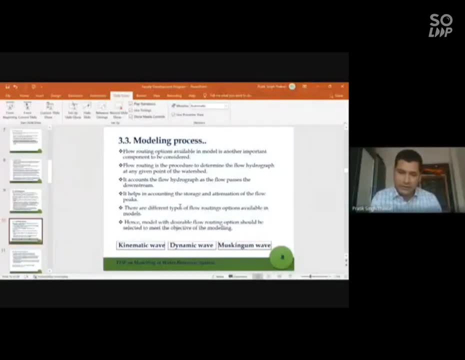 flow routing option available in the flow routing option available in the model. so hence the model with the model. so hence the model with the model. so hence the model with the desirable flow routing should be selected. desirable flow routing should be selected. desirable flow routing should be selected to meet the objective of the model. so 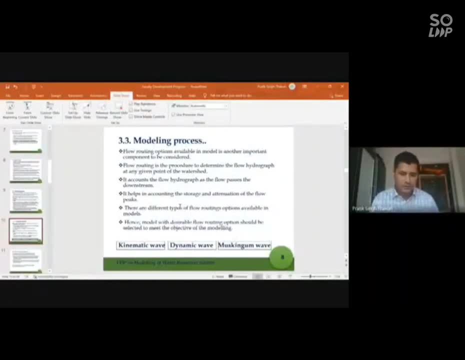 to meet the objective of the model. so to meet the objective of the model. so there are, you know, basically you can. there are, you know, basically you can. there are, you know, basically you can classify the flow routing process into. classify the flow routing process into. classify the flow routing process into kinematic 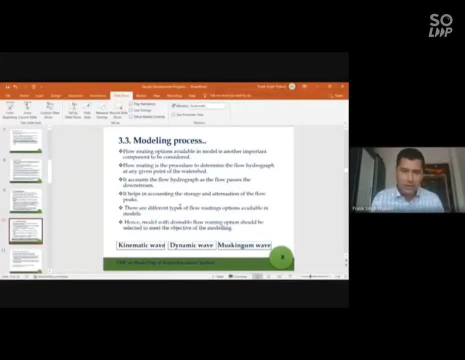 kinematic: kinematic um dynamic or musking with you know um dynamic or musking with you know um dynamic or musking with you know flow routing and the requirement or the flow routing and the requirement or the flow routing and the requirement or the peculiarity of your watershed or the 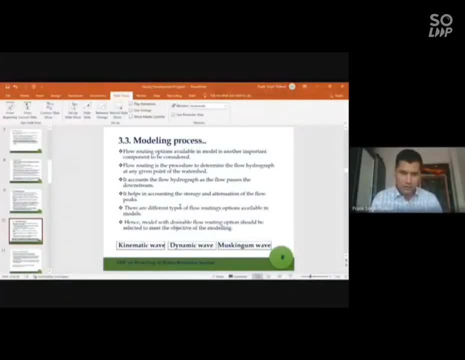 peculiarity of your watershed, or the peculiarity of your watershed or the level of data you have. understanding you, level of data you have. understanding you, level of data you have. understanding you have. you should go for the flow routing. have. you should go for the flow routing. 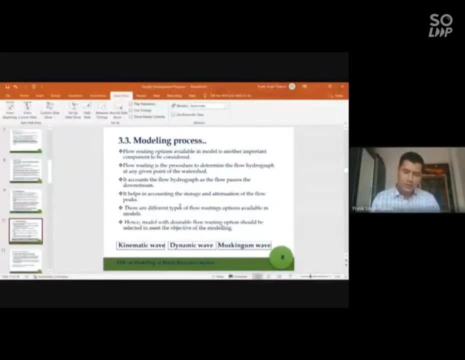 have. you should go for the flow routing, um, um, um selection as well. so the model which have selection as well, so the model which have selection as well, so the model which have your desirable flow routing option. you, your desirable flow routing option, you, your desirable flow routing option. you know from for uh, from my. 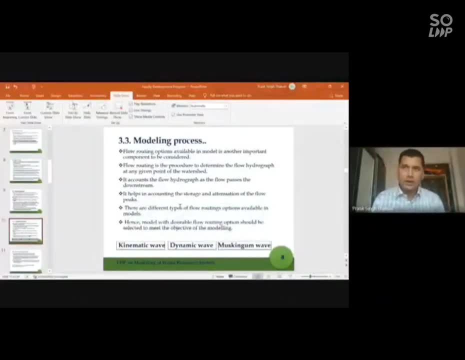 know from for uh, from my know from for uh, from my one study. it was, it was one study, it was, it was one study, it was. it was in the hilly areas and in the hilly areas and in the hilly areas, and for me, for me. 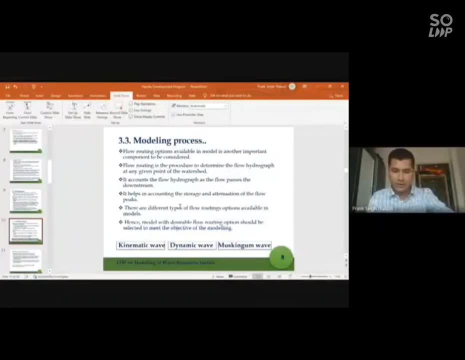 for me. they have, they have, they have. i have done a literature review, and then i have done a literature review, and then i have done a literature review and then i have known that that the dynamic wave, i have known that, that the dynamic wave, i have known that that the dynamic wave method for flow routing would be. 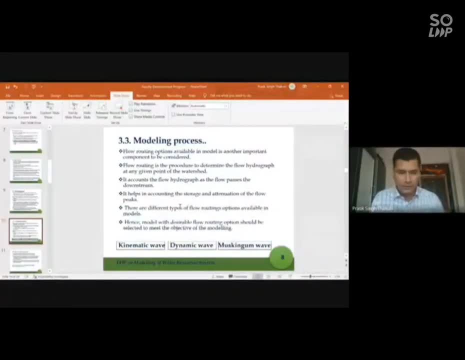 method for flow routing would be. method for flow routing would be good for good, for good for the modeling uh. the watershed with the modeling uh, the watershed with the modeling uh, the watershed with in the way that the slope of the, in the way that the slope of the 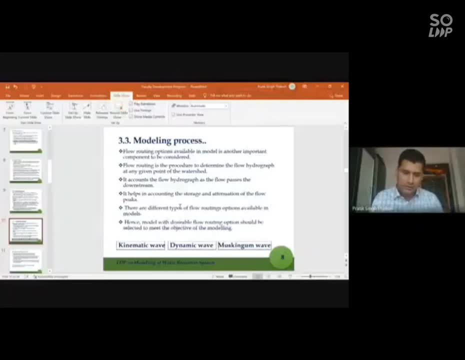 in the way that the slope of the terrain is quite steep, so terrain is quite steep, so terrain is quite steep. so the. what are the options available in the? what are the options available in the? what are the options available in the hydrological model that should be? 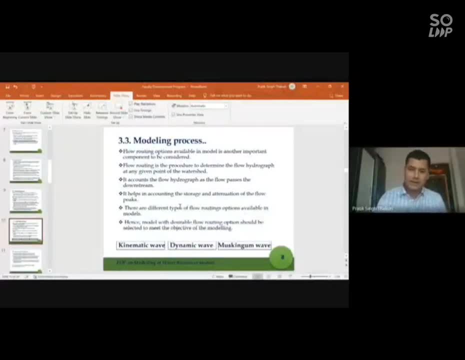 the hydrological model. that should be the hydrological model that should be also be considered in, also be considered in, also be considered in while selecting the hydrological, while selecting the hydrological, while selecting the hydrological processes. hydrological modern processing processes. hydrological modern processing. 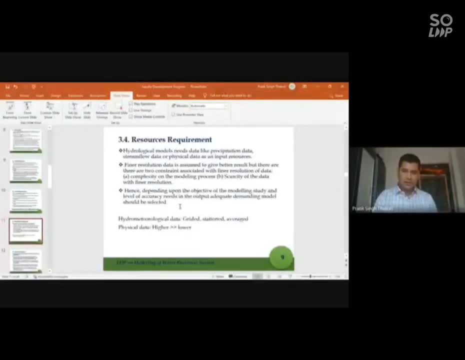 processes: hydrological modern processing in the hydrological model selection in the hydrological model selection, in the hydrological model selection. similarly the resource requirement, similarly the resource requirement, similarly the resource requirement. i have already told that the hydrological, i have already told that the hydrological. 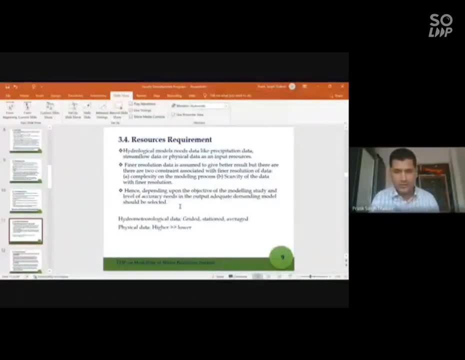 i have already told that the hydrological model needs model needs. model needs: uh precipitation data, stream flow data. uh precipitation data stream flow data. uh precipitation data stream flow data. physical data as input resources. so physical data as input resources. so physical data as input resources. so final resolution is assumed to be a: 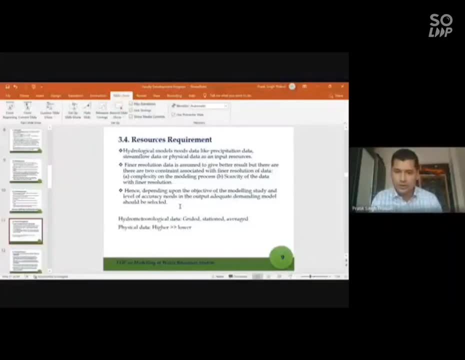 final resolution is assumed to be a final resolution is assumed to be a better, better, better, give better result, but there are two give better result, but there are two give better result, but there are two constraints associated with the final constraints associated with the final constraints associated with the final resolution data, that is, the complexity on 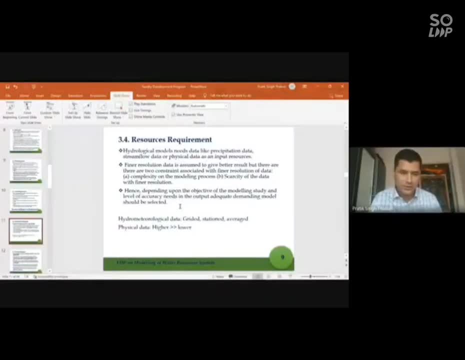 resolution data. that is the complexity on resolution data, that is the complexity on the model and the scarcity of the data, the model and the scarcity of the data, the model and the scarcity of the data, with the final resolution. so hence, with the final resolution, so hence with the final resolution, so hence, depending on the objective of the. 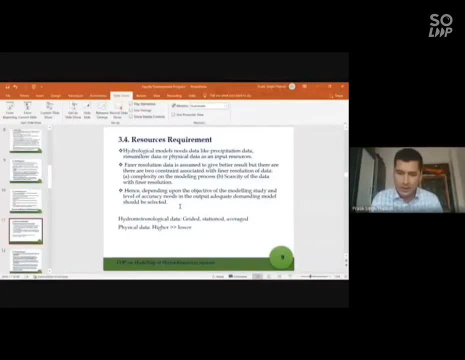 depending on the objective of the, depending on the objective of the: modeling study level of accuracy needed. modeling study: level of accuracy needed. modeling study: level of accuracy needed: um, um, um and the output advocate and the output advocate and the output advocate. demanding model should be. demanding model should be. 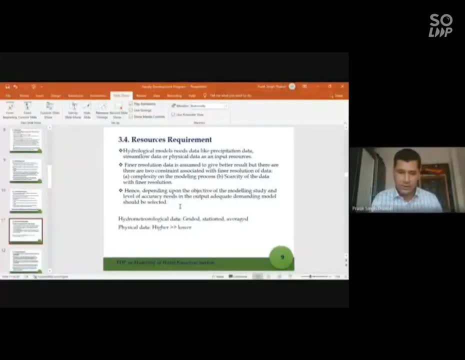 demanding model should be: should be selected, so should be selected, so should be selected. so, as i have already told um, as i have already told um, as i have already told um, that the, that, the, that the resource requirement, it would be the resource requirement, it would be the. 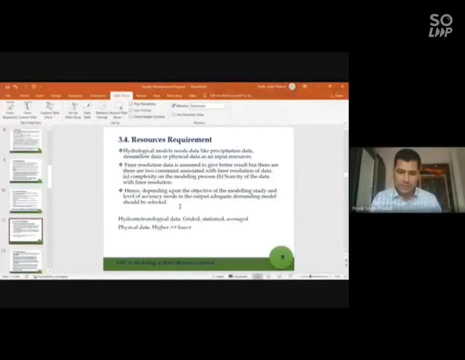 resource requirement. it would be the important criteria while selecting the important criteria, while selecting the important criteria while selecting the hydrological model. so hydrological model, so hydrological model. so, resources: uh, what the resources, you know resources. uh, what the resources, you know resources. uh, what the resources, you know the. 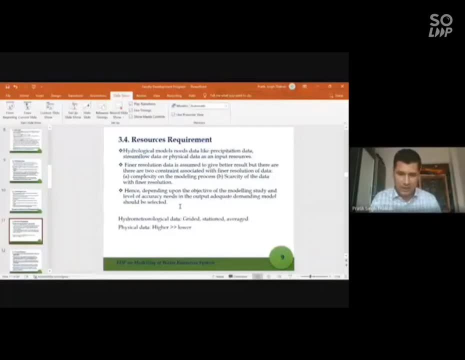 the, the you require, for, you require, for, you require for: while developing the hydrological model, while developing the hydrological model, while developing the hydrological model, i have classified into two. that is, i have classified into two. that is, i have classified into two. that is hydrological. 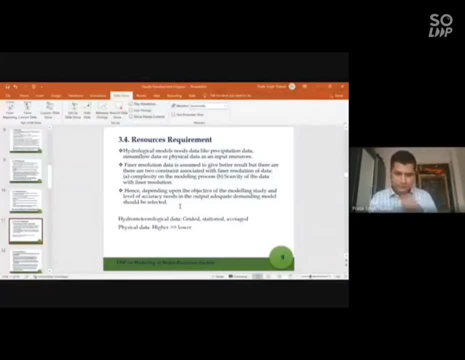 hydrological hydrological hydrometeorological data and physical hydrometeorological data and physical hydrometeorological data and physical data data data so in the hydrological hydrometeorological, so in the hydrological hydrometeorological. 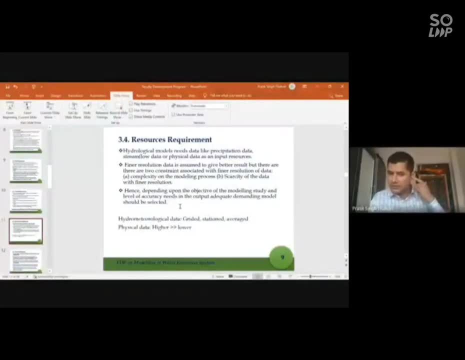 so in the hydrological hydrometeorological data, so in the hydrological hydrometeorological, especially if you say the, especially if you say the, especially if you say the precipitation or metallurgical data. precipitation or metallurgical data. precipitation or metallurgical data that can be classified into a predated 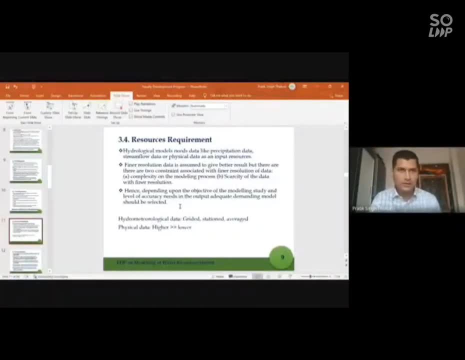 that can be classified into a predated. that can be classified into a predated, stationed or average, so stationed or average. so stationed or average. so in some uh hydrological model, you need a in some uh hydrological model. you need a in some uh hydrological model. you need a gridded precipitation data or 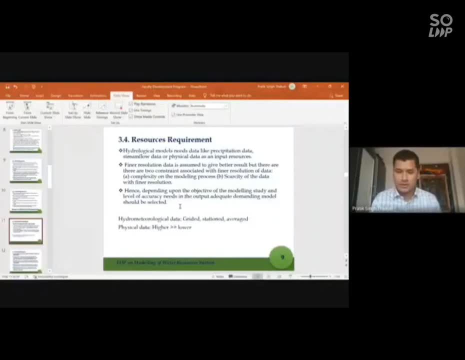 gridded precipitation data or gridded precipitation data, or in some hydrological model. you need you in some hydrological model. you need you in some hydrological model. you need, you may need a station, may need a station, may need a station data, or in some hydrological model, if you. 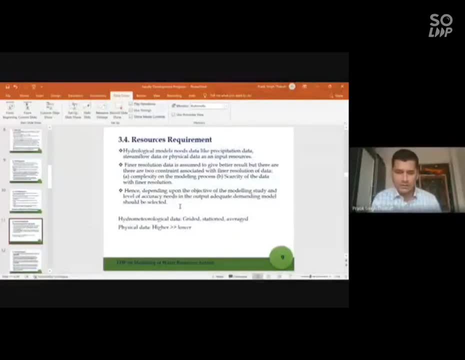 data or in some hydrological model, if you data or in some hydrological model, if you have just an average, have just an average, have just an average, decent polygon data or average data, and decent polygon data or average data and decent polygon data or average data. and that would be the- you know the surface. 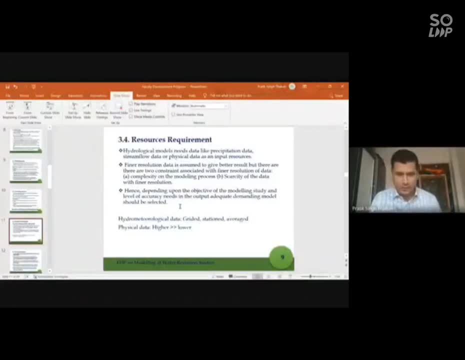 that would be the. you know the surface. that would be the you know the surface. so so, so, what is the data requirement for the, what is the data requirement for the, what is the data requirement for the model and what is your ability in the model and what is your ability in the? 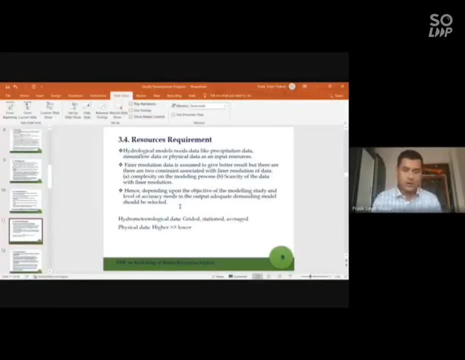 model and what is your ability in the watershed, watershed, watershed that should have. should have a that should have. should have a that should have. should have a compromised meat and similarly the compromised meat and similarly the compromised meat, and similarly the physical data as well. physical data as well. 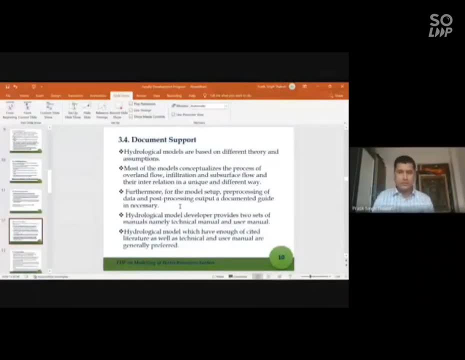 physical data as well. so another thing would be the document. so another thing would be the document. so another thing would be the document. support you know the hydrological model. support you know the hydrological model. support you know the hydrological model. are based on theory and assumption. are based on theory and assumption. are based on theory and assumption and model of the most of the model and model of the most of the model and model of the most of the model. conceptualizes the process of overland. conceptualizes the process of overland. conceptualizes the process of overland flow infiltration. 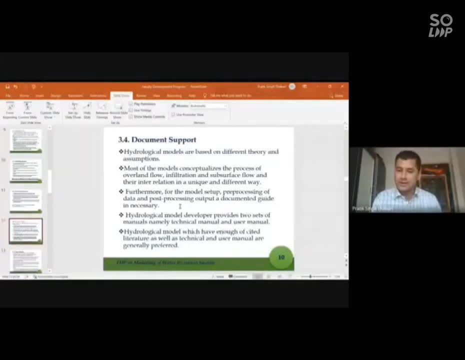 flow infiltration flow infiltration: uh soft surface flow and their uh soft surface flow and their uh soft surface flow and their interrelation in very unique and interrelation in very unique and interrelation in very unique and different way. most of the models, different way. most of the models. 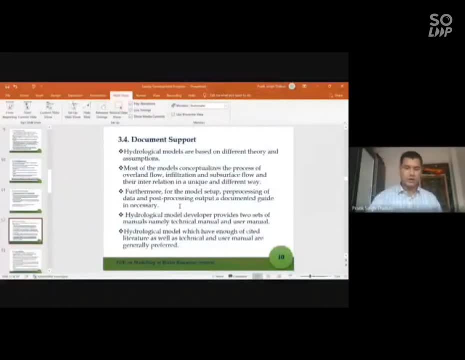 different way most of the models, the conceptualization of the processes. the conceptualization of the processes. the conceptualization of the processes varies from model to model, varies from model to model, varies from model to model. for the model setup: pre-processing a. for the model setup: pre-processing a. 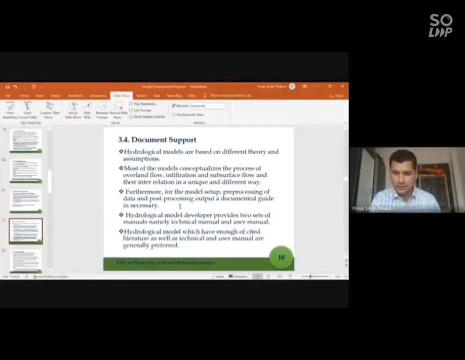 for the model setup- pre-processing, a post-processing of output, post-processing of output, post-processing of output. need a documented need, a documented need, a documented guidance. so model uh- hydrological model guidance. so model uh- hydrological model guidance. so model uh- hydrological model, you know, basically develops two shades. 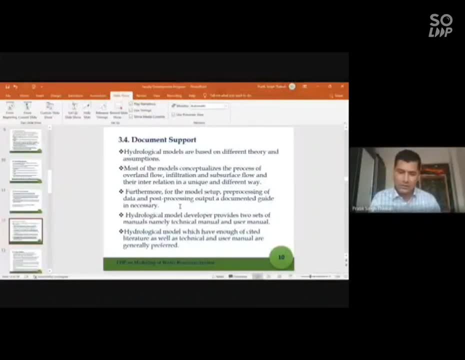 you know, basically develops two shades. you know, basically develops two shades of my manuals, namely a technical manual of my manuals, namely a technical manual of my manuals, namely a technical manual and user manual. so technical manual, you and user manual. so technical manual, you and user manual. so technical manual. you know, give the underlying processes how. 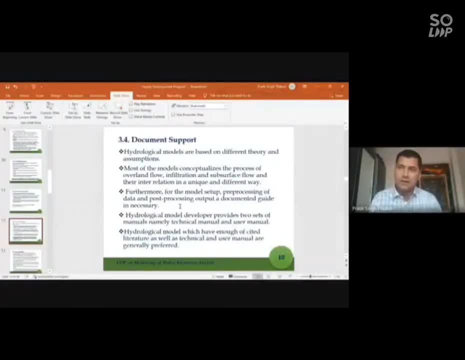 know give the underlying processes. how know give the underlying processes how it is being calculated whereas the user it is being calculated. whereas the user it is being calculated whereas the user manual usually give how the model should manual usually give how the model should manual usually give how the model should be dealt with, how it operates or the. 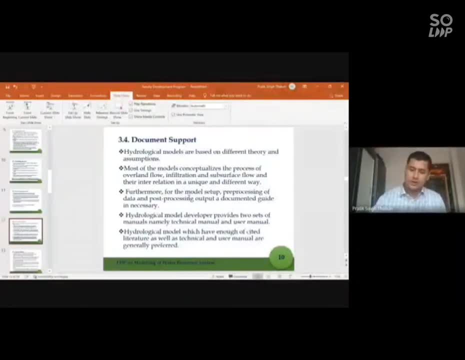 be dealt with how it operates, or the be dealt with how it operates, or the processes, processes, processes. about how it is going to be used. it about how it is going to be used. it about how it is going to be used. it should be used, so, should be used, so. 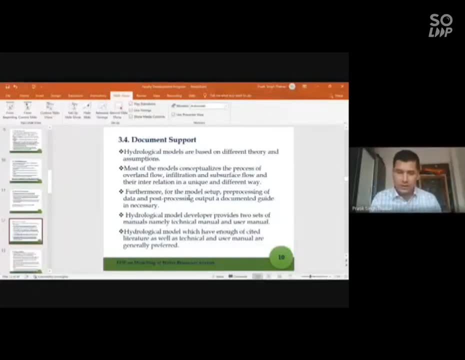 should be used. so generally, hydrological model developers generally, hydrological model developers, generally hydrological model developers, provide two set of manuals, provide two set of manuals, provide two set of manuals. uh so the hydrological model um another. uh so the hydrological model um another. uh so the hydrological model um another thing. 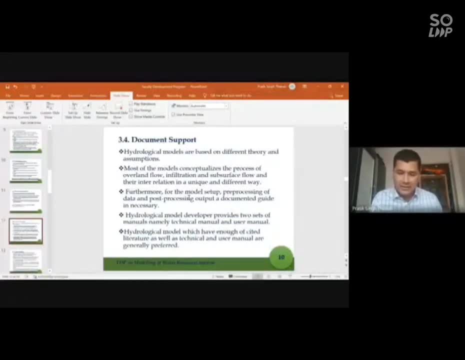 thing, thing. thing is the model which has been you know. thing is the model which has been you know, is the model which has been, you know, you know, cited in literature with the. you know, cited in literature with the, you know, cited in literature with the, and have also have the technical and 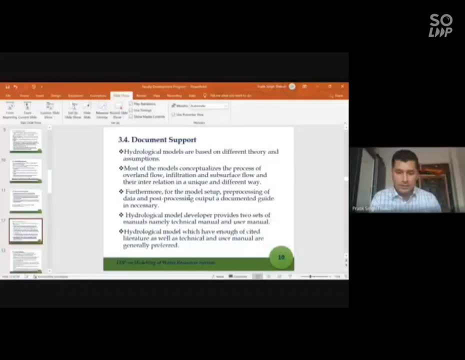 and have also have the technical and and have also have the technical and user manual available. are generally user manual available. are generally user manual available. are generally preferred, preferred, preferred. uh, you know, uh, you know, uh, you know, if you have, if you have, if you, if you have, if you have, if you. 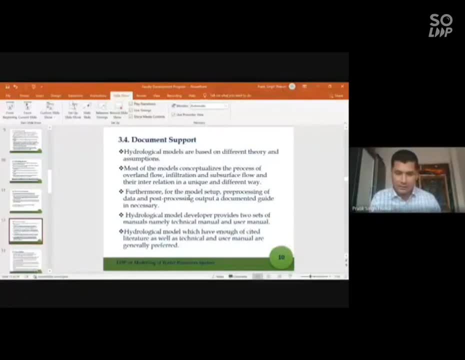 if you have, if you have enough information, or you have enough, have enough information, or you have enough, have enough information. or you have enough idea of the idea, of the idea of the underlying processes, then it's good. but underlying processes, then it's good. but underlying processes, then it's good. but in the absence of you know technical, 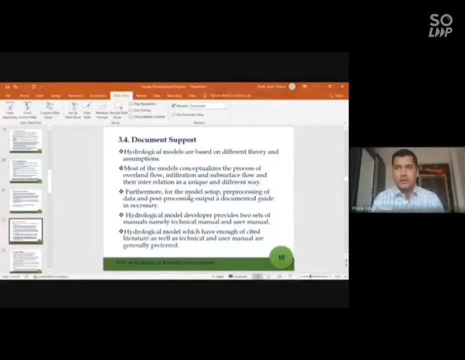 in the absence of you know technical, in the absence of you know, technical manual and user manual. those manual and user manual, those manual and user manual. those ideological model would be just converted. ideological model would be just converted. ideological model would be just converted into the black box model. 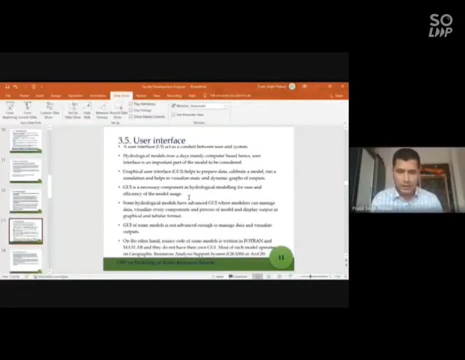 into the black box model, into the black box model. finally, finally, finally, another, another, another important criteria to be considered would important criteria to be considered, would important criteria to be considered, would be user interface. so so, user interface be user interface. so so user interface be user interface. so so, user interface is like a conduit between user and the 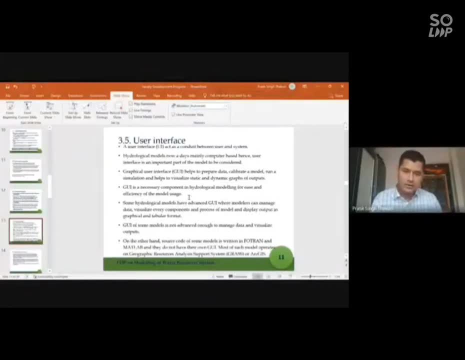 is like a conduit between user and the is like a conduit between user and the system, system of system, system of system, system of the model, the model, the model and ideological model nowadays mainly, and ideological model nowadays mainly and ideological model nowadays mainly, are computer based, are computer based. 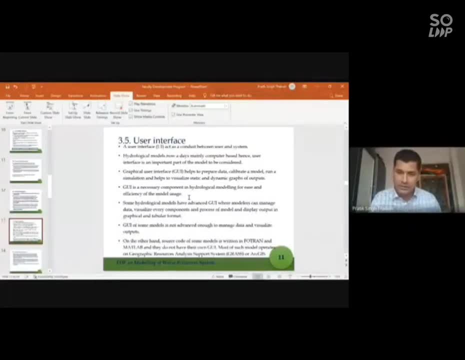 are computer based. the mathematical. they also called it the the mathematical. they also called it the the mathematical. they also called it the mathematical model. but it is completely mathematical model. but it is completely mathematical model. but it is completely based on computer and user imported the. based on computer and user imported the. 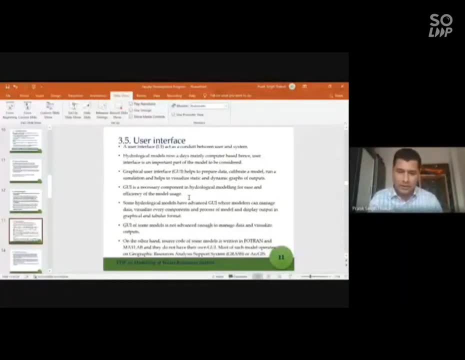 based on computer and user imported the user, user, user interface is an important part of the interface, is an important part of the interface, is an important part of the model to be considered, model to be considered, model to be considered. so graphical user interface, so graphical user interface. 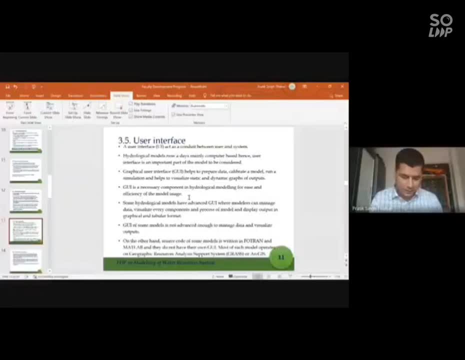 so graphical user interface. it is also known as ui. it is also known as ui. it is also known as ui are most common in these days. that helps are most common in these days. that helps are most common in these days. that helps to prepare data, calibrate model, run a. 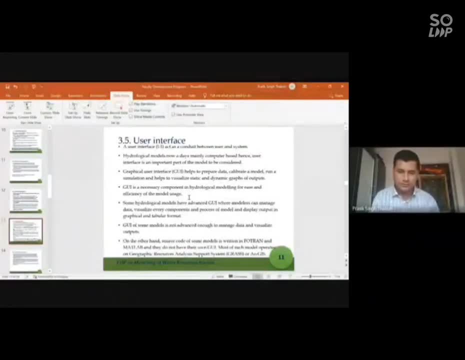 to prepare data calibrate model: run a. to prepare data calibrate model: run a simulation. help to visualize the static simulation. help to visualize the static simulation. help to visualize the static and dynamic graphs of the output. so gi is. and dynamic graphs of the output. so gi is. 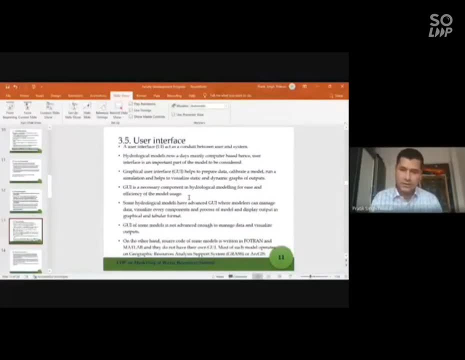 and dynamic graphs of the output. so gi is a necessary component in hydrological, a necessary component in hydrological, a necessary component in hydrological model for ease and efficiency of the model for ease and efficiency, of the model for ease and efficiency of the model users. model users: 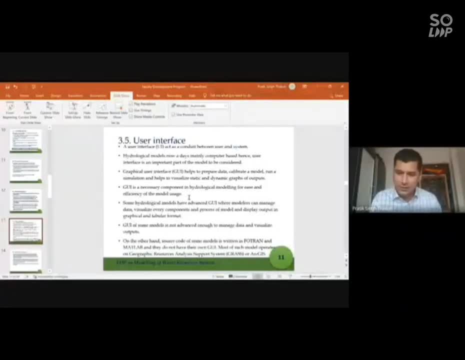 model users. so some hydrological model have advanced, so some hydrological model have advanced, so some hydrological model have advanced: gui whereas gui, whereas gui, whereas where model we can manage visualize and where model we can manage visualize and where model we can manage visualize and every component process of the model and 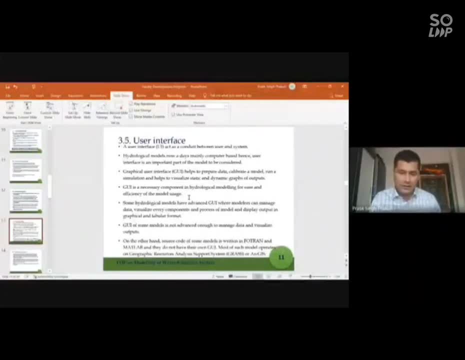 every component process of the model and every component process of the model and display output in the graphical and display output. in the graphical and display output in the graphical and tabular format, tabular format. tabular format. so gi of the some model are not advanced, so gi of the some model are not advanced. 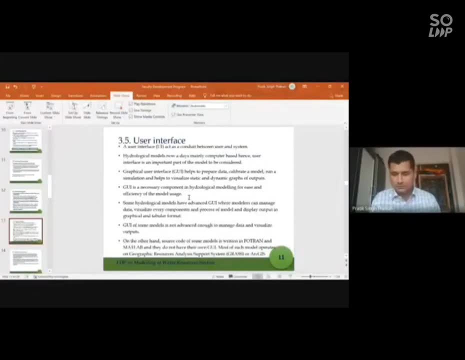 so gi of the, some model are not advanced enough to manage and visualize the output, enough to manage and visualize the output, enough to manage and visualize the output. uh, and you know, uh and you know, uh and you know, in other hand, some model have, uh, they. in other hand, some model have, uh, they. 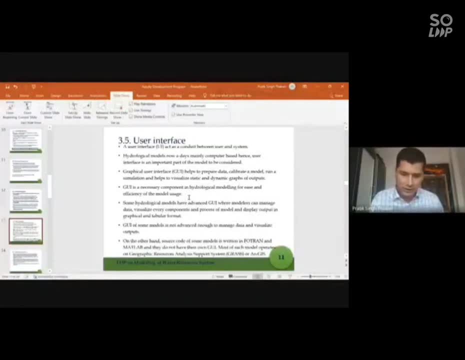 in other hand, some model have, uh, they don't have their own, uh don't have their own, uh don't have their own. uh, you know the platform, uh and they. you know the platform, uh and they. you know the platform, uh and they. they are written in fortran or matlab and 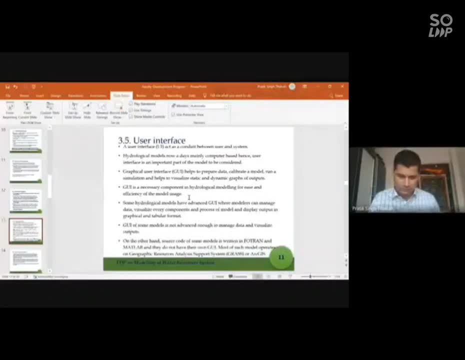 they are written in fortran or matlab and they are written in fortran or matlab and they have. they don't have their own, they have. they don't have their own, they have. they don't have their own platform and they should go for platform and they should go for. 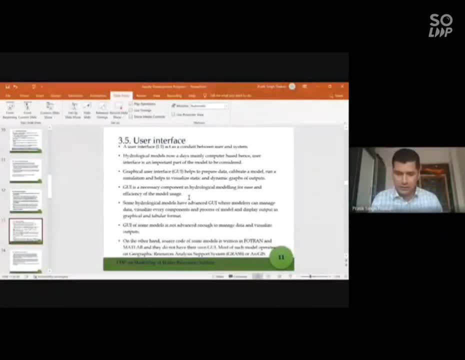 platform and they should go for um, um, um the platform, the other, the the platform, the other, the the platform, the other, the third-party platform, just like a grass third-party platform, just like a grass third-party platform, just like a grass or or arcgis, or qgis platform. they should. 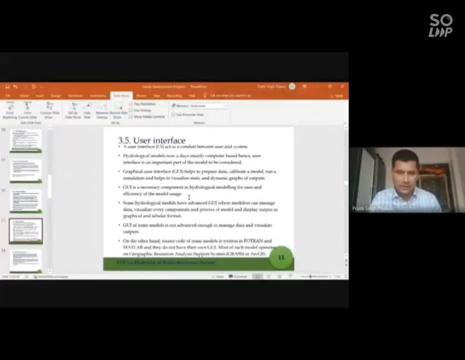 or or arcgis or qgis platform they should, or or arcgis or qgis platform they should use. so, use, so, use. so there are uh, as i have told that there. there are. uh, as i have told that there. there are. uh, as i have told that there are. 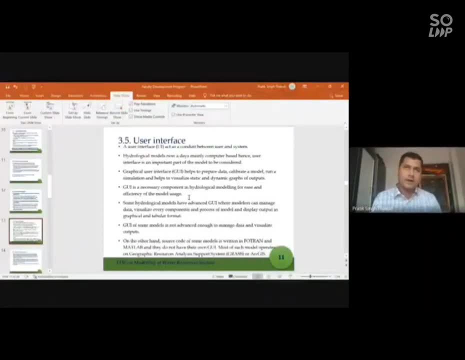 are are numerous models. so nowadays the computer, numerous models. so nowadays the computer, numerous models. so nowadays the computer models, models, models. uh do have their own uh graphical user, uh do have their own uh graphical user, uh do have their own uh graphical user interface and they are quite advancing. 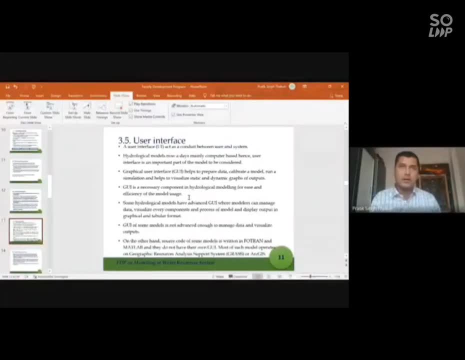 interface and they are quite advancing interface and they are quite advancing but, but, but there are. there are also the there are. there are also the there are. there are also the hydrological model which do not have hydrological model, which do not have hydrological model, which do not have their own. 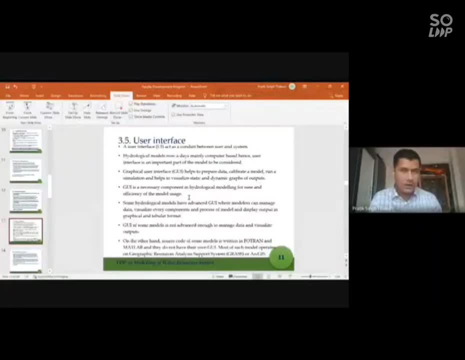 their own. their own um a graphical user interface and some um a graphical user interface, and some um a graphical user interface, and some uh hydrological model. uh hydrological model, uh hydrological model. just uh perform in the spreadsheet or in. just uh perform in the spreadsheet or in. 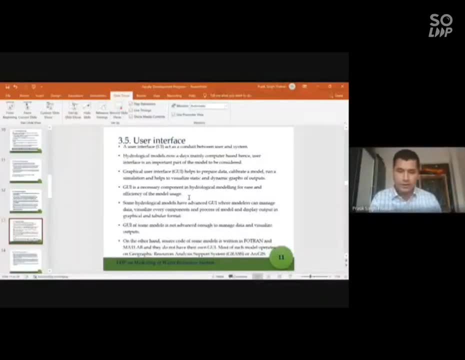 just uh perform in the spreadsheet or in the the the excel with the- uh, the mathematical code. excel with the- uh, the mathematical code. excel with the- uh, the mathematical code. so so so what is your requirement and what is the? what is your requirement and what is the? 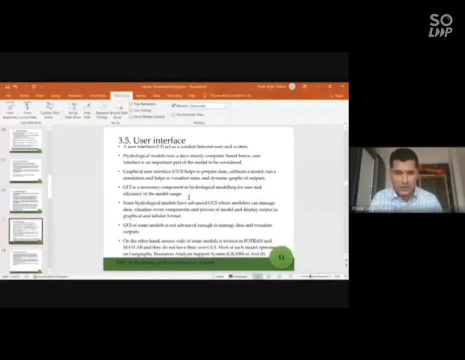 what is your requirement and what is the uh? the- their preferences on the ease of uh. the their preferences on the ease of uh. the their preferences on the ease of ease of use. ease of use, ease of use- uh, that would be also considered. uh, that would be also considered. 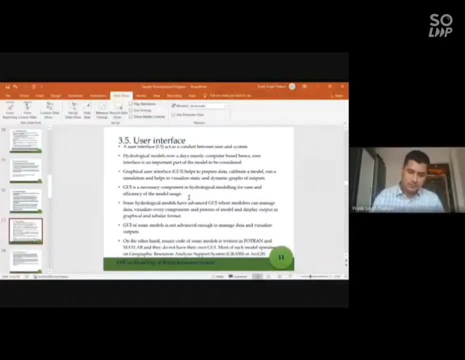 uh, that would be also considered in the user interface criteria of model, in the user interface criteria of model. in the user interface criteria of model selection, selection, selection, the um sixth criteria for model. the um sixth criteria for model. the um sixth criteria for model selection is model calibration. 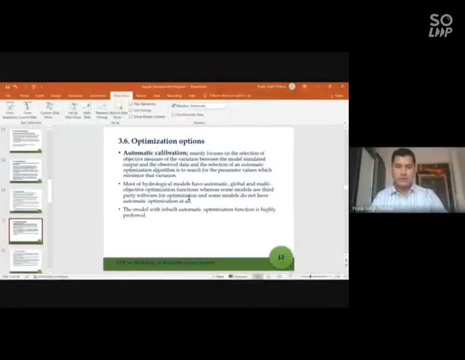 selection is model calibration, selection is model calibration, so automatic calibration, and you know so automatic calibration and you know so automatic calibration, and you know you can. you can classify a model um you can. you can classify a model um you can. you can classify a model um optimization into. you know the manual. 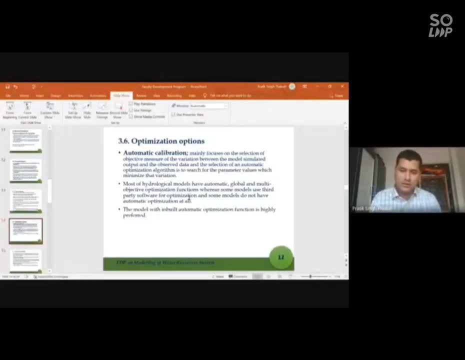 optimization, into you know the manual optimization, into you know the manual optimization and optimization, and optimization and automatic optimization. so the automatic optimization, so the automatic optimization, so the automatic calibration, automatic calibration, automatic calibration: if we talk about it is many focuses on. if we talk about it is many focuses on. 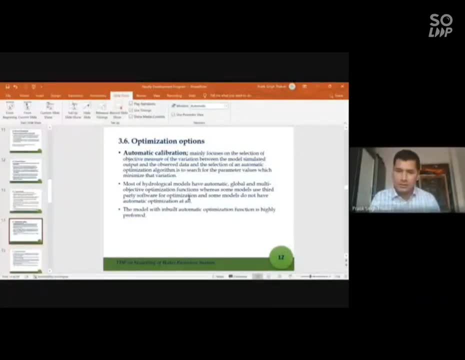 if we talk about it is many focuses on the selection of the selection of the selection of objective measure of variation between objective measure of variation, between objective measure of variation between model simulated output and observed data, model simulated output and observed data, model simulated output and observed data, and the selection of optimization. 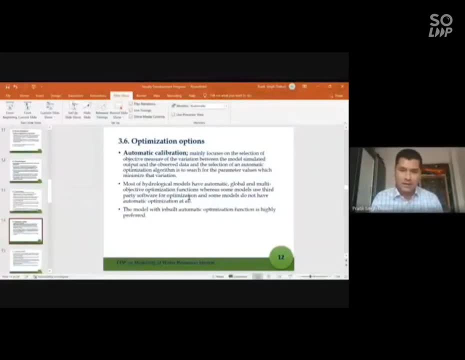 and the selection of optimization and the selection of optimization algorithm. to search the parameter value algorithm. to search the parameter value algorithm. to search the parameter value with minimize, with minimize, with minimize. is that variation so automatic? is that variation so automatic? is that variation so automatic? calibration is: 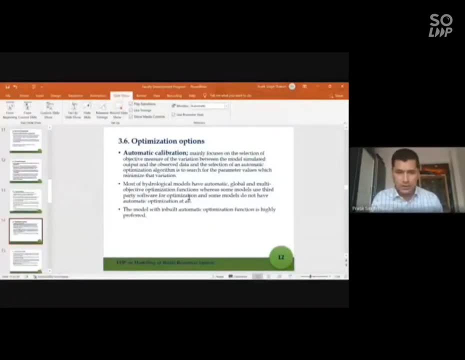 calibration is. calibration is the method which which, the method which which, the method which which look for the look for the look for the observed data and the simulated data and observed data and the simulated data, and observed data and the simulated data, and try to minimize the variation of those. 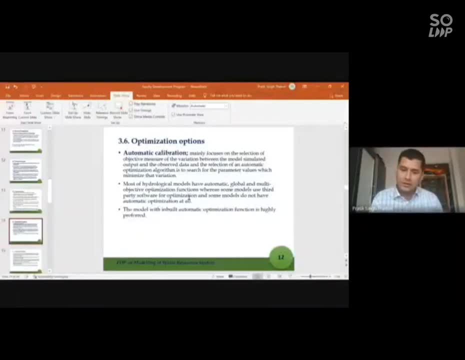 try to minimize the variation of those. try to minimize the variation of those with the selection of the automatic. with the selection of the automatic. with the selection of the automatic optimization algorithm. the process of optimization algorithm. the process of optimization algorithm. the process of automatic optimization algorithm. automatic optimization algorithm. 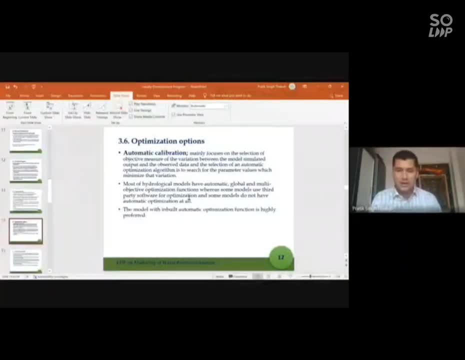 automatic optimization algorithm. so most of the ideological model do so. most of the ideological model do so. most of the ideological model do have automatic, have automatic, have automatic optimization, but not only automatic. they optimization, but not only automatic. they optimization, but not only automatic. they go for global and multi objective. go for global and multi objective. go for global and multi objective optimization function, optimization function. optimization function where some models have third-party, where some models have third-party, where some models have third-party software for optimization and some model software for optimization and some model software for optimization and some model do not have automatic optimization model. 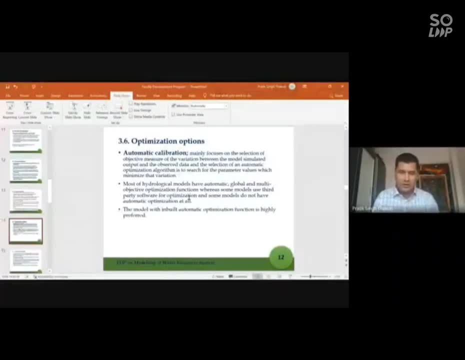 do not have automatic optimization model. do not have automatic optimization model, so so so what is the preference of the modeler? what is the preference of the modeler? what is the preference of the modeler if they would like to go for a global? if they would like to go for a global? 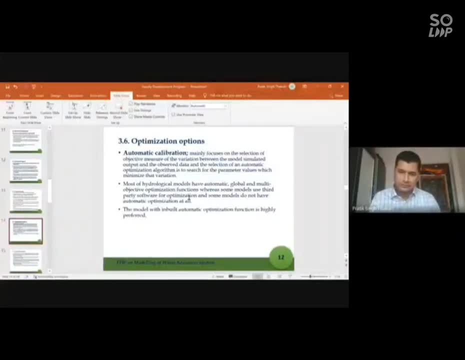 if they would like to go for a global optimization process. optimization process, optimization process. uh or uh, you know have. uh or uh. you know have. uh or uh. you know have need automatic optimization. uh need automatic optimization. uh need automatic optimization uh method. in the hydrological model, the 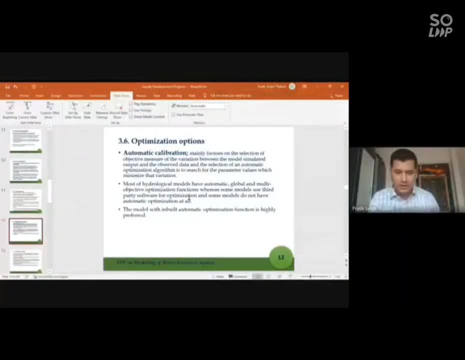 method in the hydrological model, the method in the hydrological model, the biological, biological, biological processes, then processes, then processes. then the modelers would go for the automatic, the modelers would go for the automatic. the modelers would go for the automatic calibration models, automatic models. 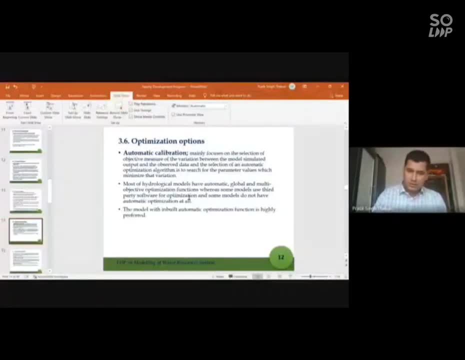 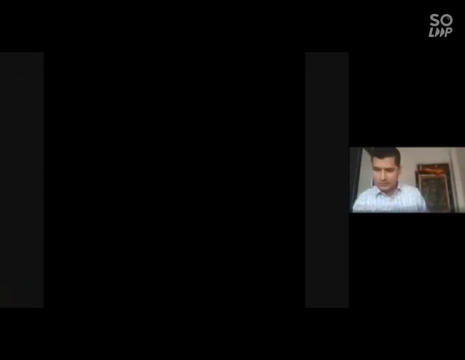 calibration models- automatic models. calibration models, automatic models which have automatic optimization options, which have automatic optimization options, which have automatic optimization options, so, so, so, yeah, so, so it is like i have been talking for a. so it is like i have been talking for a, so it is like i have been talking for a long, so i'll just like to throw a. 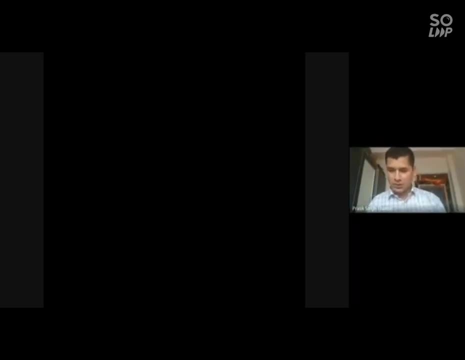 long, so i'll just like to throw a long. so i'll just like to throw a question to um. question to um. question to um the participant if they know about uh the participant. if they know about uh the participant if they know about uh global optimization and the. global optimization and the global optimization and the local optimization. the difference between local optimization, the difference between local optimization, the difference between global optimization and the global optimization, and the global optimization and the local optimization. anyone local optimization, anyone local optimization. anyone would like to answer this question? you? 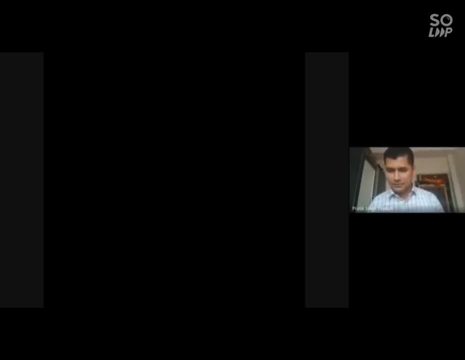 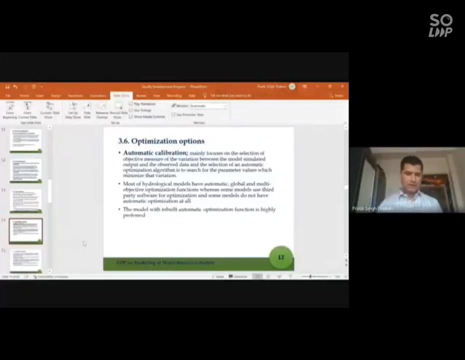 would like to answer this question. you would like to answer this question. you can just write it here. yes, i have just given a question, you can. yes, i have just given a question, you can. yes, i have just given a question. you can just write, just write, just write the difference between global. 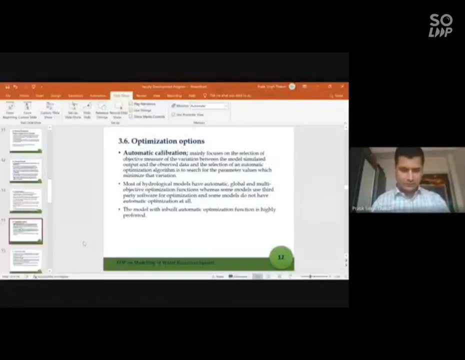 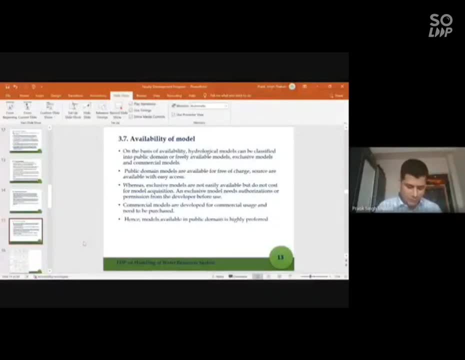 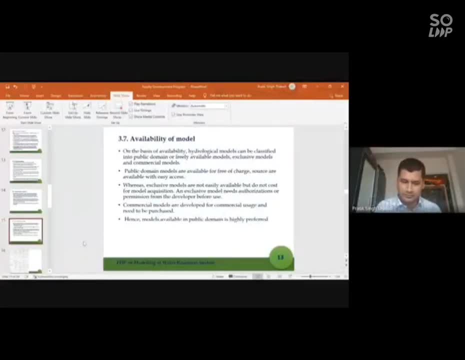 beginning of the beginning of the my presentation. if there are different, my presentation. if there are different, my presentation. if there are different type of type of type of model: um. some of the models are model um. some of the models are model um. some of the models are available in public domain, while some 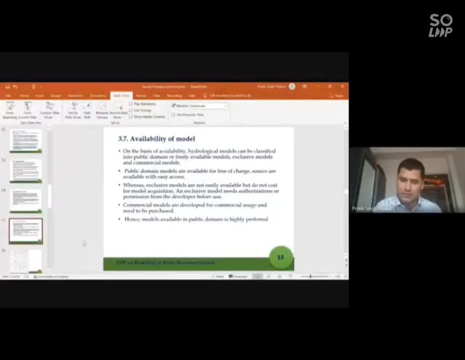 available in public domain, while some available in public domain, while some are exclusive and some are for the are exclusive and some are for the are exclusive and some are for the commercial purposes. so, on the basis of commercial purposes, so on the basis of commercial purposes, so on the basis of the availability, ideological model can be. 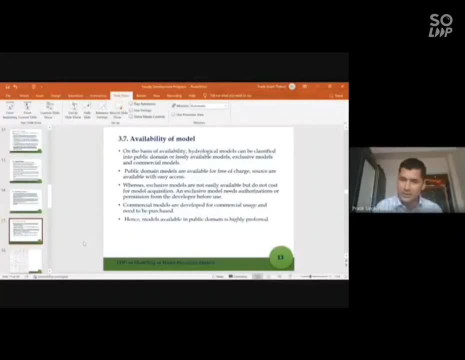 the availability ideological model can be. the availability ideological model can be classified into the public domain or classified into the public domain or classified into the public domain or freely available, freely available. freely available exclusive models or commercial market exclusive models or commercial market exclusive models or commercial market public domain models are available for. 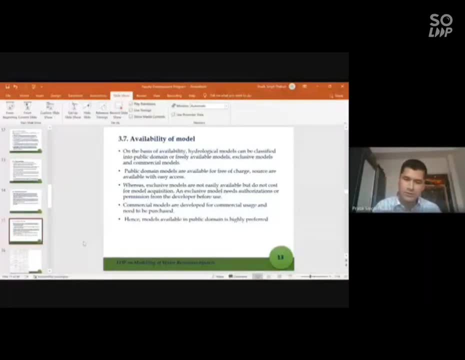 public domain models are available for public domain models are available for free of charge. source are available with free of charge source are available with free of charge. source are available with easy access, whereas exclusive models are easy access. whereas exclusive models are easy access, whereas exclusive models are not. 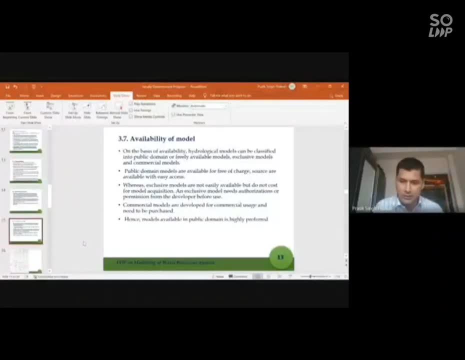 not not freely available, but uh, but they do not freely available, but uh, but they do not freely available, but uh, but they do not cost as well for model cost, as well for model cost as well for model acquisition: the exclusive model needs uh, acquisition: the exclusive model needs uh. 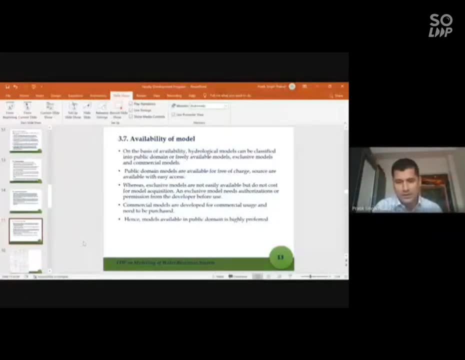 acquisition, the exclusive model needs uh authorization or permission from the authorization or permission from the authorization or permission from the developer before use. and similarly, they developer before use. and similarly, they developer before use. and similarly they are commercial models, are commercial models, are commercial models, and. and. and they are developed for commercial uses. 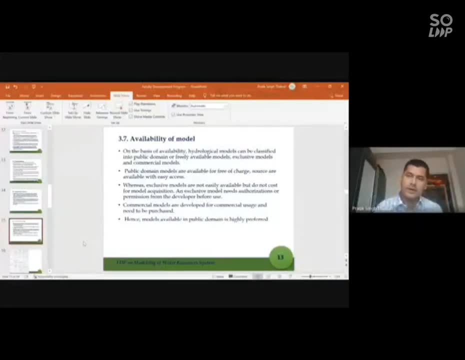 they are developed for commercial uses. they are developed for commercial uses and need to be purchased, so, and need to be purchased, so, and need to be purchased, so, uh, depending on the uh, depending on the uh, depending on the fund available, and depending on the fund available and depending on the 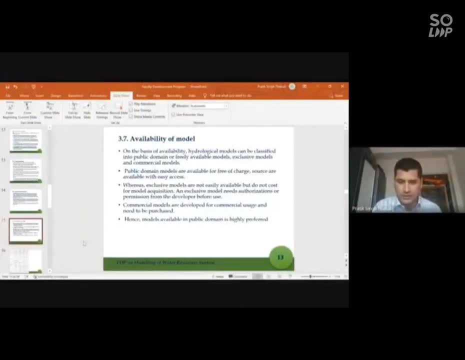 fund available and depending on the purpose of the study purpose of the study purpose of the study. you know the model should be selected. you know the model should be selected. you know the model should be selected based on the evaluative model as well, based on the evaluative model as well. 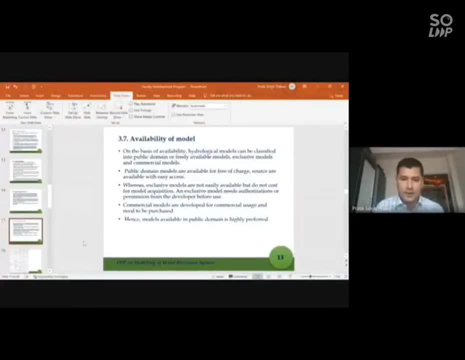 based on the evaluative model as well. so these were the seven criteria for, so these were the seven criteria for, so these were the seven criteria for model selection and, on these criteria, model selection, and on these criteria, model selection, and on these criteria, there are multiple factors as well, so 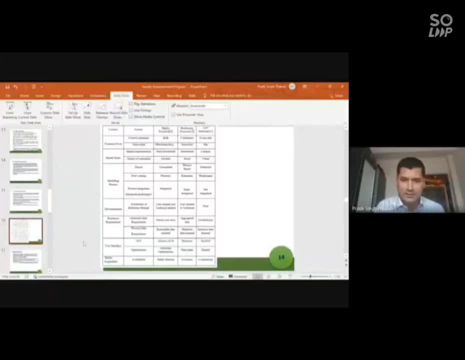 there are multiple factors as well, so there are multiple factors as well. so these were my, these were my, these were my, the criteria and factor and the, the criteria and factor and the, the criteria and factor and the preferences level, preferences level, preferences level for my study, and it was, it was a. 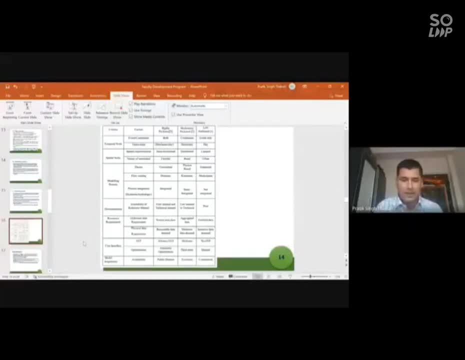 for my study and it was. it was a for my study and it was. it was a rural watershed in the rural watershed in the rural watershed in the hilly areas of sri lanka, hilly areas of sri lanka, hilly areas of sri lanka, where i conducted this study. so 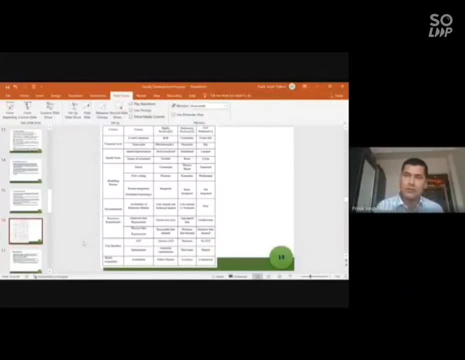 where i conducted this study. so where i conducted this study. so i, i was, i, i was, i, i was not having a, not having a, not having a fund to collect the or purchase the fund to collect the, or purchase the fund to collect the or purchase the ideological model. so 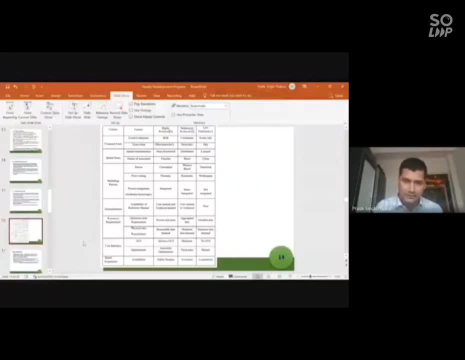 ideological model. so ideological model. so, depending upon my requirement, depending upon my requirement, depending upon my requirement, i have classified, i have classified, i have classified models and sort out my criteria, then models, and sort out my criteria, then models and sort out my criteria, then factors, and given the preferences from: 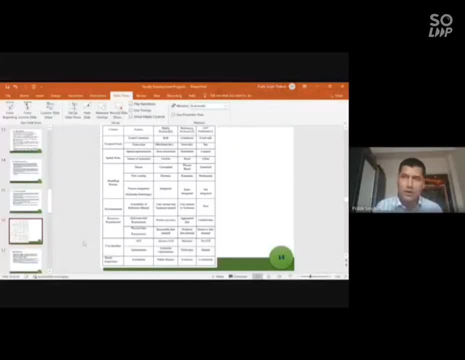 factors and given the preferences from factors and given the preferences from high to high to high to low, likewise, low, likewise, low, likewise any model. can you know any model? can you know any model? can you know? give the you know preferences and sort. give the you know preferences and sort. 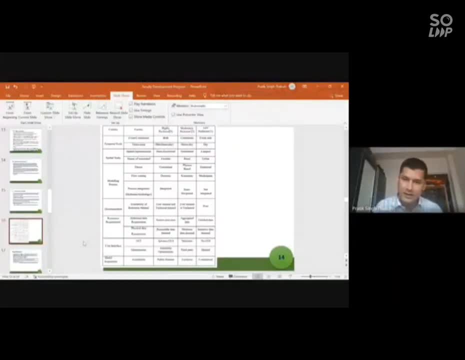 give the you know preferences and sort of their character criteria and multiple of their character criteria and multiple of their character character criteria and multiple factors and give their preferences factors and give their preferences factors and give their preferences and um choose a suitable and um choose a suitable. 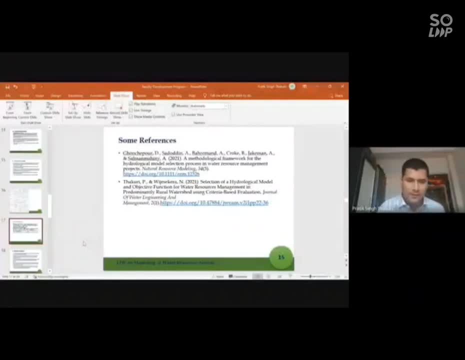 and um choose a suitable ideological model. so now i'm ideological model, so now i'm ideological model, so now i'm end of the first segment of my end of the first segment of my end of the first segment of my presentation and presentation and presentation. and that was how ideological model should. 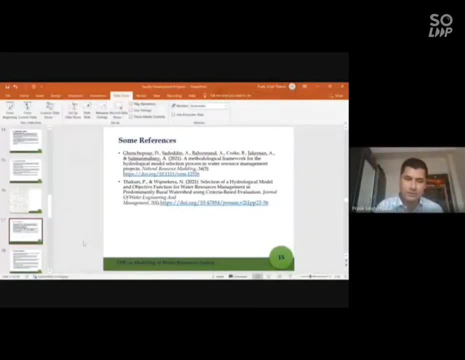 that was how ideological model should, that was how ideological model should be be be selected based on the criteria evaluation, selected based on the criteria evaluation, selected based on the criteria evaluation. you know, you know, you know, you can, first, you know, select the. you can first, you know, select the. 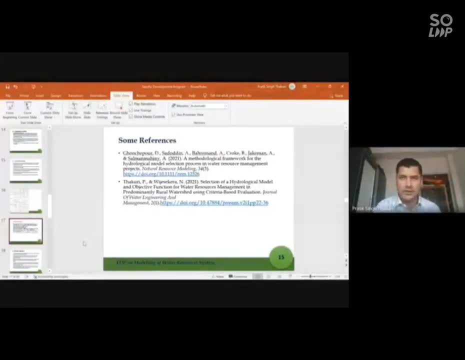 you can, first, you know, select the criteria and their factors, and you know criteria and their factors and you know criteria and their factors and you know, give the preferences label, give the preferences label, give the preferences label, assign their values and assign their values, and assign their values and or assign the weighted values and get a. 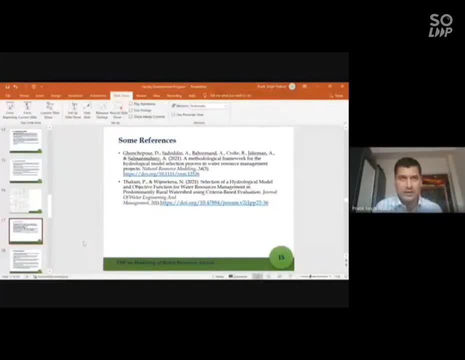 or assign the weighted values and get a, or assign the weighted values and get a. final, final, final. you know result, so i i'm citing here you know result, so i i'm citing here you know result, so i i'm citing here two literature um. two literature um. 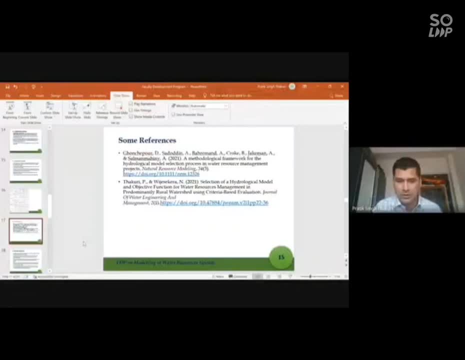 two literature, um, and the one is in the uh natural and the one is in the uh natural and the one is in the uh natural: resource modeling and the? the paper is a resource modeling and the? the paper is a resource modeling, and the? the paper is a methodological framework for hydrological 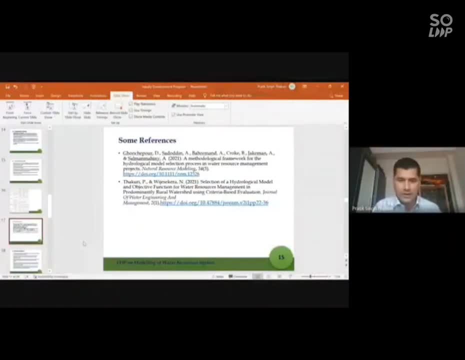 methodological framework for hydrological methodological framework for hydrological model selection, model selection, model selection process in water resources management process, in water resources management process, in water resources management project, project, project, uh this, this uh research, also uh this this uh research, also uh this this uh research. also give a framework, a methodological frame. 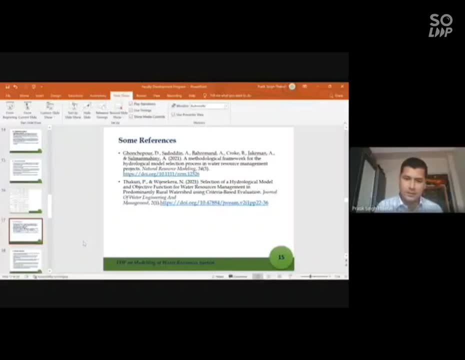 give a framework, a methodological frame, give a framework, a methodological frame of how hydrological models should be, of how hydrological models should be, of how hydrological models should be selected, selected, selected. um for a modeling study. similarly, um for a modeling study. similarly, um for a modeling study. similarly. the another literature is uh written. 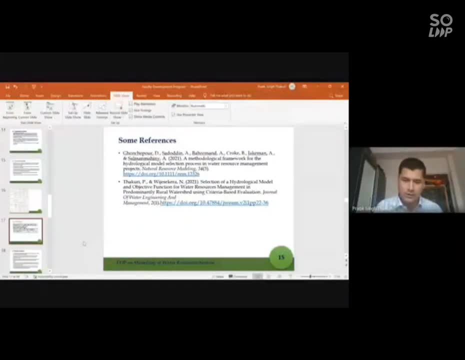 the another literature is uh written. the another literature is uh written. the paper was written by me. the paper was written by me, the paper was written by me and it published in journal of water and it published in journal of water and it published in journal of water: engineering and management. 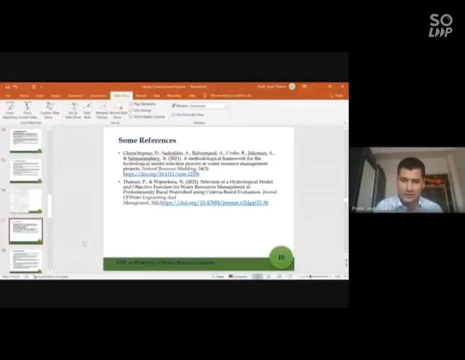 engineering and management. engineering and management, and it is on this the process of, and it is on this the process of, and it is on this the process of selection of hydrological model and selection of hydrological model and selection of hydrological model and objective function for water resources. 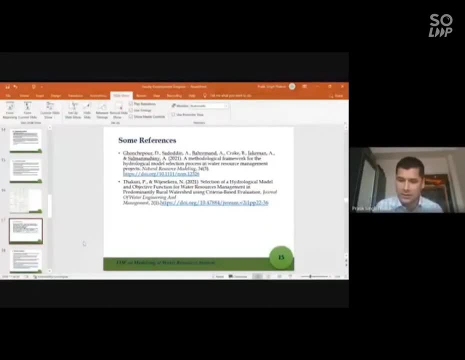 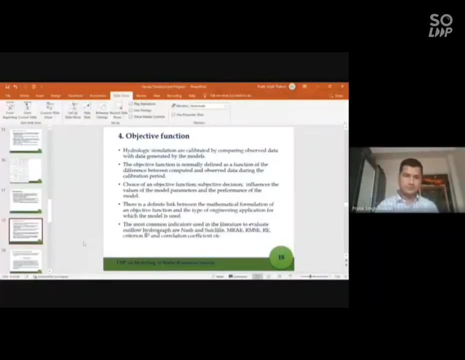 objective function for water resources: objective function for water resources management and the management and the management and the ruler areas using criteria: evolution ruler areas using criteria: evolution ruler areas using criteria: evolution criteria: best evaluation. yeah, now we'll head towards uh the another. now we'll head towards uh the another. 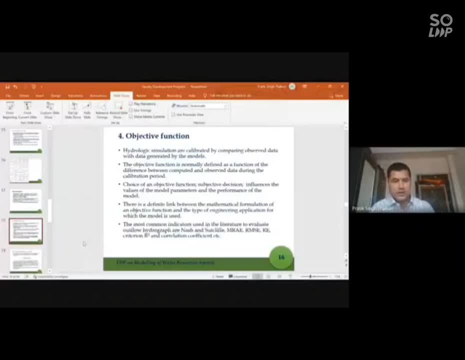 now we'll head towards, uh, the another segment of the presentation that would be segment of the presentation, that would be segment of the presentation, that would be in the objective function. this is also an in the objective function. this is also an in the objective function. this is also an important. 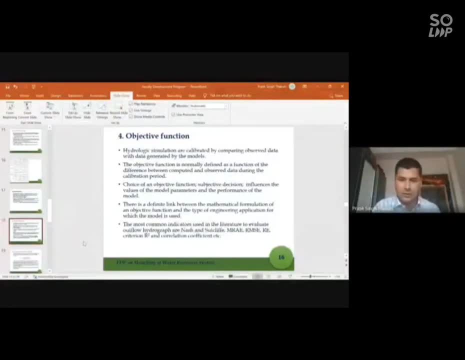 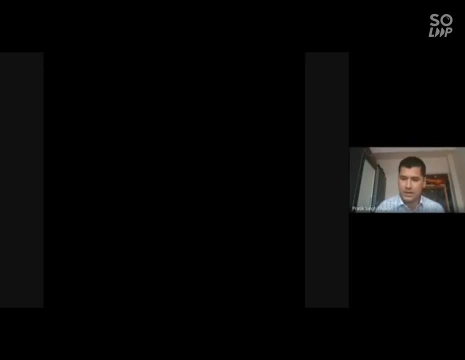 important, important factor to be considered, factor to be considered, factor to be considered in hydrological modeling, so in hydrological modeling, so in hydrological modeling. so yes, yes, yes. anyone would like to answer what is? anyone would like to answer what is? anyone would like to answer what is objective function? 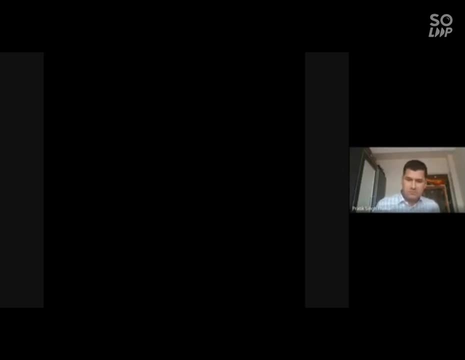 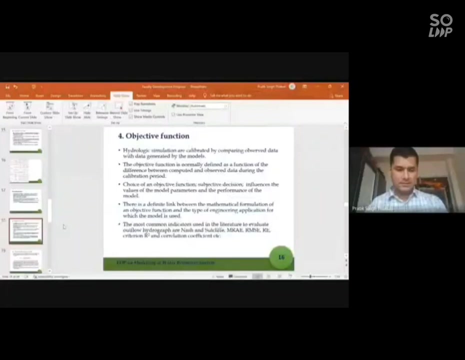 and what is the use of objective function and what is the use of objective function and what is the use of objective function. you can just write it, okay: so yes, so yes, so yes, is my slide visible? so yes, is my slide visible? so yes, is my slide visible? yes, yes, 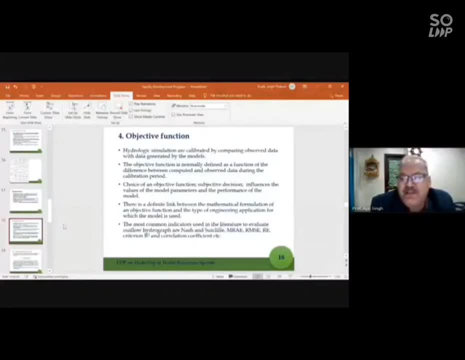 yes, yes, yes, yes. so what is the, the local optima and the? so what is the, the local optima and the? so what is the, the local optima and the global optima? please explain as a layman: global optima and the global optima. please explain as a layman. 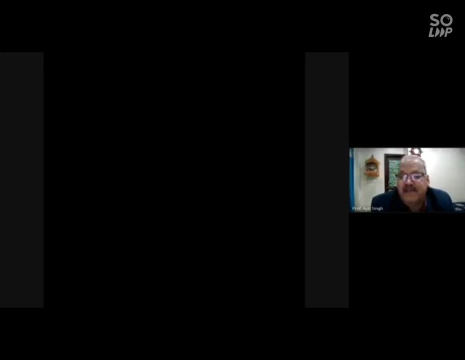 global optima and the global optima. please explain as a layman: local optima and global optimize. if you local optima and global optimize. if you local optima and global optimize. if you have any idea, have any idea, have any idea? okay, so the local optima is, uh like. 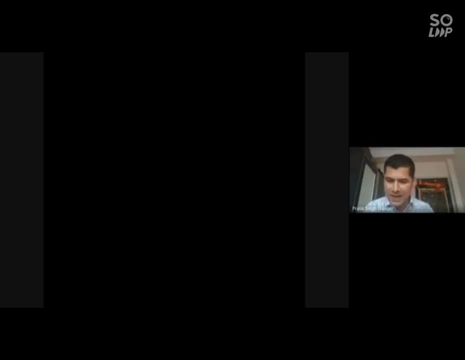 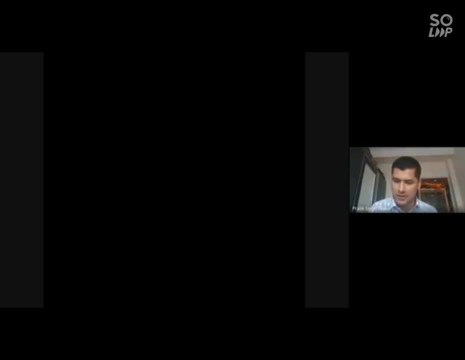 you know, try to optimize that parameter. and you know, try to optimize that parameter and look for, look for, look for the, the, the objective function of the objective function, of the objective function of the model. and once you reach into the model, and once you reach into the, 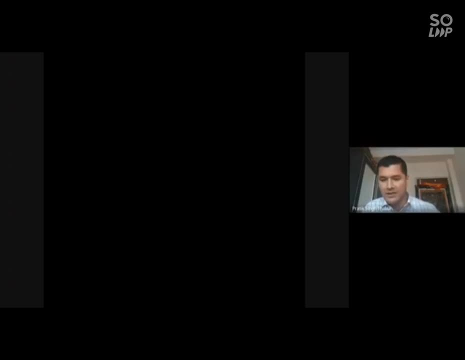 model, and once you reach into the optimum label, then you just leave optimum label, then you just leave optimum label, then you just leave and go for another parameter for and go for another parameter for and go for another parameter for. so means uh local. so means uh, local. 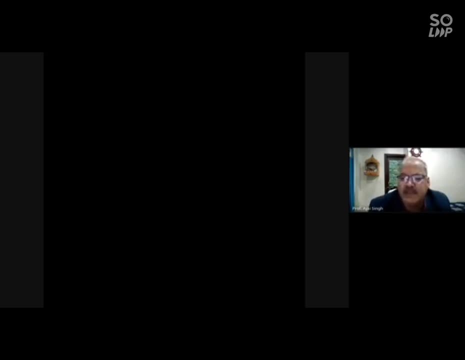 so means uh, local, that local variable, or the that local variable, or the that local variable, or the parameter that may be the infiltration parameter, that may be the infiltration parameter, that may be the infiltration rate. yeah rate, yeah rate, yeah. and the objective function may be r and the objective function may be r. 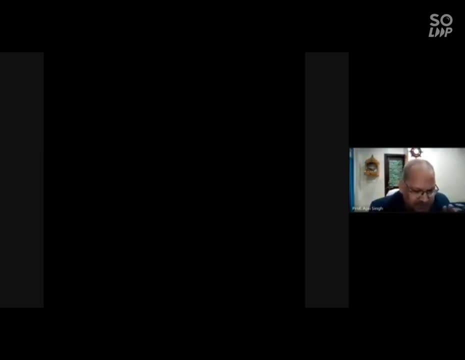 and the objective function may be r, square or nse. yeah, okay, so. square or nse? yeah, okay, so, square or nse? yeah, okay, so. infiltration rate will be optimized to. infiltration rate will be optimized to. infiltration rate will be optimized to get the appropriate value of nse. 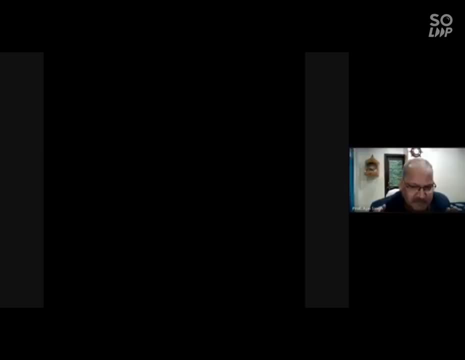 get the appropriate value of nse. get the appropriate value of nse. the objective function: yeah, one at a the objective function: yeah, one at a the objective function: yeah, one at a time and then one at a time. yeah, then time and then one at a time, yeah then. 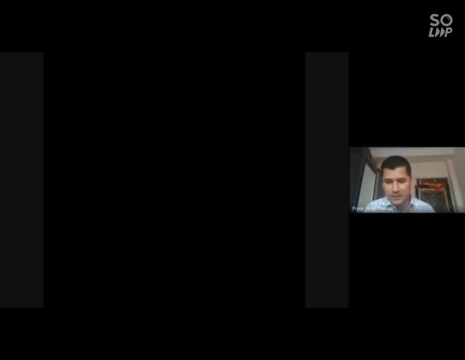 time and then one at a time, yeah, then you just move to another, and at that you just move to another, and at that you just move to another, and at that time you know the time, you know the time, you know the the. the nse may go up or or low. 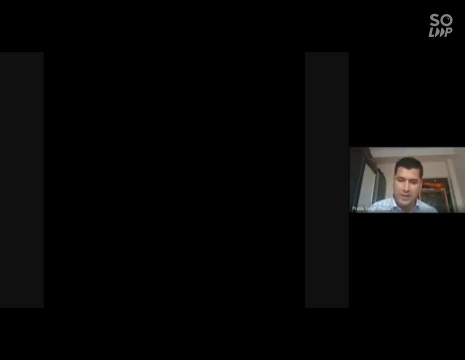 the the nse may go up or or low, the the nse may go up or or low, uh, and they did this, the uh, the uh, and they did this, the uh, the uh, and they did this, the uh. the optimization you have done in the the. 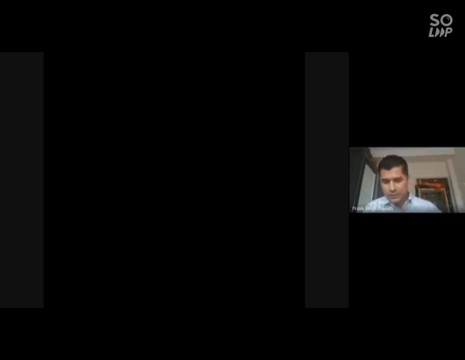 optimization you have done in the, the optimization you have done in the: the infiltration um, infiltration um, infiltration um, would be, wouldn't be, would be, wouldn't be, would be, wouldn't be done again. but in the global um, done again. but in the global um, done again. but in the global um optimization, you, you look for all the. 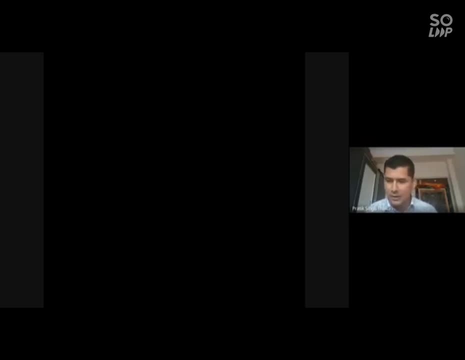 optimization. you, you look for all the optimization, you, you look for all the parameter at parameter, at parameter, at one at a time and one at a time and one at a time, and look for, look for, look for a compromised optimization, and you, you a compromised optimization and you you. 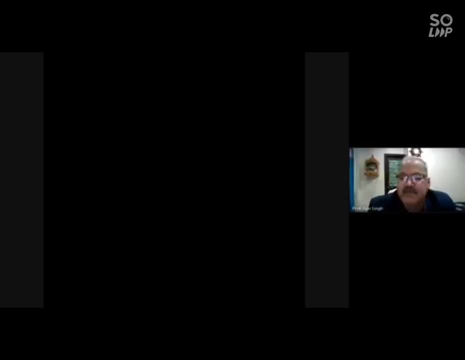 a compromised optimization and you, you get a set of compromised parameters, get a set of compromised parameters, get a set of compromised parameters compensating one to another, compensating one to another, compensating one to another. yes, yeah, i got it. yes, yeah, i got it. yes, yeah, i got it. um, since we are discussing, let me read a. 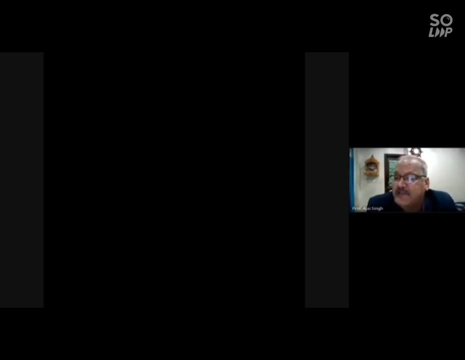 um, since we are discussing, let me read a? um since we are discussing, let me read a question from the bias. he is asking: why question from the bias? he is asking why question from the bias? he is asking why urban special skill model is less? urban special skill model is less. 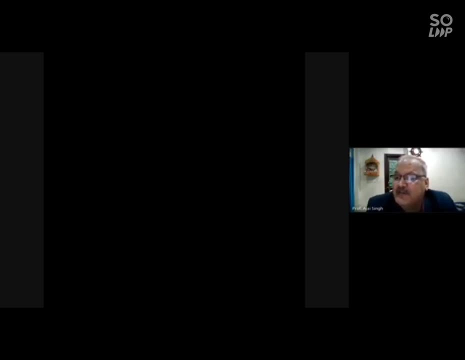 urban special skill model is less preferred, preferred, preferred. urban special model. urban special model. urban special model, special skill model, special skill model, special skill model. okay, okay, okay, yeah, so it's not less preferred or highly. yeah, so it's not less preferred or highly. yeah, so it's not less preferred or highly preferred. if if. 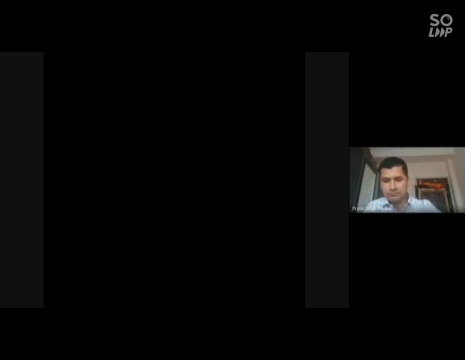 preferred if, if preferred if. if you want um a model to be, you know you want um a model to be. you know if you are, if you have a um, you are. if you have a um, you are. if you have a um research study or case study to be. 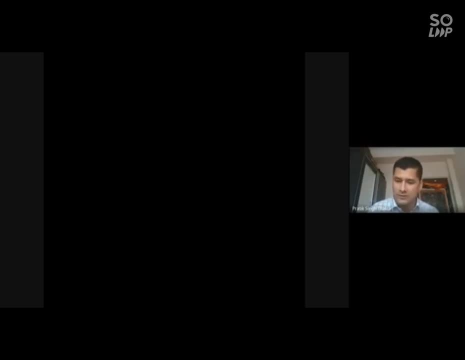 research study or case study to be research study or case study to be conducted in the urban uh watershed, conducted in the urban uh watershed, conducted in the urban uh watershed? uh, then you'll definitely go for you know. uh, then you'll definitely go for you know. uh, then you'll definitely go for you know the model, like the stormwater. 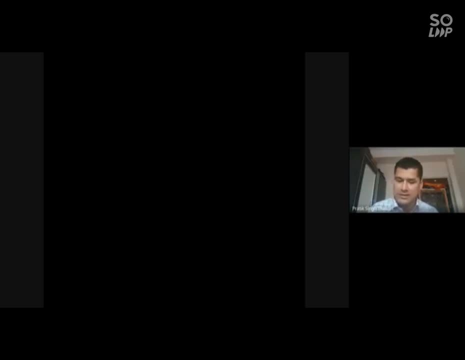 the model like the stormwater, the model like the stormwater management model, or you can say swmn management model, or you can say swmn management model, or you can say swmn, and that is especially designed for and that is especially designed for and that is especially designed for urban watershed. so, depending upon the 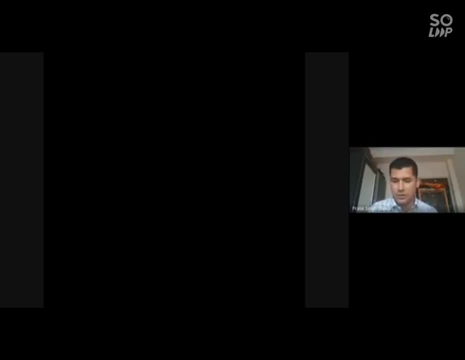 urban watershed. so, depending upon the urban watershed, so depending upon the the purpose of your study, the purpose of your study, the purpose of your study, um, you go for um the model selection, um you go for um the model selection, um, you go for um the model selection, it's not. 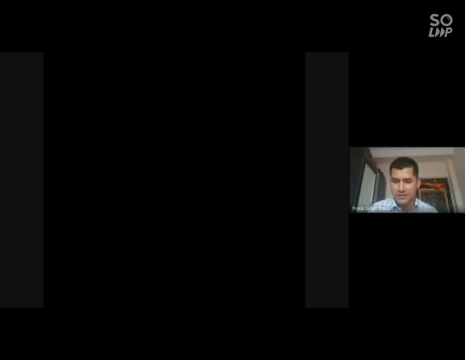 it's not. it's not less preferred or highly preferred. it's less preferred or highly preferred. it's less preferred or highly preferred. it's always about the rational selection, or always about the rational selection, or always about the rational selection, or rational decision on the rational decision on the. 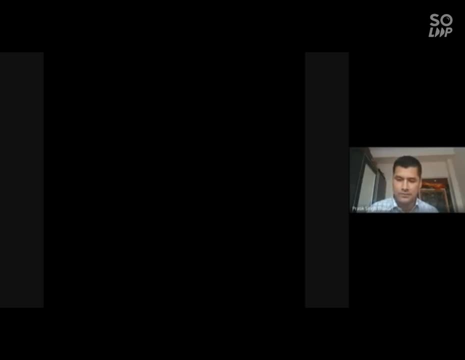 rational decision on the selection of the model. any example of urban special skill model. any example of urban special skill model, any example of urban special skill model. you know, i don't know any model which is which is. i don't know any model which is which is. 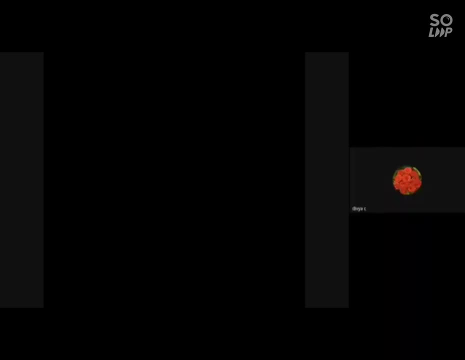 i don't know any model which is which is named by, named by, named by this term. yes, uh, so actually in the this term. yes, uh, so actually in the this term. yes, uh, so actually in the criteria. sir has listed there, he listed criteria. sir has listed there, he listed. 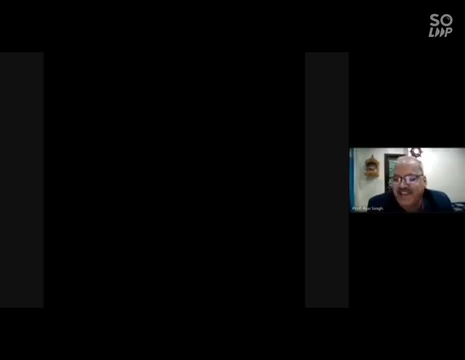 criteria sir has listed there. he listed like the spatial urban spatial model is like the spatial urban spatial model is like the spatial urban spatial model: is less preferred, less preferred, less preferred. oh okay, yeah, okay. so now, now you please go ahead, yeah, okay. another thing, another aspect of the 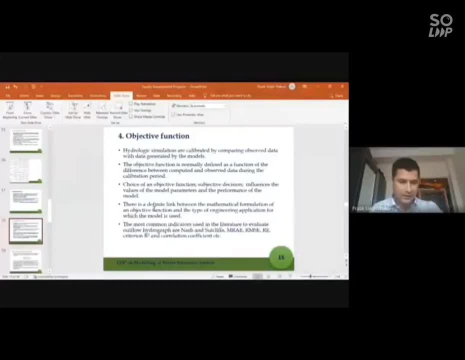 another thing, another aspect of the another thing, another aspect of the hydrological model. that hydrological model, that hydrological model, that uh, uh, should be, uh, should be, uh, should be in the hydrological modeling, should be in the hydrological modeling, should be in the hydrological modeling, should be considered, is the objective function. so 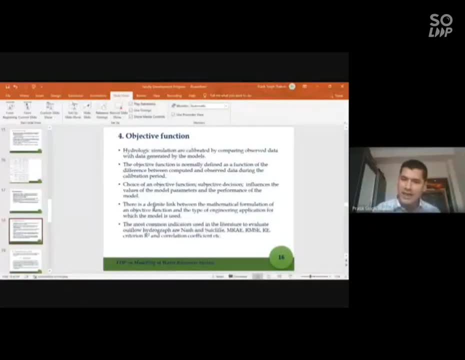 considered is the objective function. so, considered is the objective function. so, uh, what is objective function? uh, uh, what is objective function? uh, uh, what is objective function? uh, hydrological simulations are calibrated. hydrological simulations are calibrated. hydrological simulations are calibrated by comparing observed data set with a. 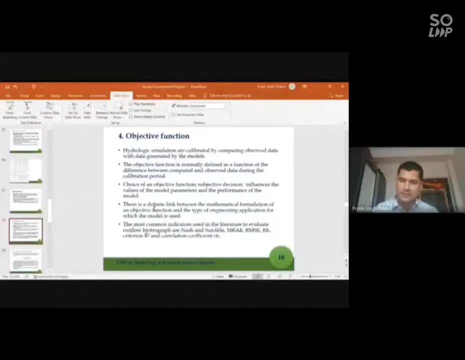 by comparing observed data set with a, by comparing observed data set with a data generator model and the objective data generator model and the objective data generator model and the objective function is function is function is you know the function of difference? you know the function of difference? you know the function of difference between computed and the observed data? 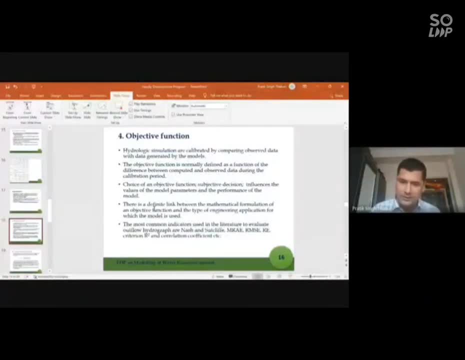 between computed and the observed data, between computed and the observed data set during the calibration of model set during the calibration of model set during the calibration of model. so the choice of objective function is so, the choice of objective function is so. the choice of objective function is also another subjective. this 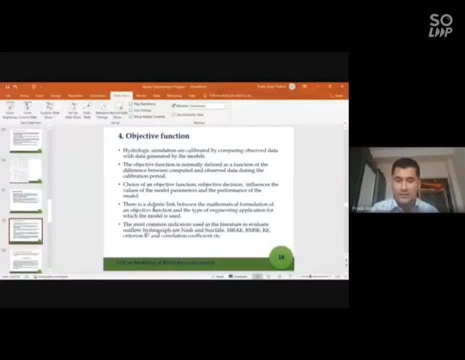 also another subjective. this also another subjective, this decision, and that influences the value decision and that influences the value decision and that influences the value of parameters and the performance of of parameters and the performance of of parameters and the performance of model so, model so, model, so the selection of objective function. 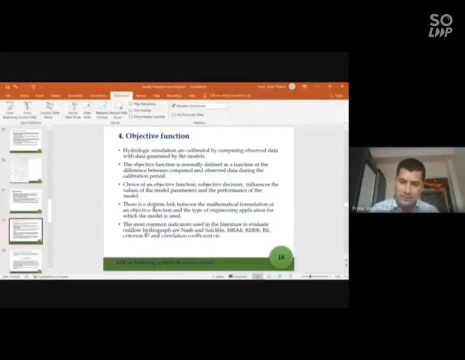 the selection of objective function. the selection of objective function should also be very rational and that should also be very rational, and that should also be very rational and that would you know, would you know, would you know really influence the model parameters and really influence the model parameters and 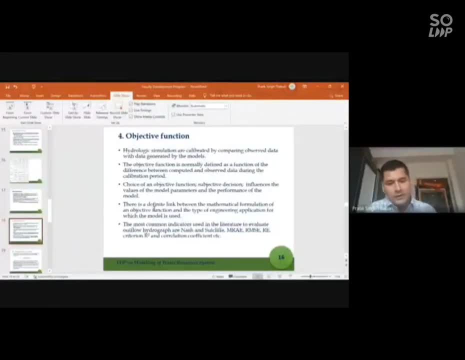 really influence the model parameters and performance of the model, performance of the model, performance of the model. so there is a definite link between. so there is a definite link between. so there is a definite link between mathematical formulation and an mathematical formulation and an mathematical formulation and an objective function and the type of 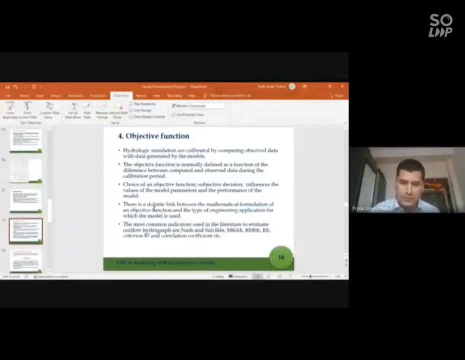 objective function and the type of objective function and the type of engineering application, which engineering application, which engineering application, which which the model is used. so, uh, you know which the model is used. so, uh, you know which the model is used. so, uh, you know, objective functions are different there. 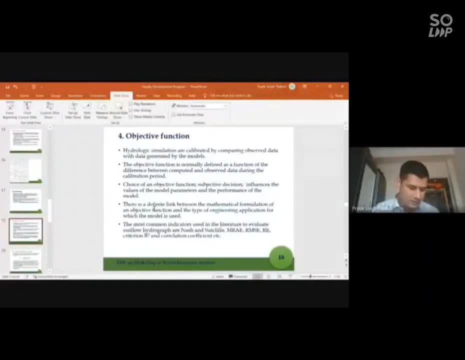 objective functions are different. there, objective functions are different. there are a lot of objective functions. there are a lot of objective functions. there are a lot of objective functions. there are a lot of efficiency criteria. are a lot of efficiency criteria? are a lot of efficiency criteria available? but 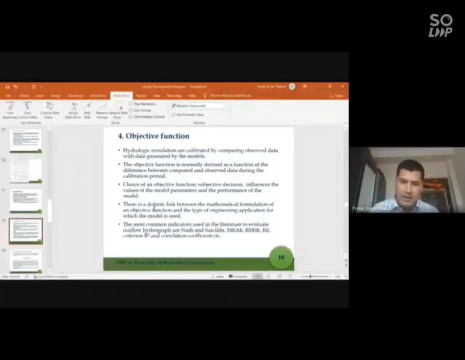 available, but available. but all of them has some mathematical, all of them has some mathematical, all of them has some mathematical function, function, function, and that mathematical function is and that mathematical function is and that mathematical function is associated with you know, and that mathematical function is associated with, you know, with some engineering application. so 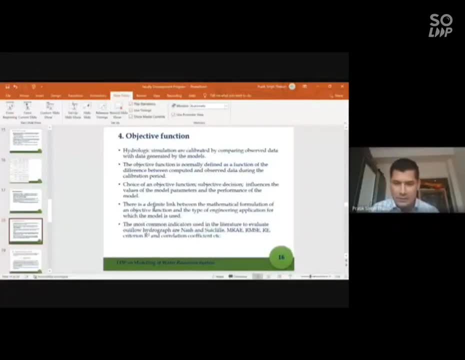 associated with, you know, with some engineering application. so associated with, you know, with some engineering application. so you have to, you have to, you know, you have to, you have to, you know, you have to, you have to, you know, find the link between the mathematical, find the link between the mathematical. 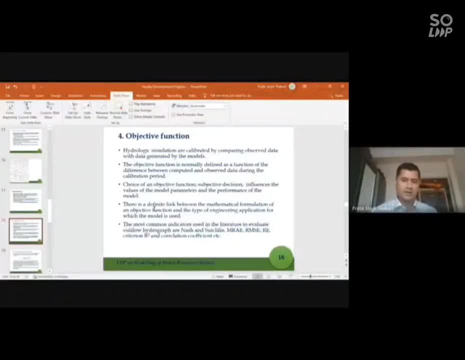 find the link between the mathematical formulation and of the objective formulation, and of the objective formulation and of the objective function, and the type of engineering function and the type of engineering function and the type of engineering application, that application, that application that could be, you know, used so the most. 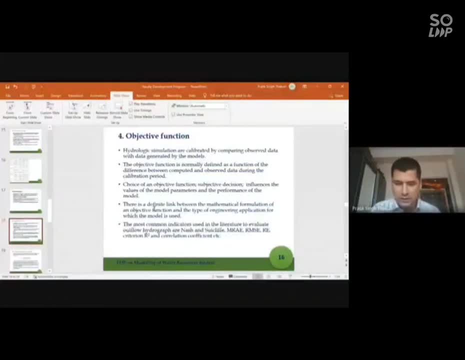 could be, you know, used. so the most could be, you know, used. so the most common indicators are the goodness of common indicators, are the goodness of common indicators, are the goodness of feet also. they call feet also, they call feet also. they call objective function in the literature, uh. 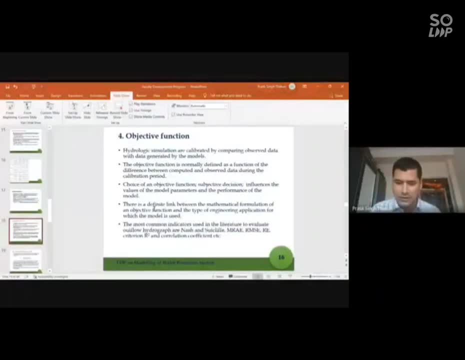 objective function in the literature: uh, objective function in the literature: uh, to evaluate flow hydrograph. are you know to evaluate flow hydrograph? are you know to evaluate flow hydrograph? are you know mass subtlety, or mass subtlety or mass subtlety or mean? ratio of absolute error? root mean. 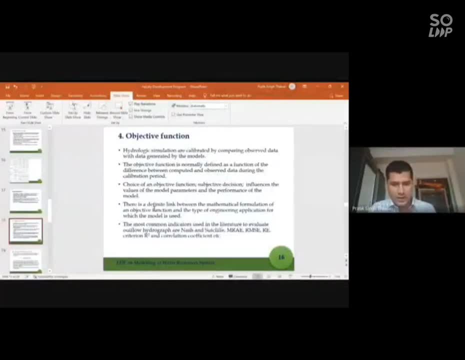 mean ratio of absolute error root. mean mean ratio of absolute error root, mean square error. uh, you know relative error, square error. uh, you know relative error, square error. uh, you know relative error, something like r square or coefficient. something like r square or coefficient, something like r square or coefficient. variation, coefficient correlation. 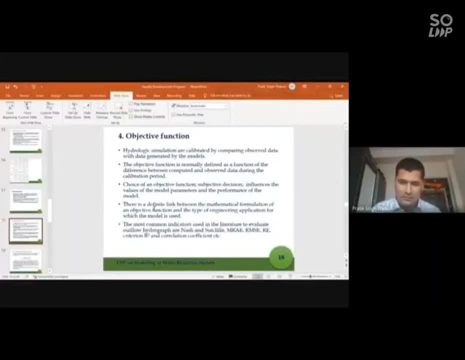 variation, coefficient, correlation, variation, coefficient, correlation, coefficient. so there are coefficient, so there are coefficient. so there are four or five i have listed here, but four or five i have listed here, but four or five i have listed here. but there are multiple, you know there are. there are multiple, you know there are. 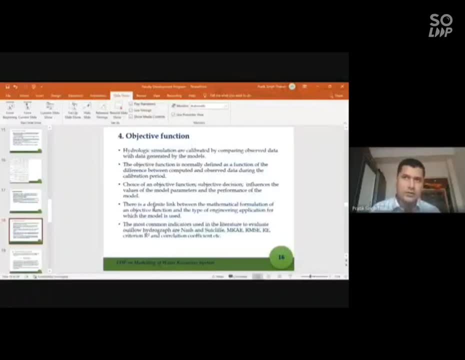 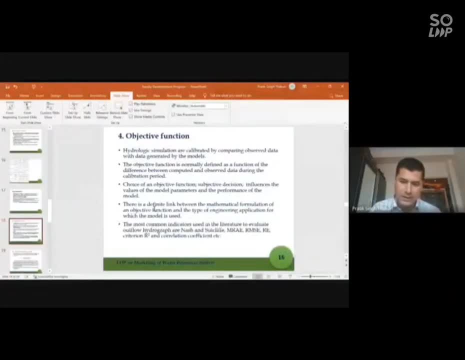 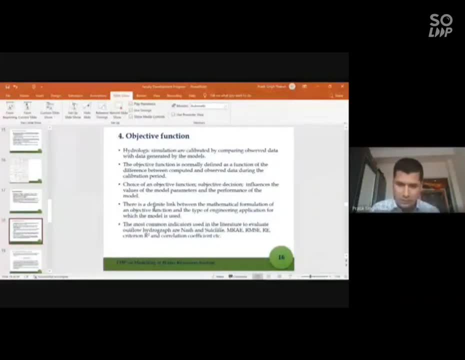 this study. so, likewise, you, you can, you know, exclude other objective functions or other goodness of it. so it's not necessary. you, really, you have to have a lot of objective functions and go for a multi-objective- um, you know, optimization. uh, if your purpose of the study, 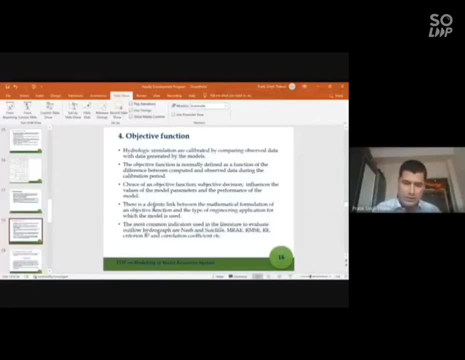 is clear and what you are aiming for, then you can go just for a one or two objective function to have, you know, uh, for to have a better calibration or better optimization of the model. so yeah, i've just told a few examples of an objective function. i'll know i'll not go very deep into all these. 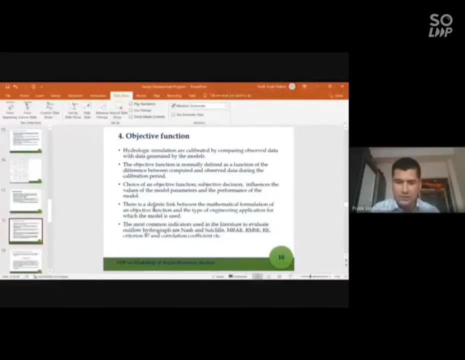 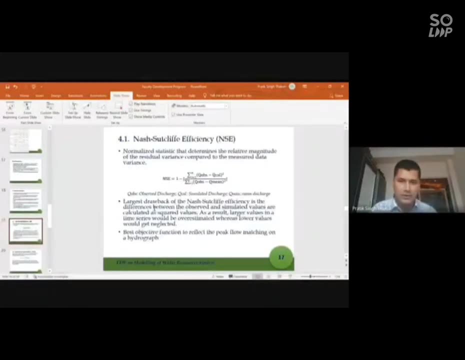 objective function, their mathematical formulation. but i'll briefly go in the few of this objective function, like nash short cliffs and mra. so nash short cliff is one of the objects function that is being popularly used, uh for optimizing the model parameter. so these are normal normalized statistics. um that determines relative magnitude of residual variance. 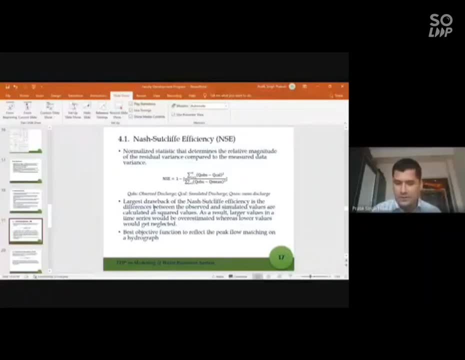 compared to the measured variance. so variance that object: um digital observed this child minus calculated distance, uh squared is the variance. so this is just a mathematical formulation of this um natural efficiency, but you know you have to um if you go deep into national it has a largest uh drawback is that the difference between observed and simulated. 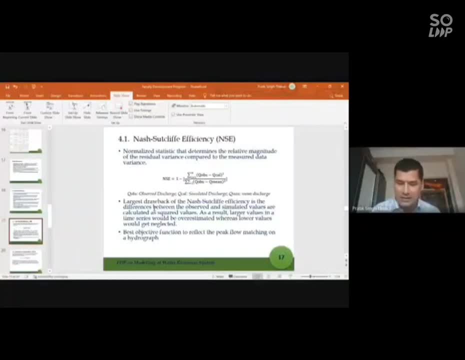 values are square values. as a result, larger values in the time series- you know, if you have a continuous date of eight years, the larger value are overestimated where lower values get neglected. so if the model is not performing in the, in the in the lower um uh data, or if model is not performing, 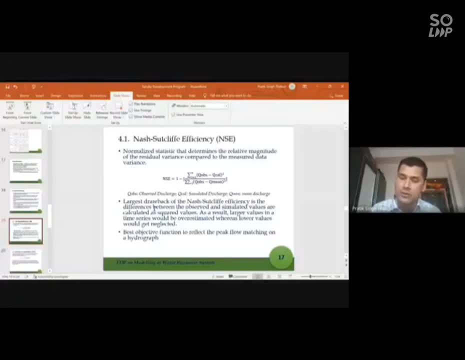 in the, even in the in the in the lower um uh data, or if model is not performing in the even in the, even in the in the in the lower um uh data, or if model is not performing in the even in the, even in the. you know the low flows or the intermediate flow region of the hydrograph uh, the, the nash. 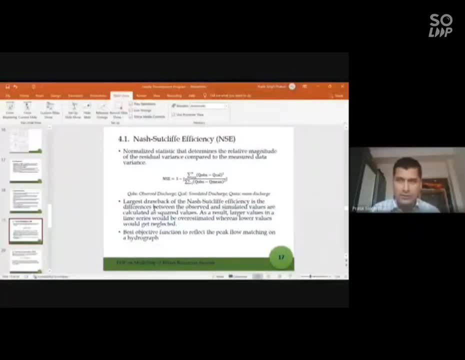 shot click can give a better result and that that would be a complete disguise. that, uh, the result is giving is showing a good. it is closer to one, it's like 80 efficiency or 90 efficiency, but, um, it is not giving a proper matching in low flows or intermediate flows. so if 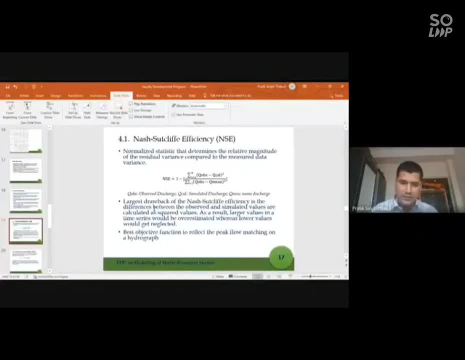 that is the largest uh drawback of national efficiency. so it's the best objective function to, but it is the best objective function to for peak flow matching. so having told that uh, i would say that nashville short leaf is a good uh efficiency criteria. goodness of fit or a goodness of fit for flood, hydrograph or flood. 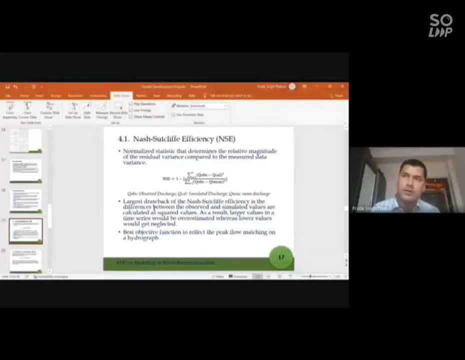 modeling purposes. if you, if you are trying to model for something like water, water resources or drought management case study, then you should rather go for other hydrological, other efficiency criteria, um than these uh, nash, short clip efficiency. so you have to, uh, you know properly, uh, uh, you know, go deep into the objective function, the mathematical formulation, do a deep. 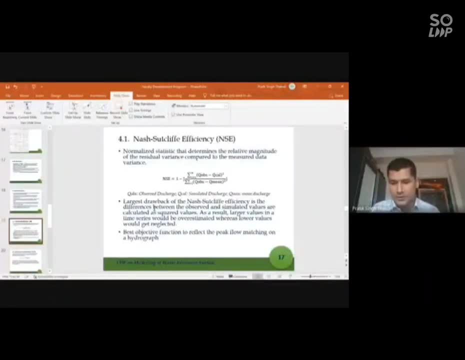 literature review before selecting the objective function of the uh for your study. the second thing, second objective function i'll be mentioning here, is mean ratio of absolute error. so the mean ratio of absolute error is the mean ratio of absolute error. so the mean ratio of absolute error is the. 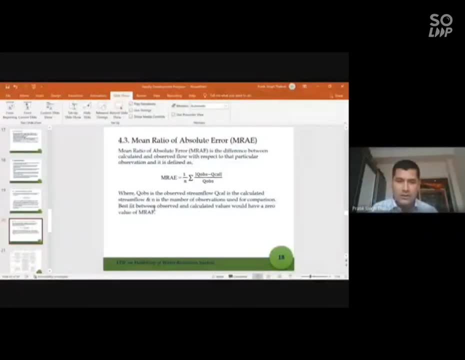 mean ratio of absolute error. so the mean ratio of absolute error is the mean ratio of absolute error. what happens is, you know the difference between observed and calculated discharge. um, you know, it is the ratio of the observed calculated discharge with respect to the observed one. so it's a mean ratio. is the difference between calculated and observed flow with respect to. 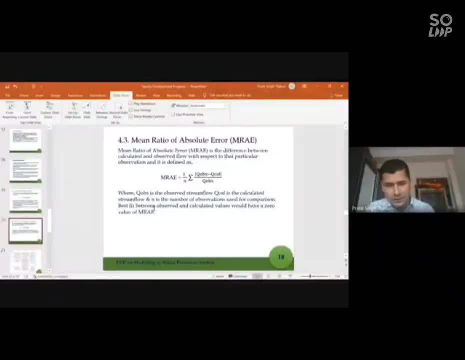 particular observation. so it gives a, you know um error. uh, with respect to each and every data set. it is in every point in the data set. so, um, but the thing is um, the best fit between uh, observed and distributed, observed and calculated value would be zero. uh value for mra. so, um, the thing is in the mra. if, if, um, if the observed value 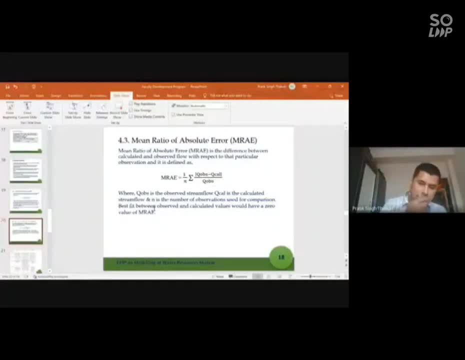 is zero, then it would be um invalid because it would be divided by the zero. so the measured drop back in the uh mean ratio of absolute error would be zero. so the measured drop back in the uh mean ratio of absolute error would be zero. so the measured drop back in the uh mean ratio of absolute. 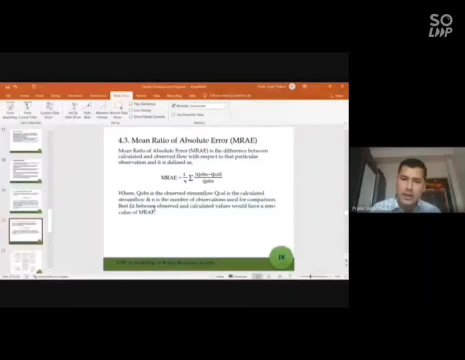 error is that if there is no flow condition in the uh hydrograph, then the uh, you. you should not select this uh mean ratio of accelerator. so you know, if you select the mean ratio of absolute error as an objective function, and uh, if there are no flow condition, then the, this, um, the, the, 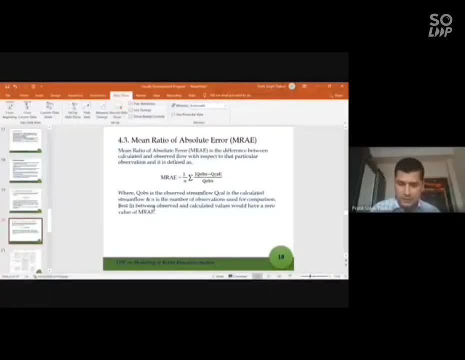 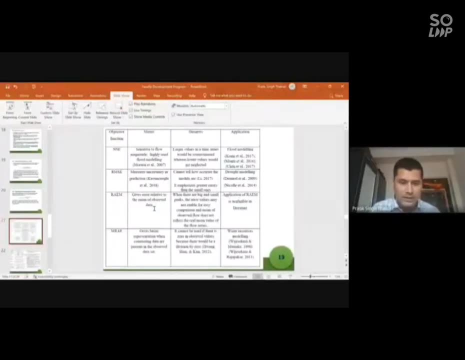 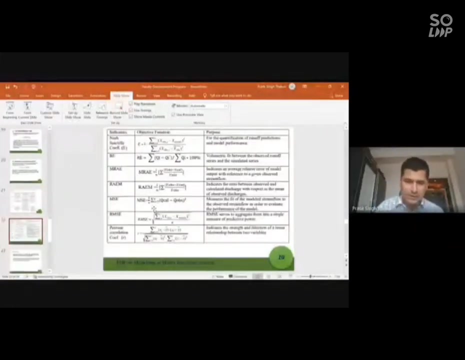 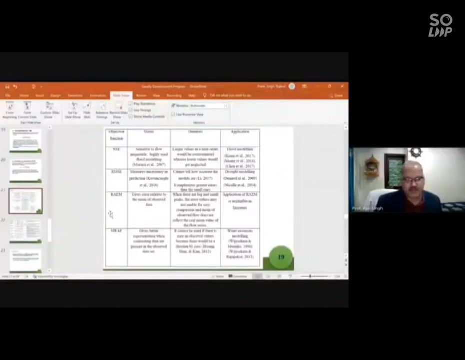 objective function would not keep a better result or it will go completely void. so, um so, i have, um uh, listed out the merits and demerits of few uh objective function and the purpose, as well, of those objective function. is my slide visible right now? yes, yes, you, you are clearly audible and slides are visible. yeah, please, please, go ahead, yeah, so. 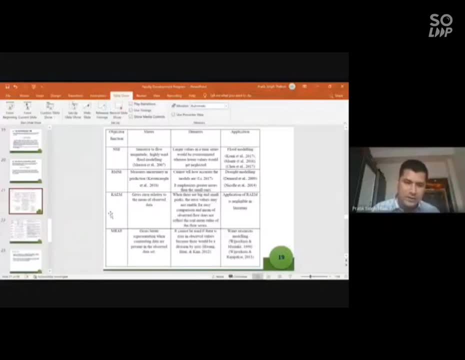 there are um i have listed um four. you know objective functions, so um those objective functions um are like natural cleaves and root mean square error or ratio of absolute error to mean and mean ratio of absolute error. so there are a lot of other objective function as well, but you have to um go deep inside the literature and the 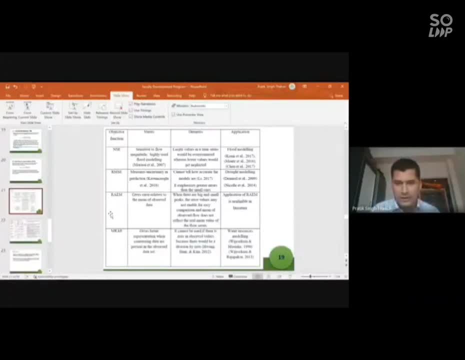 mathematical formulation, uh, before um selecting them for your study. so for root natural cliff, you know it's a sensitive to flow magnitude and highly used for flood modeling. so that is, uh the advantage: it is highly used for modeling and the demerit is the larger value in the time. 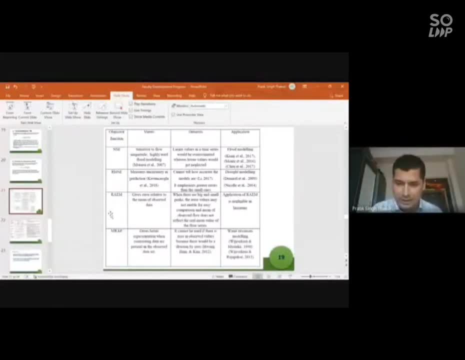 series would be over estimated, whereas lower value is neglected. so it is the application. it has been, you know, mainly used for flood modeling. similarly, you know, root mean square error. this, the merit, is the major uncertainty in the prediction, and the demerit is that cannot tell how accurate the model are. it infasses greater errors than the lower ones. so 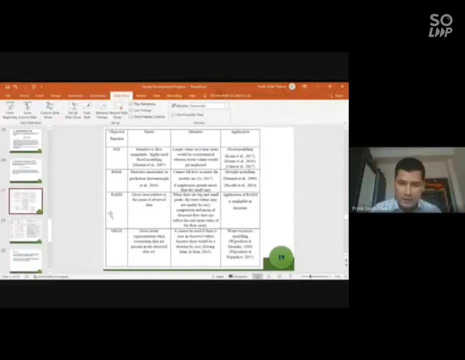 it increases in the more error. it's a the indicator of error. so it increases in the greater error and the less smaller errors in the model would be. you know, the neglected. so it is mainly chosen for the dot modeling. so similarly, the model on this objective function is the mean. 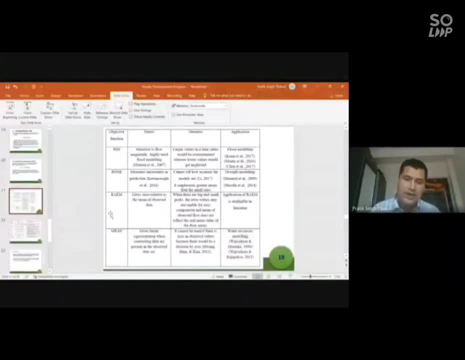 ratio of the absolute mra, which gives a better representation when contrasting data are present in the object data set. but uh, you know, the major demerit is it cannot be used if there are zero in the observed values, because there they would be divided by the zero. so water resource modeling, uh, 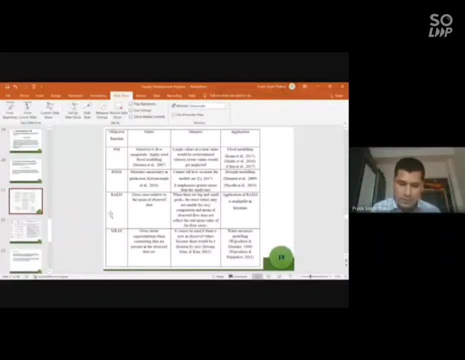 it is this. this model is heavily used for water resources modeling, namely like for the utility, proper purpose, if you would like to build a irrigation reservoir or something like that, or for a drinking water supply condition where the intermediate flow reasons are more important. in these cases, you know, the mean ratio of absolute error are selected. so the based on the purpose of 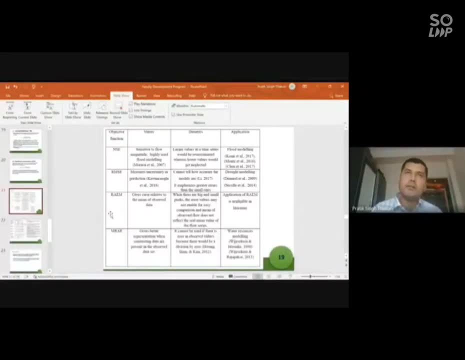 the system is the mean ratio of the absolute error. so the based on the purpose of the system is the mean ratio of the absolute error are selected. so the based on the purpose of the study, the based on the engineering application of the hydrological model, the objective function. 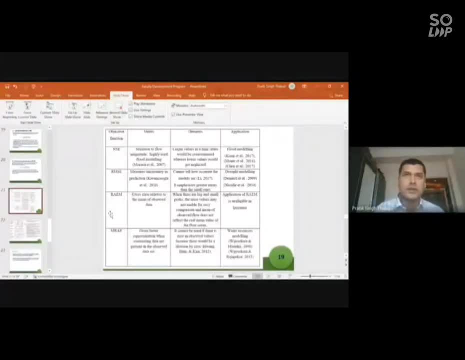 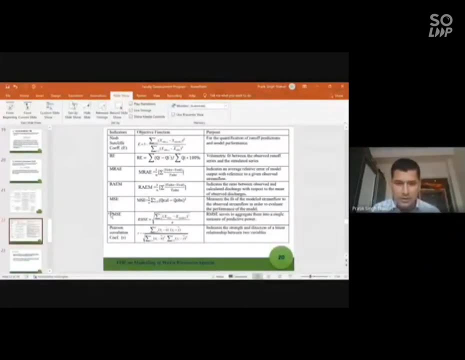 should be selected. as it name suggests, the objective should be the clear. so the other indicator you know. furthermore, with the pearson coefficient and um, you know, root mean square error. these i have listed all these model mathematical function and their purpose and you can just go through it later in this. 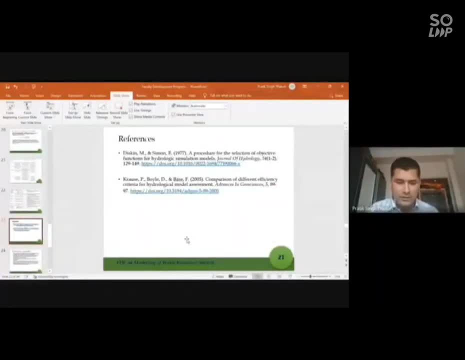 slide, so i'll be sharing uh two other references for selection of the hydrological model objective function in hydrological modeling, and that is the procedure for selecting um objective function for hydrological simulation model, and another is comparison of different efficiency criteria for hydrological model assessment. so this objective function is sometimes 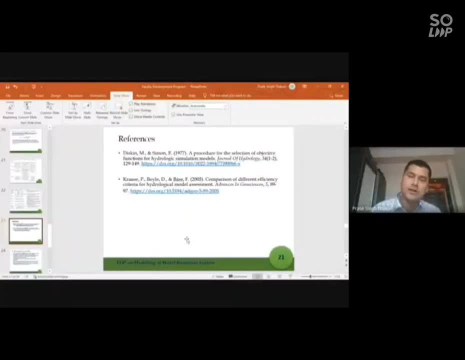 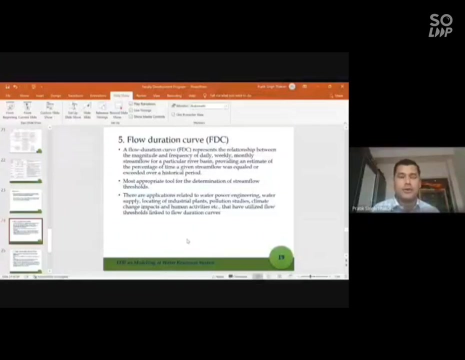 called objective function, efficiency criteria, goodness of feed or whatever. but the selection of these objective function or efficiency criteria, or goodness of food, should be rational and based on the engineering application. you are the purpose of the study you are supposed to carry out in your watershed. now the fifth uh domain i'm going to touch in this lecture is the flow duration curve. 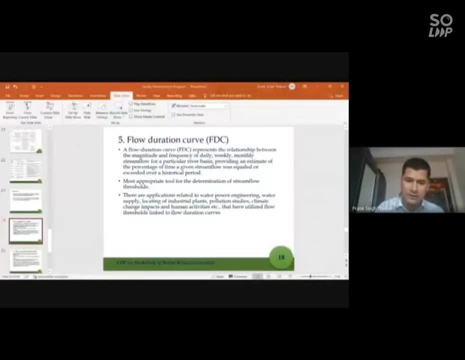 yeah, so how many of you are familiar to uh flow duration curve? okay, so flow duration curve so it has um. you know, flow duration curve has uh a significance in hydrological modeling because you can, you can, you can identify the flow threshold of the um, of the 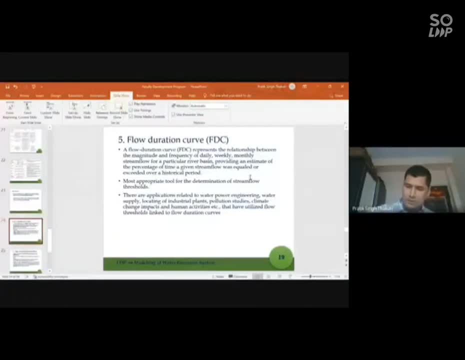 of the flow duration curve. so you can, you can identify the flow threshold of the um hydrograph. and you can, you can tally with the simulated um uh result of the uh hydrological model and see which regime or which which area of the flow hydrography is, or which area of the flow is uh giving a perfect result in the 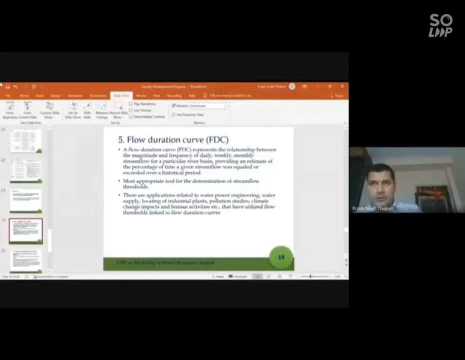 hydrological model modeling. if you, if you want, um, uh, uh, flood, um, you know model and uh. if the model is giving better result in the intermediate flow, um regime or the low flow reason, then this model cannot be good for uh flood hydrograph. or if you, if you want a model to be used, uh in the 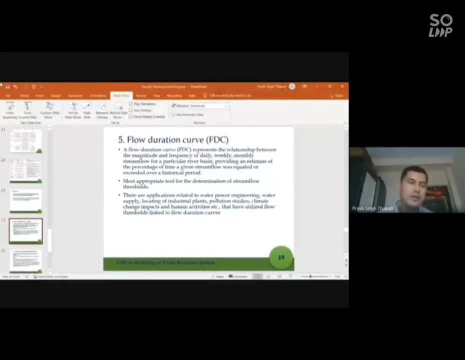 drought modeling, or, if you want model to be used for some water resource development process, uh, rather than flood modeling, uh, then you would rather go for intermediate flow or the low flow region and the your. your requirement for peak flow matching may not be as important as the intermediate. 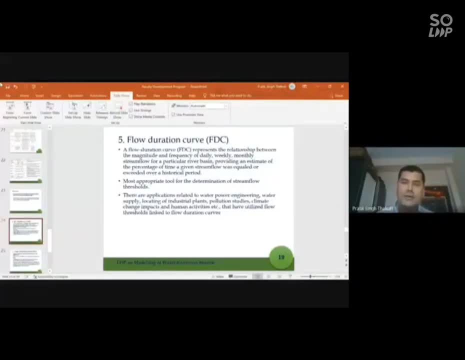 and uh low flow region. so flood hydrograph, you know flow, hydro flow duration curve matching is should also be considered and should also be um importantly, looked, while hydrological uh modeling is performed, uh, while hydrological modeling is performed, your, your hydrograph matching, and while you are matching your hydrograph uh or you are inspecting your, 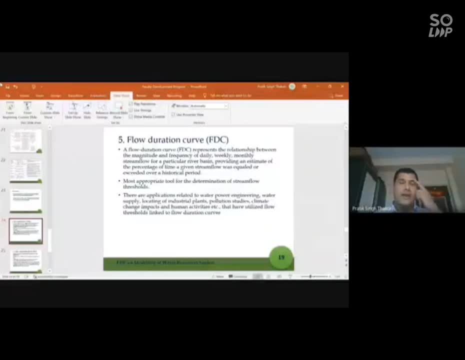 flow hydrograph, comparing your observed for hydrograph and uh simulated flow hydrograph. uh, you may not, you know, recognize if your intermediate flows are perfectly matching or not, or if your, your objective function, some kind sometimes, may not give clear picture. if your intermediate or low flows or high flows are matching, what is the condition of the flow regimes? but, uh, if you, if 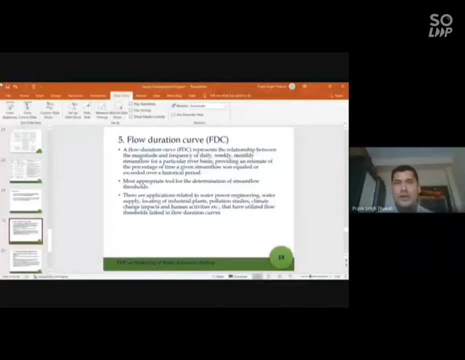 you try to, um, you know, compare the flow hydrograph between your, the observed, and the, uh, the simulated flow, and you will get a direct picture how, uh, your flow regimes are matching or not, which will be in which, if you represent, either it is high flow or intermediate flow, in which reason the model is 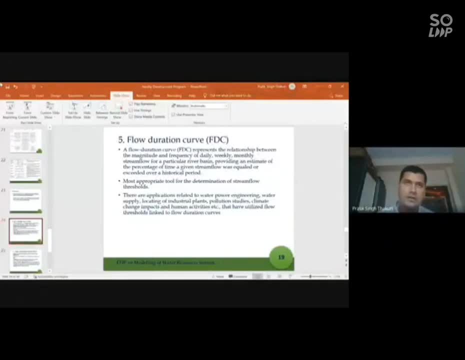 performing better or if your your purposes of the model is modeling is being fulfilled or not. that can be checked. so what is flow duration curve? flow duration curve represent the relationship between magnitude and the frequency of daily, weekly, monthly uh stream flow for a particular river basin, providing an estimate, um, of the percentage of time a given stream flow was. 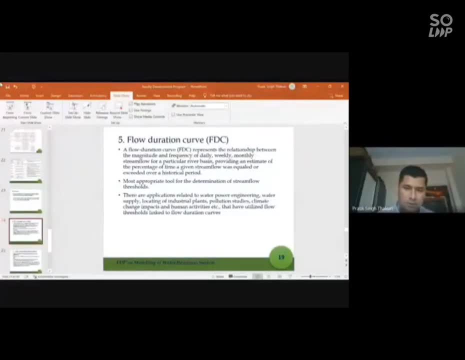 equaled or exceeded over the historical period. so the most appropriate uh tool, the flow hydrograph- you know the flow duration curve is also um- is the most important tool, appropriate tool for determination of uh stream flow threshold. so if you have um, a hydrograph, uh, you have a data. 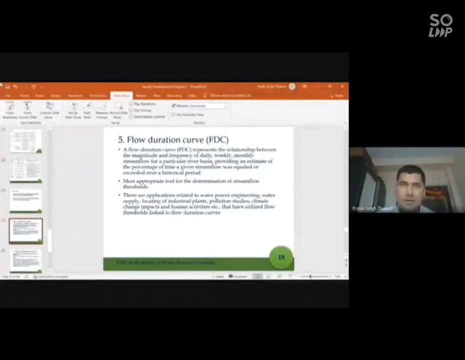 hydrological data and if you would like to, you know to classify your hydro, hydrograph or hydrological data into you know three um domain: high flow, medium flow or, uh, you know, low flow. then how would you do it? uh, so for this um, you know giving the threshold, 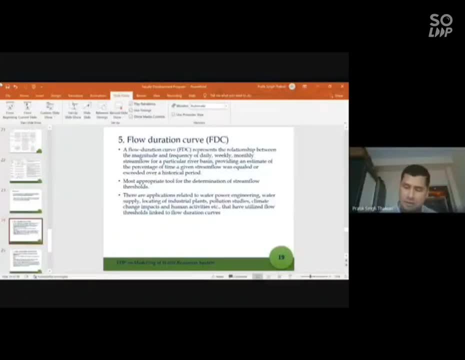 for uh flow regime. the flow duration curve is a very appropriate tool. so there are application related uh water power engineering, water supply, uh locating industrial plants. you know the uh pollution studies. climate change impacts human activities so the flow duration curve has a lot of activities and especially nowadays the flow duration curve are being used and preferred in. 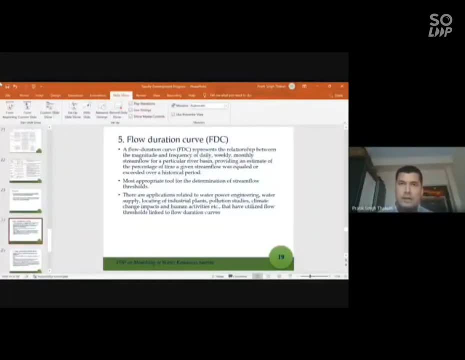 the environmental flow uh requirements. you know, in the, in the mountainous europe areas there, especially in nepal or the northeast of india or bhutan, there have been a lot of hydropower development and the the environmental flow requirement or guidelines are required. so for the 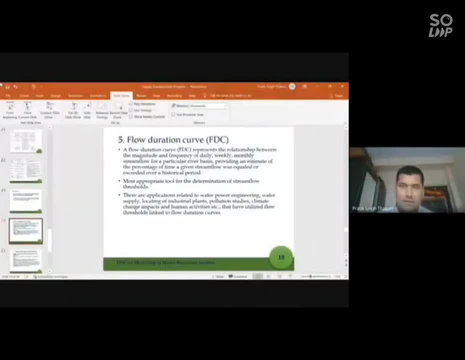 those conditions. you know the flow duration curves, uh, give, uh, you know you would solve as a tool for data determining streamflow threshold. you can determine that the 10 threshold of this stream flow is low flow. so you should at least preserve the low flow condition or the intermediate flow condition. so yes, 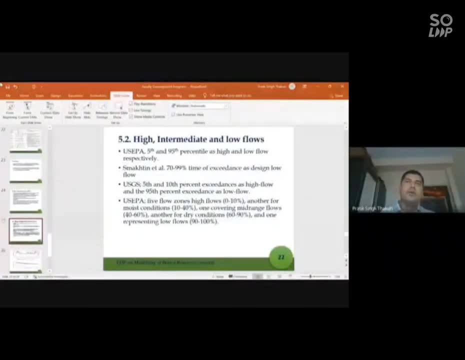 so what is? how much percentage of the flow is high flow? how much percentage of the flow is the low? that is still not, I know, the clear. so the US EPA says that the flow that exceed fifth percentile and is high flow and the flow that actually 95 percentile. 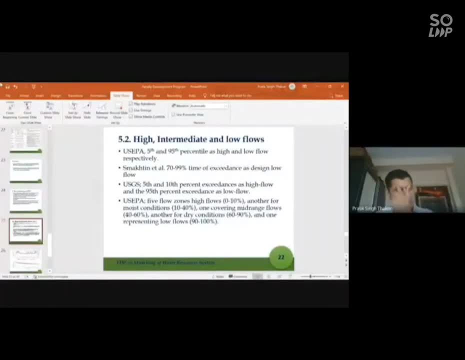 is low flow, you know, and a researcher, the Russian researcher, did a study of a nebulous river basin and other saltation river basin and you know said that like 70 to 99 percent of time of accidents would be considered as a low flow condition. similarly, United States Geographical Survey, have you know. 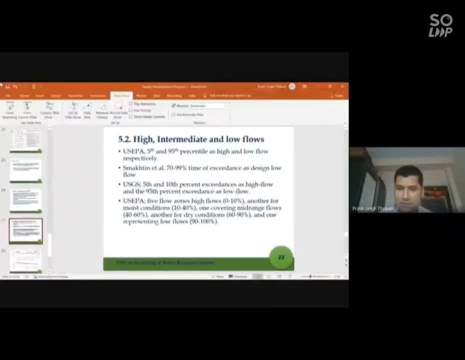 conducted a research and said that five, fifth and ten percent percent of accidents as a high flow and 95 percent accidents as a low flow. but they have also said that it can vary as per the watershed condition and US EPA. further, you know, divided flow condition into five flow region. number one condition is: 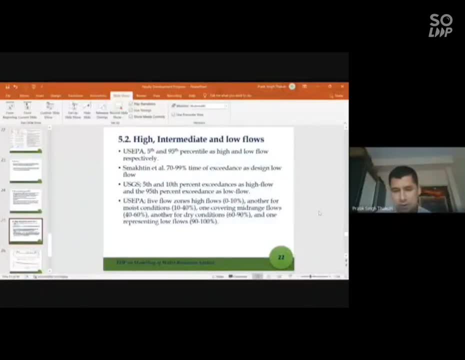 the low flow condition and the low flow condition is the low flow condition and you know high flow, that would be 0 to 10 percent of percent of of time of accident and that is called high flow. and the another condition is the moist condition, that would be 10 to 40 percent of the percent of time of accidents. 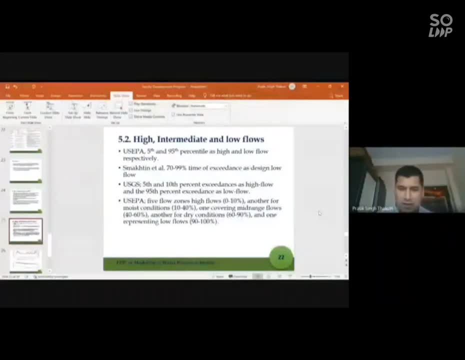 similarly, mid-range flow that would be 40 to 60 percent and dry conditions 60 to 90 and the local condition 90 to 100. so there are a lot of you know, standardization or guideline that says that what the high flow, low flow or 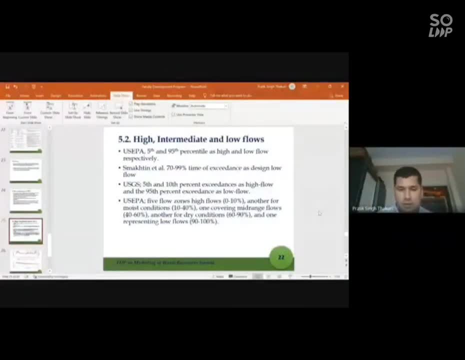 intermediate flow should be but but it may vary from watershed to watershed. the high flow of your watershed or the high flow of other watershed may vary, so it should also be rationally selected. what is the high flow condition of your watershed or your hydrograph? in my study I'll give you example of my modeling study I have carried out and the here I'm showing. 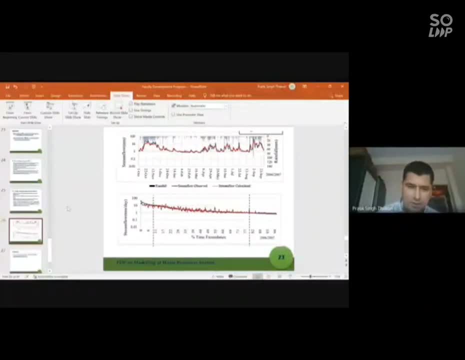 this is the. this is a, a watershed in Sri Lanka, uh called elagawa watershed, and the hydrograph of 2006 and seven. this is the hydrograph of 2006 and seven and I have used. I did a modeling study there using stormwater management model and uh 2006 and seven for the year 2006. 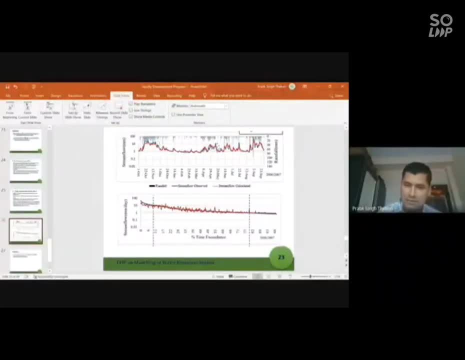 and you can clearly see uh the good matching of the hydrograph in the all reasons. but uh, here, if you see the flow duration curve, uh the the high flow region where in my my study I have considered uh the flow region above 10 percent percentage time of accidents is considered high and the 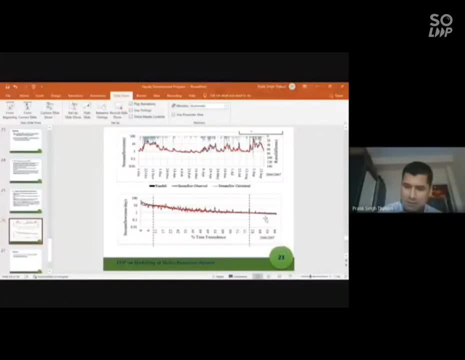 flow regions: uh, 80 percent time of accidents. low and between: is the intermediate or the medium flow? here you can see the high flow are thoroughly being underestimated by the model, whereas low flows are being overestimated and the intermediate flows are being fairly stimulated by the model. so 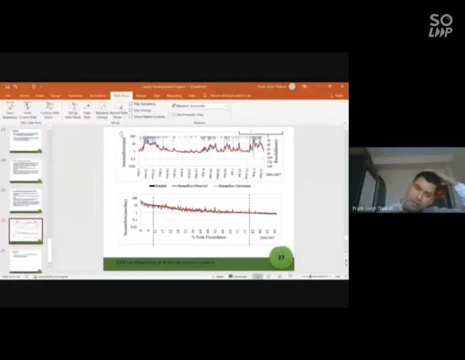 I could conclude that this model, my model or my modeling- uh work. did not uh work good for flood management uh or flood modeling process. rather, it would be good for some water resources development project or water resources management project. so it did not work good for uh flood management or flood control project. so, depending upon your engineering, 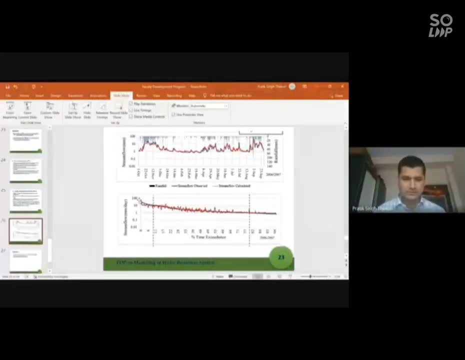 application or the purpose of the study. uh, your hydrological uh model and this flow duration curve would you know, serve a tool, you know, for how and which uh don't regime of the um hydrograph is being, uh, you know, modeled fairly or roughly or bad, so I'd like to share um the across. another reference by a professor. 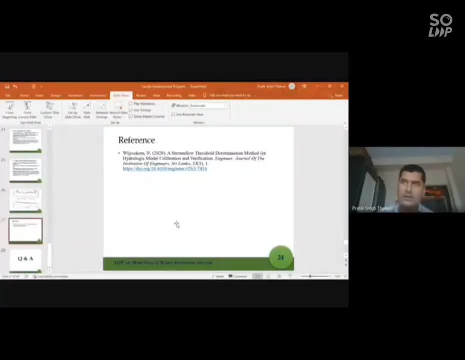 uh. so on which you say he was my supervisor in in Sri Lanka and he had authored um uh, a paper called a stream for threshold determination method for hydrological model calibration and simulation in engineers journal of Institute of engineers, Sri Lanka. I will have, clearly, you know. 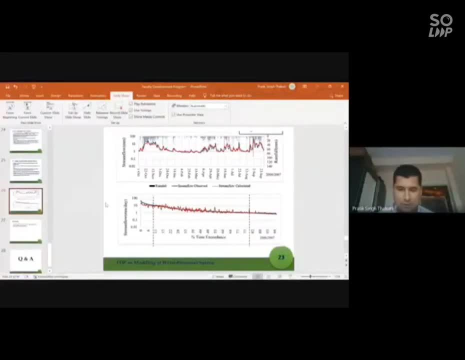 given the process, how you can, uh, you know, classify the threshold or give, you know, estimate the threshold of the hydrograph to high, medium and low flows, or you can just, you know, look at, inspect at the your hydrograph and the flow duration curve and give high and medium and low. so generally it 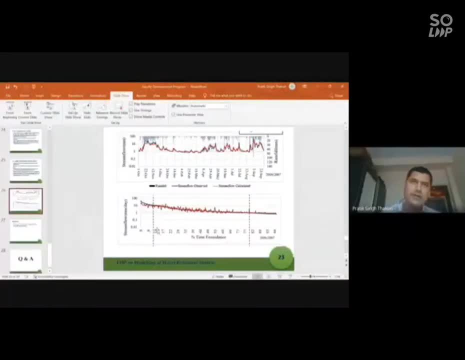 is considered that that the uh zero to ten percent is considered as the high flow, 10 to 80 percentage as the medium or intermediate flow and 80 to 100 percentage percentage time of accidents is called low. so this is the reference and I would like to, if the participants 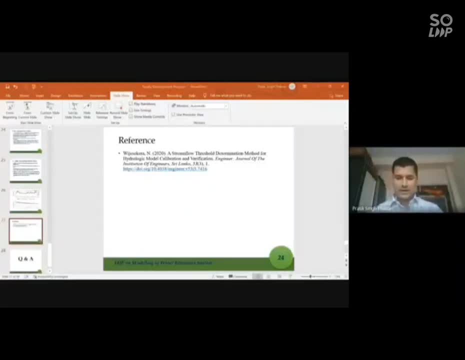 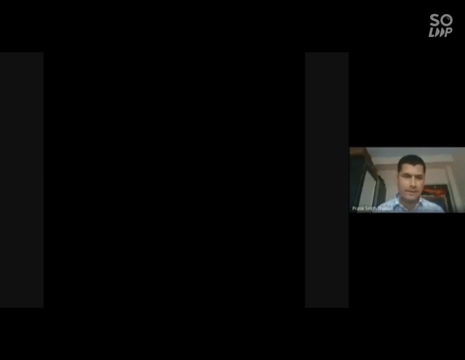 are not familiar in four duration curve. I can. I can share you the spreadsheet calculation after this ledger. I just, yes, so I'm just doing a spreadsheet calculation. we have calculating it and showing it you, you all, and i'll also share you the spreadsheet and you can. 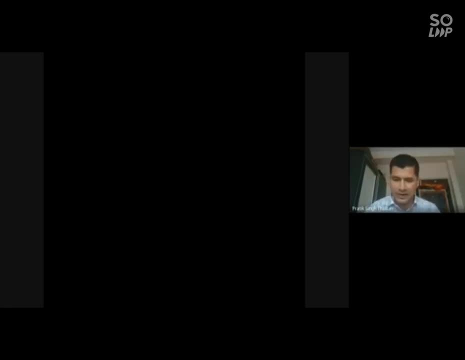 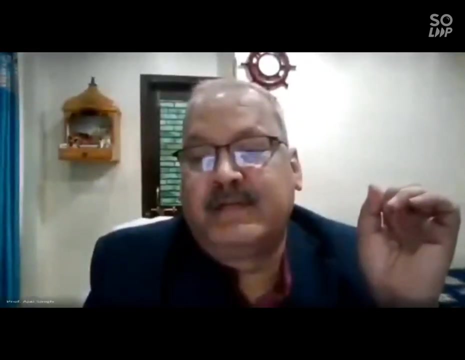 you can try it. you're on your own. uh, after looking at this flow duration calculation. so this is um. yes, the spreadsheet is visible. no, it's not. is it visible now? it's not visible to me, okay, so stop sharing. i think it's visible, all right. 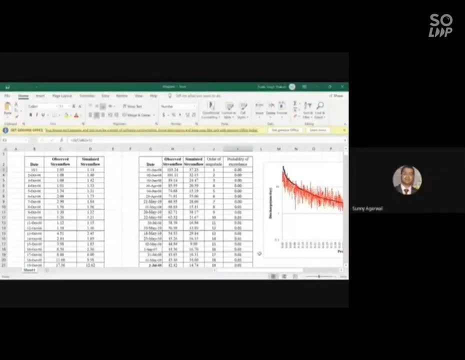 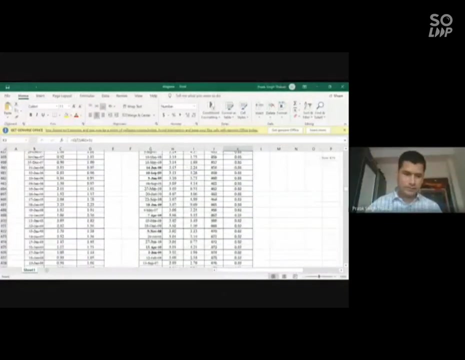 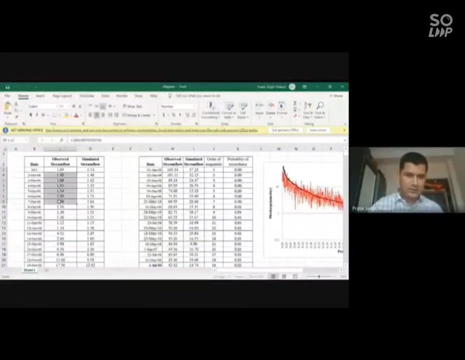 yeah, so what i have done is i have the data from 2006 to 2010.. this is this was the four-year data for calibration of my model and this is my the observed streamflow data. you know the observed water yield, especially in specific in mm per day. so this was the observed 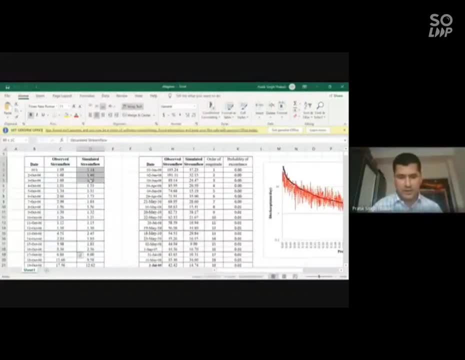 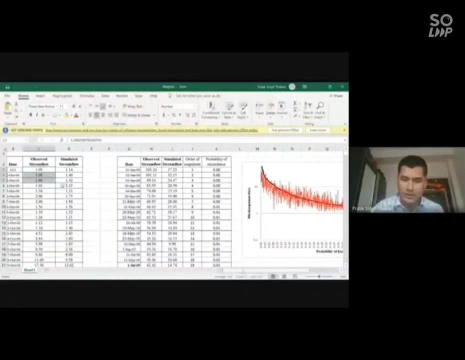 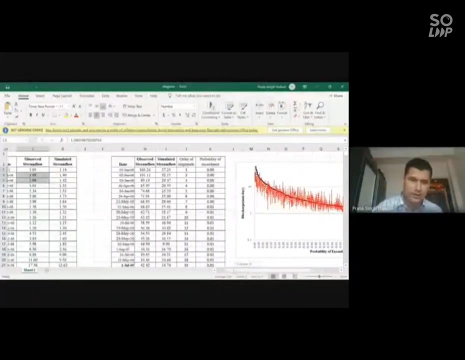 water yield of my watershed and this is the simulated water level of my uh watershed. so how would i draw a flow duration curve of this watershed, this hydrograph, and compare with my simulated streamflow data, simulated water data? so what i did, was i just what i did? was i just arranged this high? 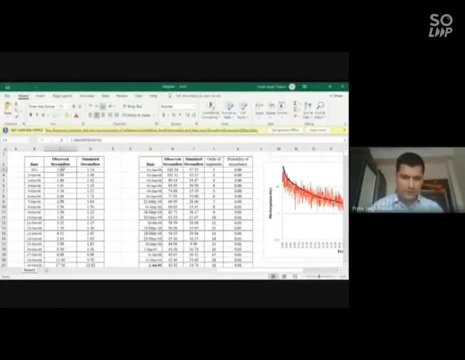 my observed streamflow data. just selected all these of these and arranged it in a ascending to descending form, that is largest or smallest, and the corresponding date and the corresponding stream flow is also corresponding stream flow. so the simulated stream flow is also changed. so, yes, the high. 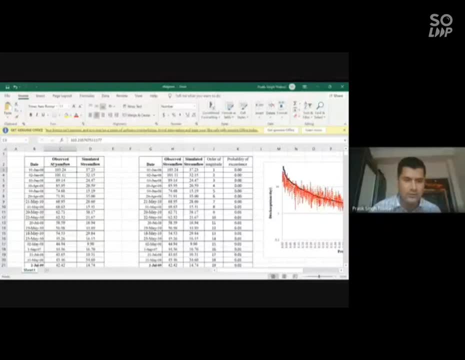 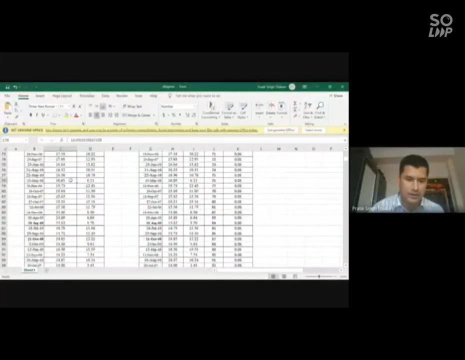 highest stream flow. i just observed streamflow, or i observed water was 103 mm per day, whereas the corresponding high streamflow, or the water at least, only 37. so you can see the. my model was very badly estimating the, the higher flow region, whereas if you go in the lower domain of the, in the intermediate 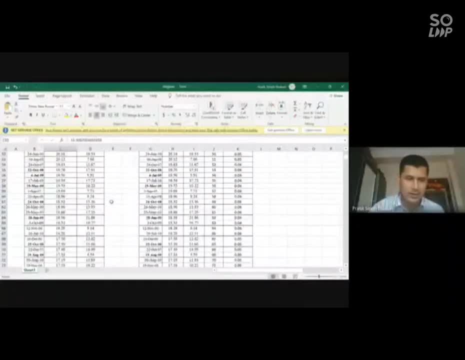 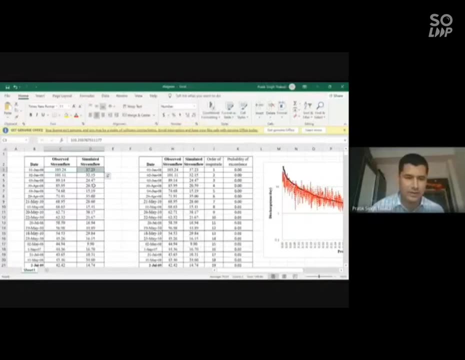 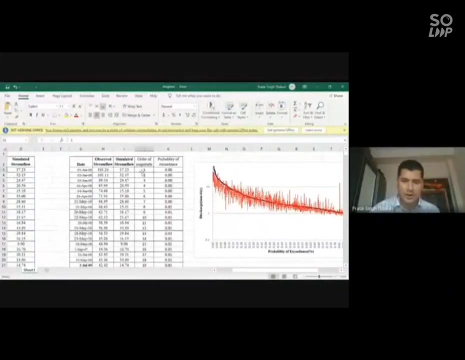 flow. it is fairly estimating here. so you can, just looking at the values, you can just, you know, get the idea that the high flow reasons are not being properly estimated by the model. now, what i did was what i did was i gave the order of magnitude from one to. there are 100, 1461 data, so i gave the order. 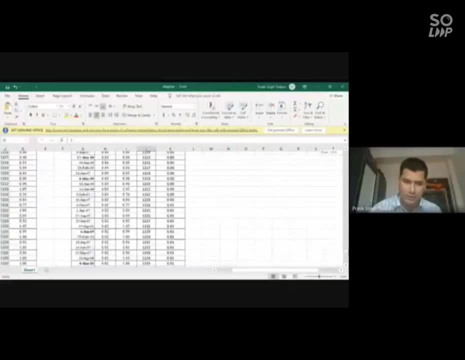 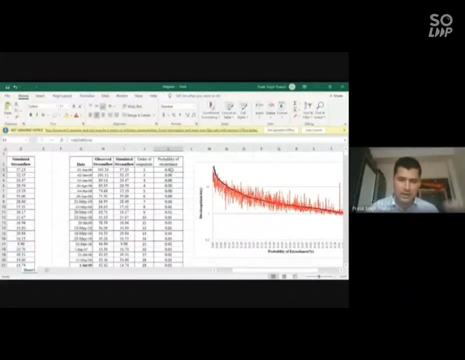 one to one and one thousand four hundred and sixty one. now you can calculate the probability of the accident. the probability, the formula, is this: the flow, this flow uh, which is 103, occurs only occurred only one time. so the probability of occurring it, uh, in the flow hydrograph or in the in the data is like almost zero, whereas 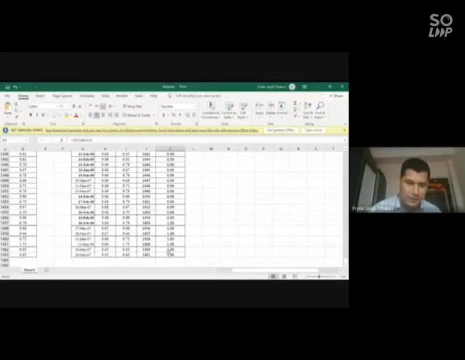 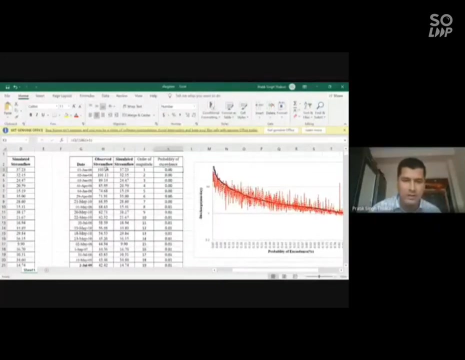 this 0.65 mm per day occurred almost. you know the value above this are almost all. so this, the probability of occurring this flow, is almost 100. so this way i calculated the probability of accident. the formula is the order of magnitude divided by the number of the data and if it is in 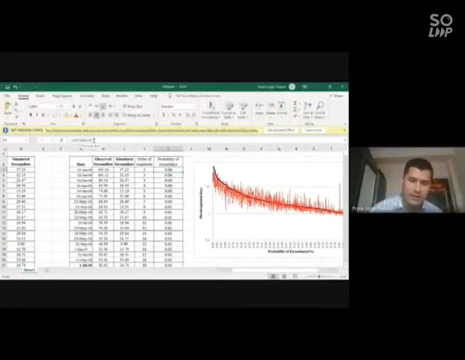 it is, or you can just add one, uh, and make it even. it is even, just leave it so. number of the number of data in the time series. my number of data in my time series was 1461 for four years and, and it is odd, so i added one, and this is the probability of accident. so 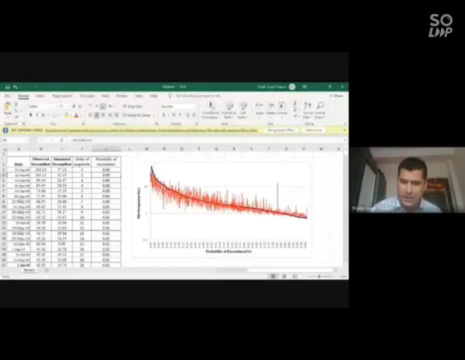 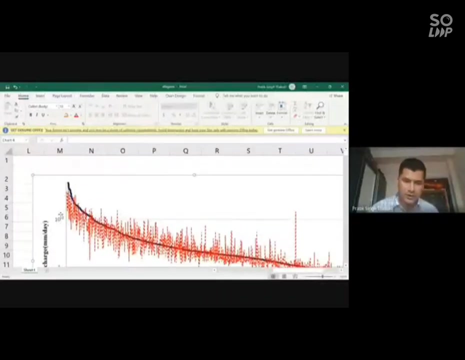 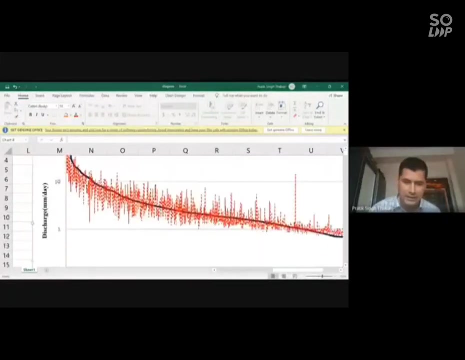 i plotted it. the order, the. this is object and and the corresponding stream flow. so you can see that in the, if i magnify it, this is 106.7. please Should i magnify it? okay, let's see. uh, yeah, if i magnify it, and, and this is in the logarithmic scale. 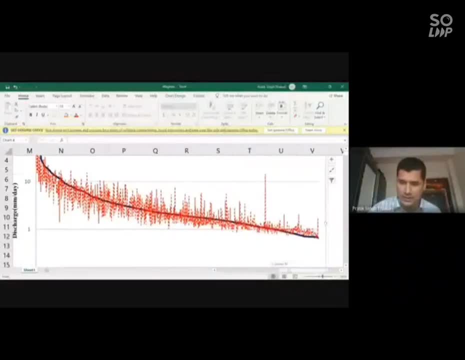 to see the data in. visualize the data in in the the magnified version. so if i magnify it, i can see that the higher flow regions are not being properly estimated and the no underestimated estimated. so this cannot be, you know, shown through your objective function or 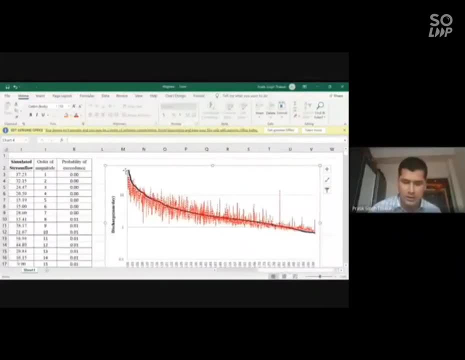 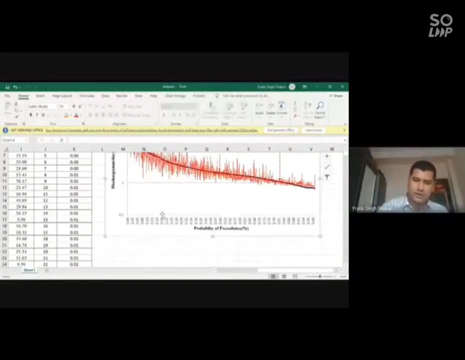 your hydrograph comparison so for you to you know, see how well which resin of the watershed is being properly modeled, or you know to ensure that your high flow regions are being properly modeled or not. you have to go to this flow duration curve and visualize and inspect if your model is giving fair result in the all. 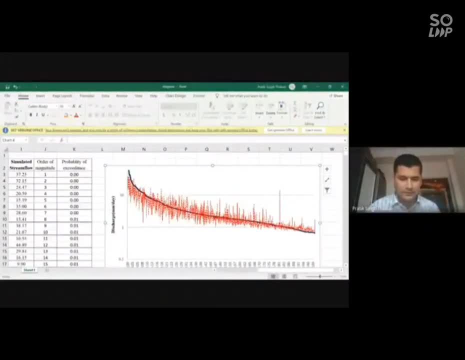 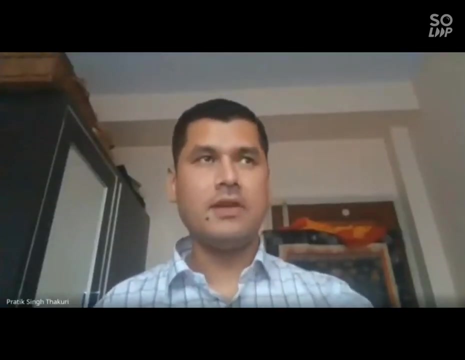 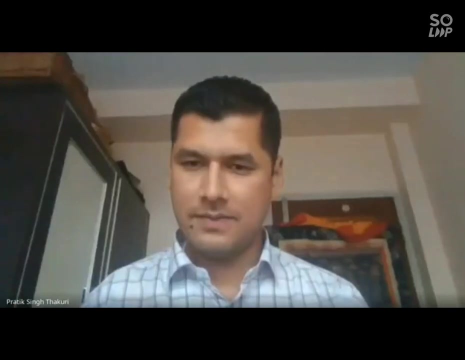 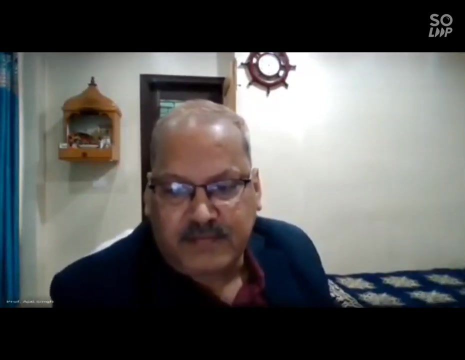 the flow, regions or desired for regions or not. with this I have come to the end of my presentation and if you have any question, yes, so I have come to the end of my presentation. so if the participant have any question, so I'll be answering any question please, especially mr Pateek. 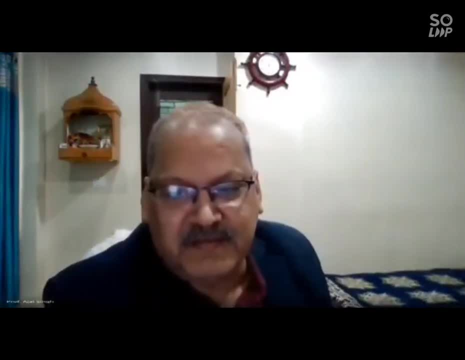 we. we do not use the flow duration curve. you know that logical, that modeling studies, but it's quite good that that's a better way to see how the high flows and low flows are matching. so this is quite interesting. yeah, normally Configurator USA we are using to to estimate the environmental flows in. 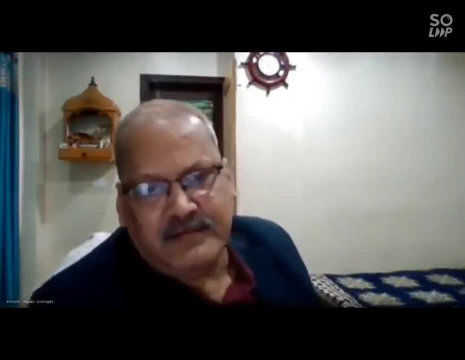 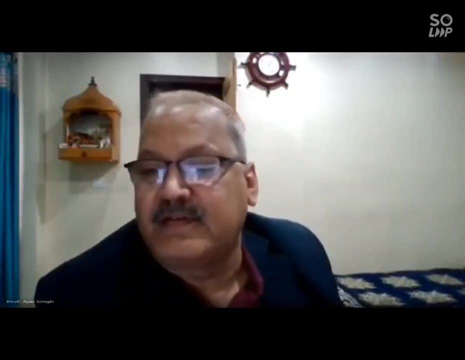 the region. we have been using this any. any questions from the participants are still there. there someone, the Bourbon, is asking: can we userobe言 sempre? us symbols? London, undefined. yeah, usually you will use fdc to calculate honor mark of data legally. yeah, you can, you can, you can. 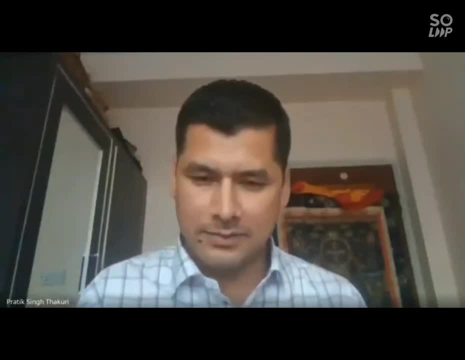 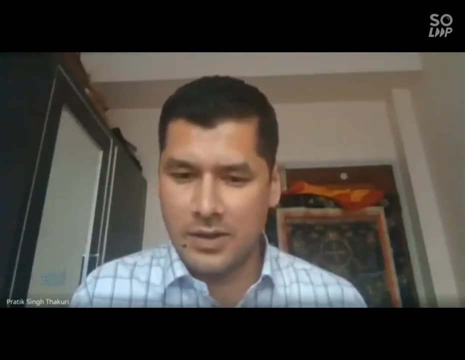 calculate fdc just for online data and you know I didn't Me shell students, few cents and other data while observed data, but uh, uh, the uh. in my presentation i would. i said that, uh, you know you can see if your model is giving uh clear. you know that if your model is estimating uh, uh, the flow regimes, 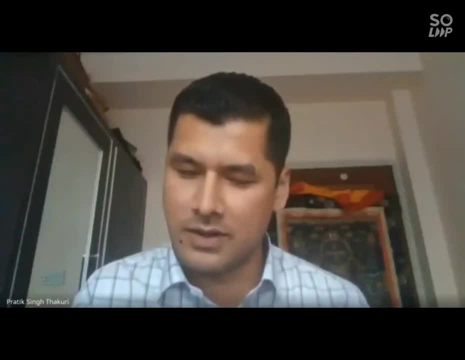 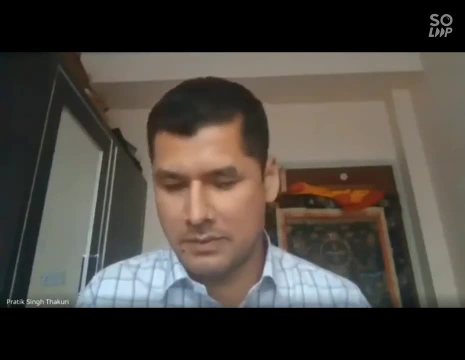 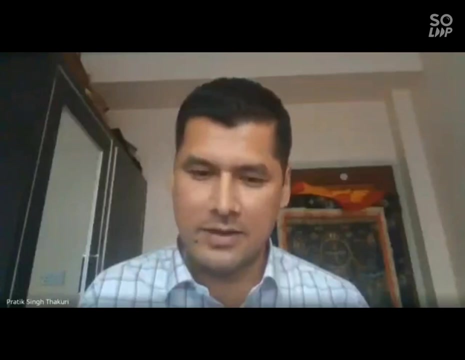 or to to to verify the model result in all the flow regime. uh, your your purpose that this? this is an additional purpose the fdc can serve. so, just before the professor, as i said, that he is to use fdc just for the observed data, for environmental flow consideration or for separating the flow. 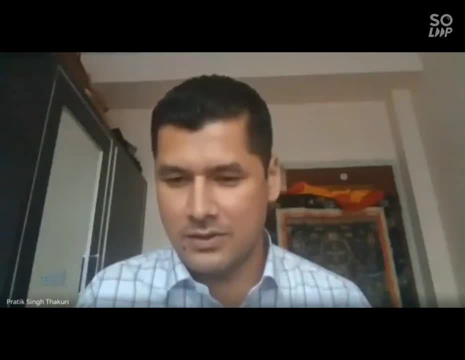 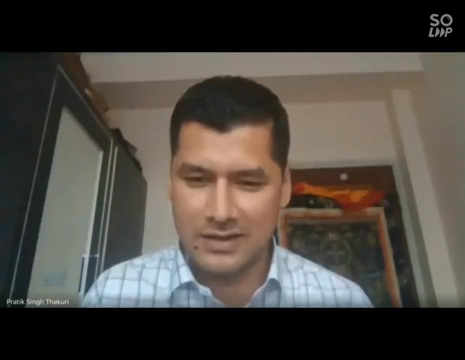 threshold in the, in the watershed, in the flow hydrograph. so, yes, you can only calculate the flow duration curve for observed data. that is what being done initially, but this is another area of you know, the engineering or in hydrology i'm describing in my presentation. it is, it is. it is always better to use the fdc for the. 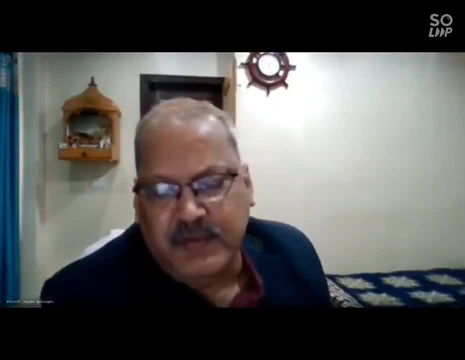 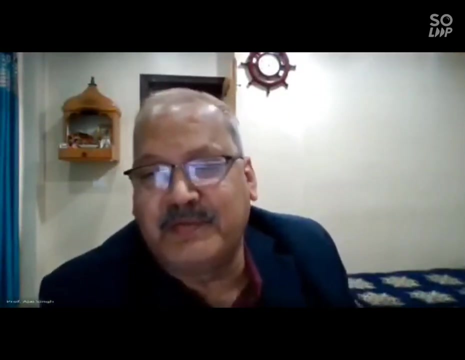 that are predicted values also, because ultimately this is going to give you the incidence of probability, which is quite informative it is good to use with predicted values also, you can use both. so someone is quite attentive during the whole uh program. yeah, that's good someone, what you are doing. 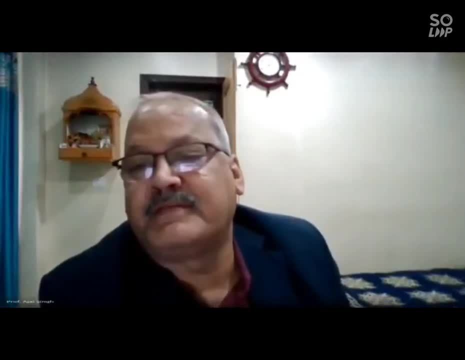 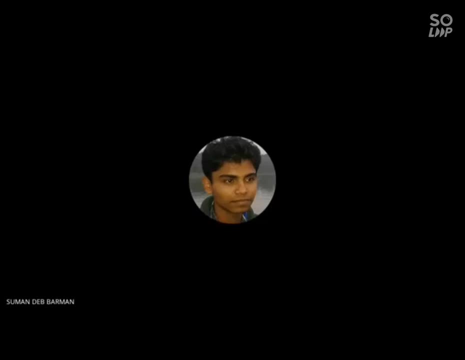 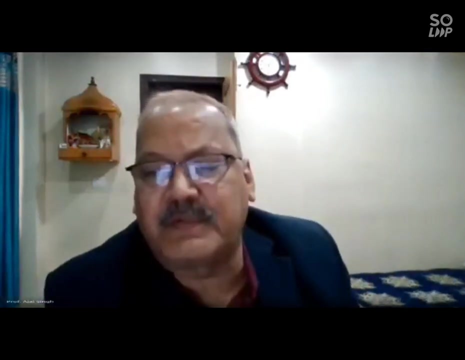 are you a student or you are at a job? yes, sir, student, sir student. yeah, geographic background and my research area, mainly fluvial geomorphology. fluvial geomorphology, that's quite interesting. this program is quite good for you. so you, you are master student or you are doing phd. 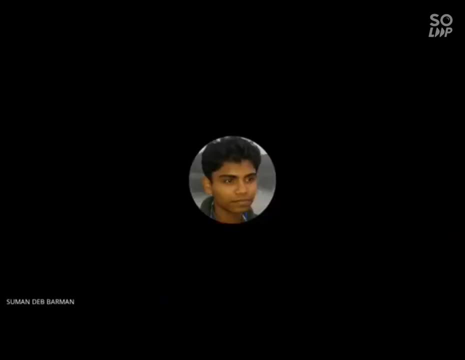 sir, my phd sir, masters have completed 2015.. from which university you're doing, sir? the university of burdwan, burdwan, west bangalore. yes, sir, good, very nice sir. one, one question, another. you were mentioned: the calculate this threshold, determine the stream. 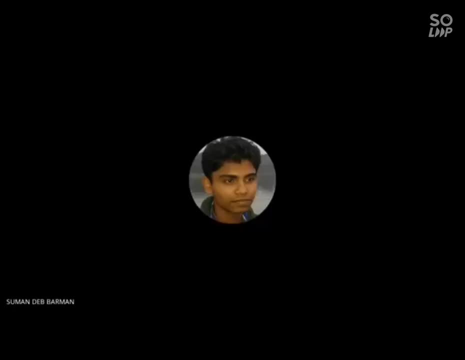 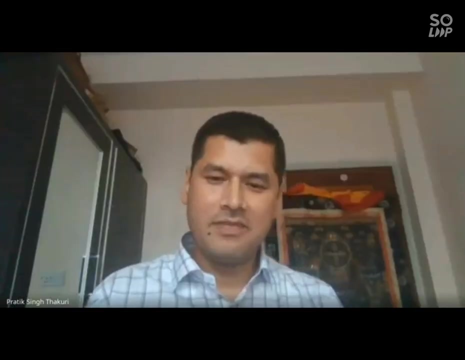 flow threshold like others parameter. where can i apply different statistical tools to identify this threshold? in that case, this only probability. i didn't get your question. can you repeat it please, sir? in our geographical research for the other parameter we are calculate the threshold value but three and commission matching時間, so it is not happening: delay and more. 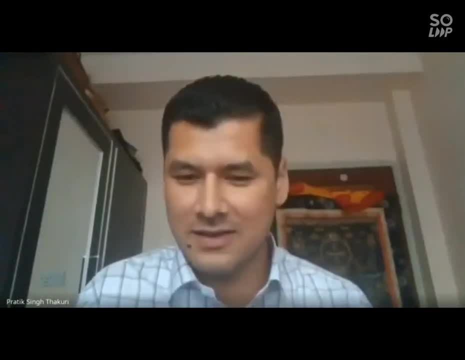 so small flow time of the flow duration are, uh, these are, oh i don't know, the Pixel a little bit long or a longer. one result that some. so one question i think there are some people are asking: does rington state test dreams will require a flow duration curve? how to calculate from the current flow that honestly, i like your ten percent in and out, because if you are not familiar with the flow, possible kind of things, you have to calculate percentile from para constant and sun value, like your 10 percent, 90 percent, yes, yes. 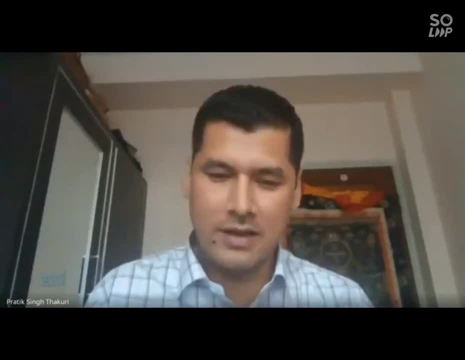 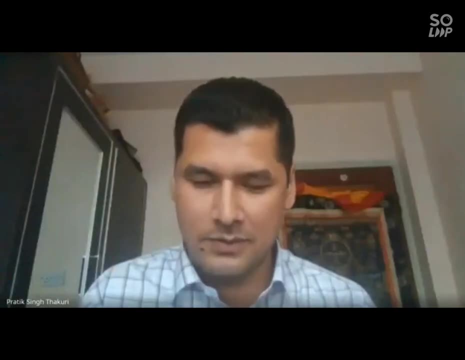 the researchers. they go to the literature by the agencies like USEP or USGS. they have the general trend of taking 10% as a low flow and 10% as a high flow, 80% as a low. So that is. 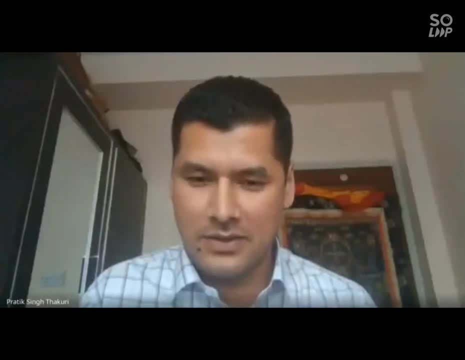 the trend. But there is a paper, there is a process that says that how detailed you can go through the spreadsheet and calculate each and everything and rationally select high flow, low flow and intermediate flow And that would be specific just for your watershed. There is a 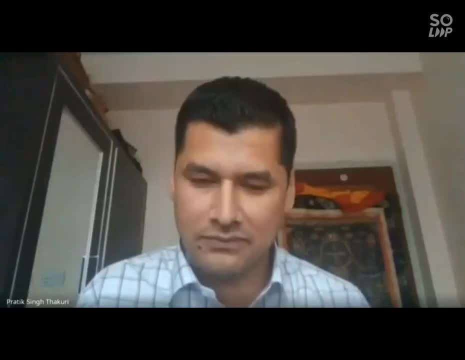 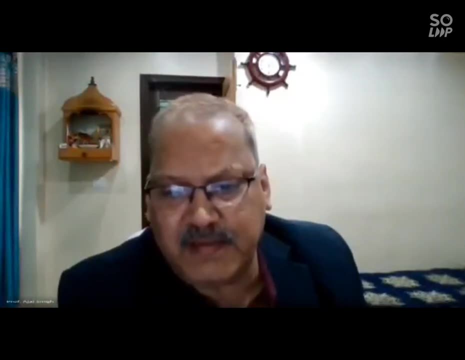 process. yes, You have to go through that paper. Yes, I would like to add: a threshold is going to be decided by the project, your overall mandate, for which you are working. If you are planning some irrigation system design that it may go up to the 90%. 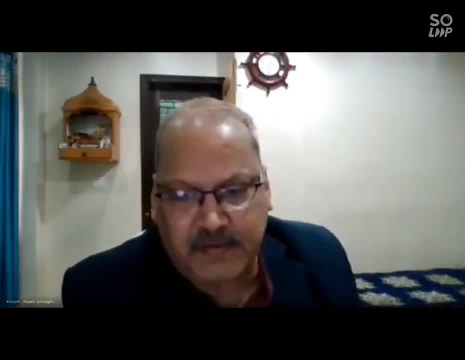 or like that. That particular flow will have the probability of 90%. So with this you can plan the irrigation system. So it depends upon that overall, that objective of the program also, Is it true, Mr Pratik? Yeah, yeah, So I think with this let us close this session. 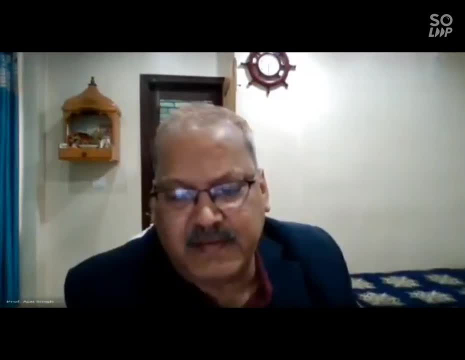 And very nice lecture was delivered by Mr Pratik, Very interesting. especially. I found that it was quite interesting to hear that statistical measures and its interpretation that the flow duration curve was quite interesting for me also. Very informative session, sir, And we 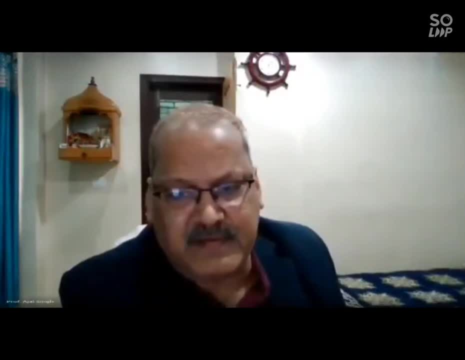 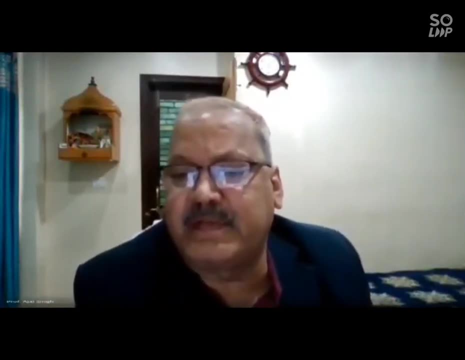 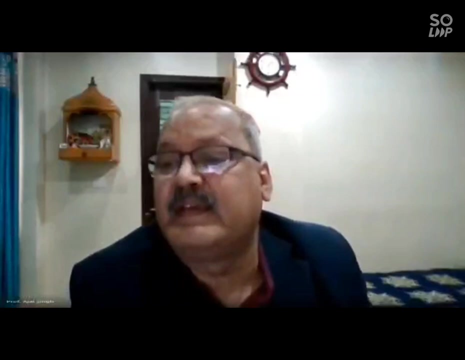 thank that you agreed to deliver the lecture in the FDP organized by Central University and AICT. We are very honored And I would like- I just requested that one of the participants to say- to extend thanks on behalf of all the participants. I think there needs to be a discussion. 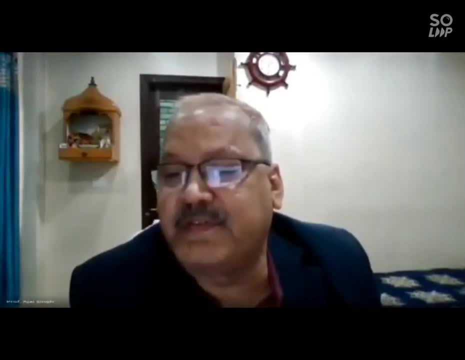 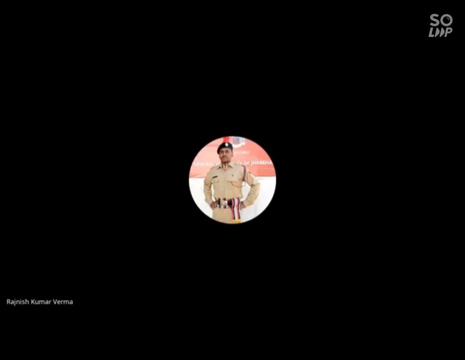 I think Rajneesh Kumar Verma has agreed. I'll request him to say a few words. Rajneesh, You can put on the camera and please say something. Yes sir, Yes, Rajneesh, Yes sir, Good afternoon sir. 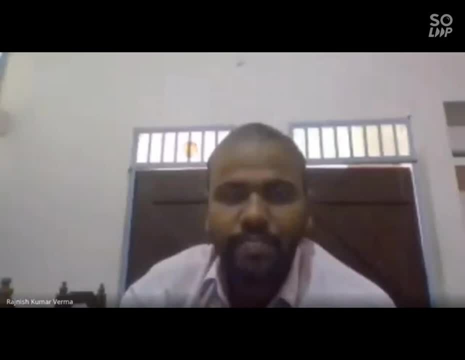 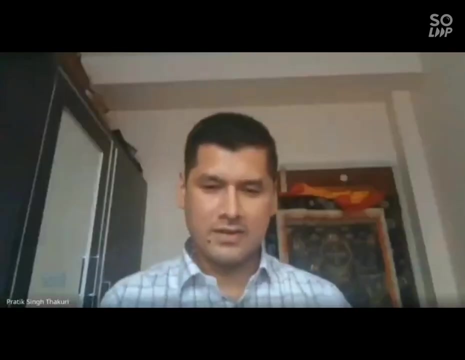 Good afternoon, Good afternoon. I would like to thank Mr Pratik Singh Thakuri on behalf of all the participants for his very informative lecture. The whole lecture was quite impressive and content valuable information. it will help in our research work. thank you, sir. thank you, so he, he is one of the participants. 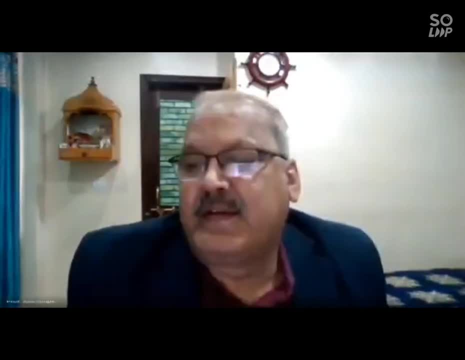 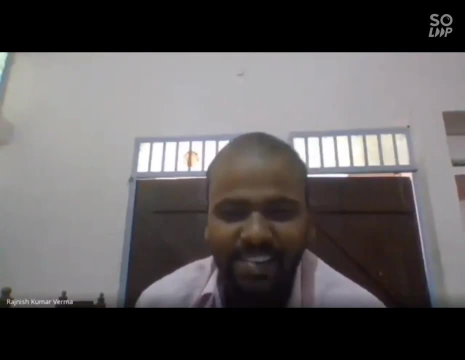 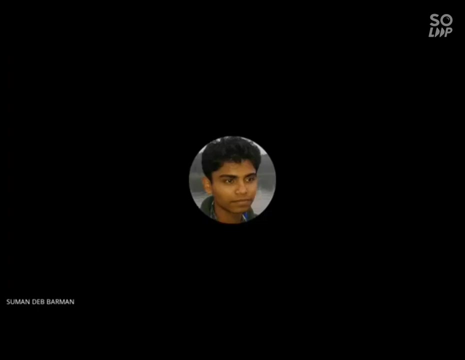 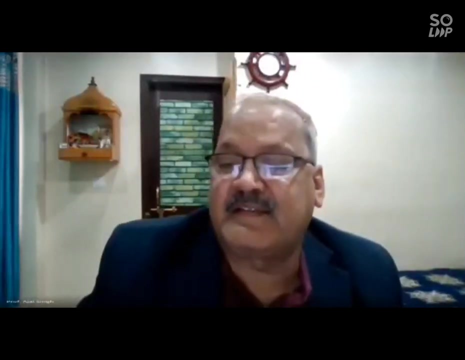 and uh, thank you for this, and you are from the police force or the defense? no, sir, actually. uh, that was my lcc photo. i've done lcc, uh, and make all these characters. okay, yes, sir, okay, hello, sir is also writing. thank you, sir. praveen kumar has also extended. yes, yeah, thank you everyone. 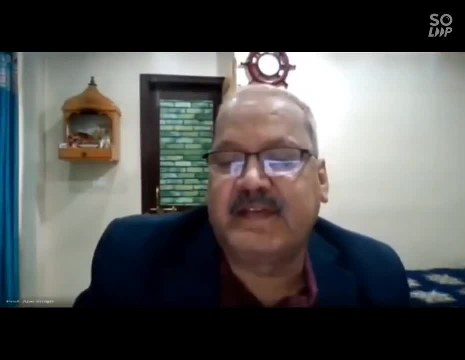 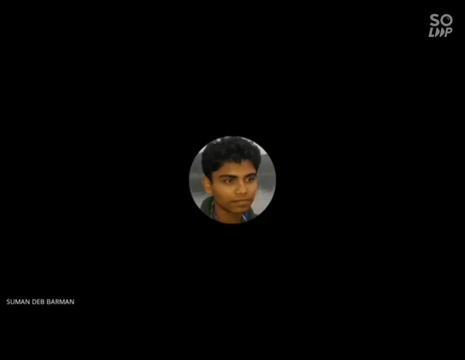 and thank you. yeah, okay, mr prateek. yeah, with this we are going to close this session and resume that three o'clock. yes, yes, last one, sir. i'm one question, sir for getting different discharge and sediment data of nepal, how to get as an indian research scholar? 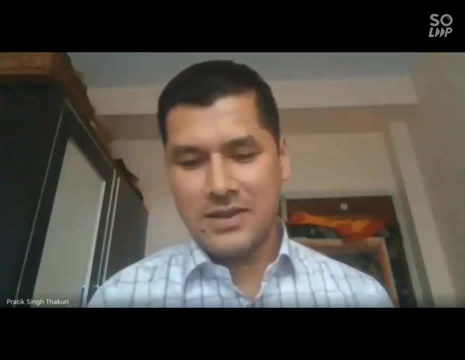 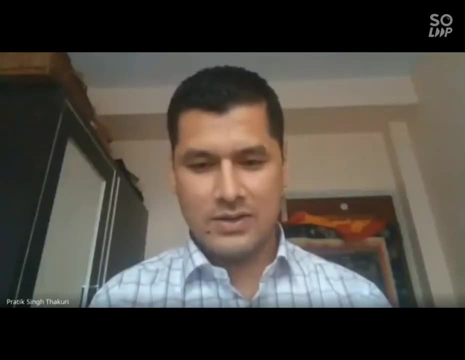 okay, you would like a discharge and sediment. you know the discharge data. you can, uh, you can go to the website of the department of hydrology and meteorology and you can just put a query and they'll give you the available discharge and precipitation data. uh information. the 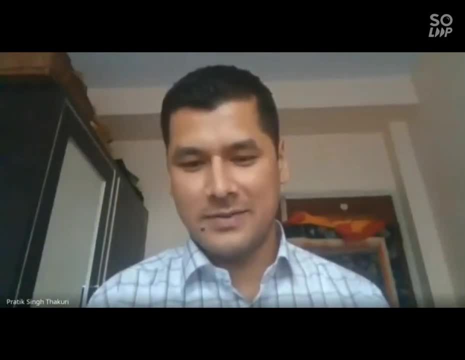 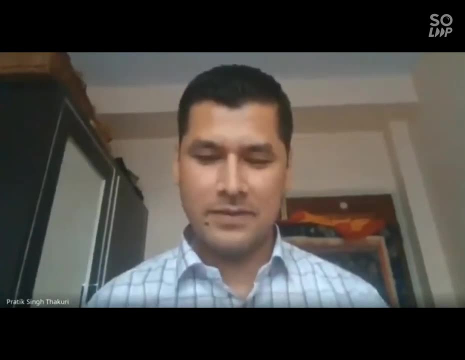 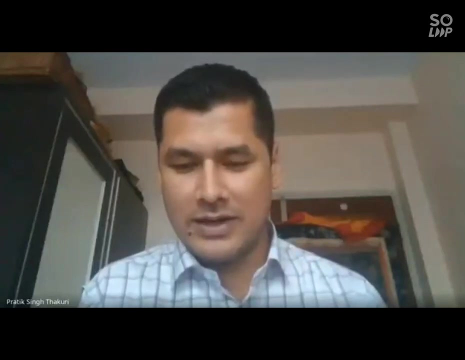 availability, just, and then you have to. you have to write uh, the, the data time series, which data span you like, then they'll estimate the budget uh of the uh data. you need to pay for it. then if, after paying uh you, you will be able to get it, but yeah. 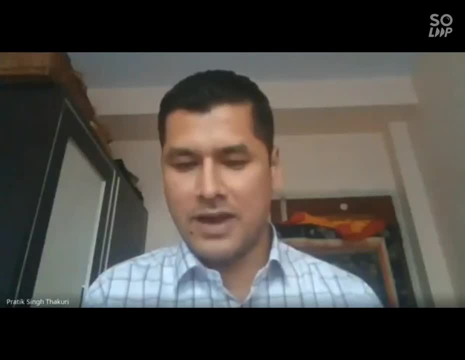 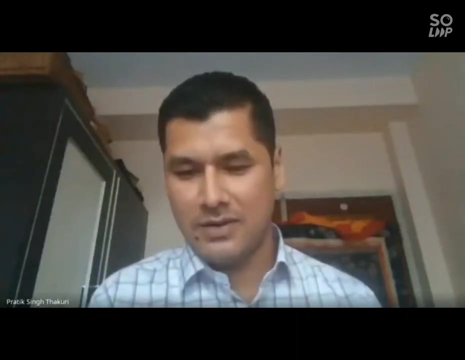 it's available in the website of department of hydrogen. it's called dhm and the sediment data. that is not being collected by any one in agency. it is being collected by the projects- hydropower projects or other hydropower dam projects. so it's scattered. it really needs uh. 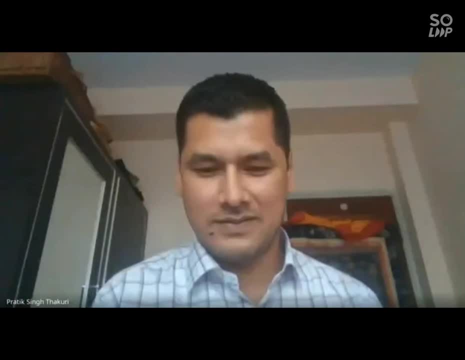 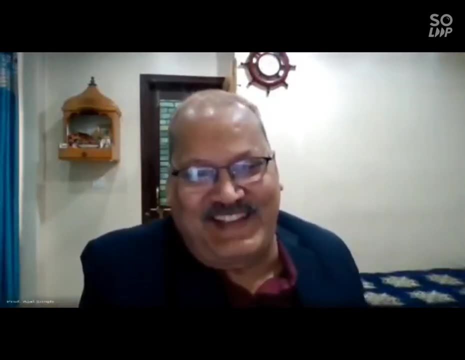 for work to be, you know, done, or else, the most easiest way, that you can, include mr patik as your supervisor, someone that that you can. you can, uh, that you can explore whether he can be added as a co-guide in your dissertation program or not. so if he does, then he will make you available all the data. 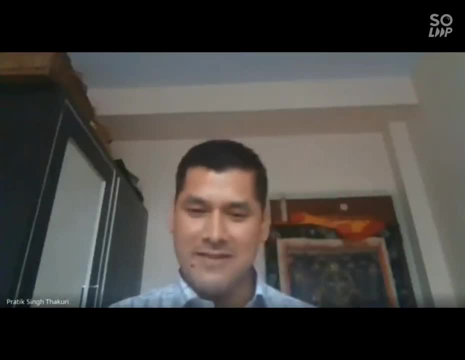 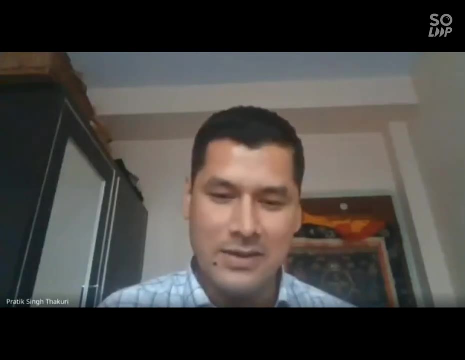 yeah, sure, so yeah, if any participant have any further queries or you know um they would like any suggestion or they have any problem or they would like my suggestion, then you can email me and i have provided my email address in my presentation. i'll say i'll. 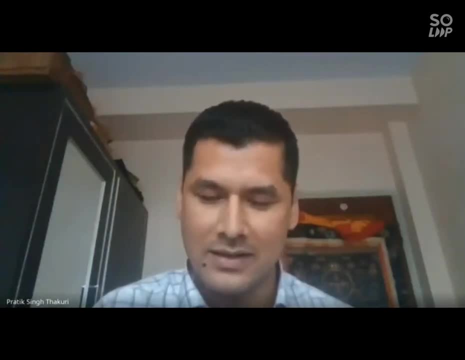 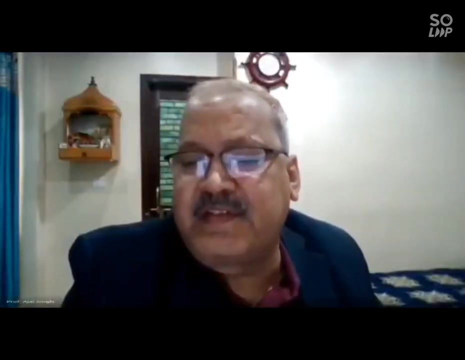 be sharing my presentation slide to professor azay and he'll be circulating, i think. yeah, and you can always, always email me and i'll be. you know, i'll try to help as possible. yeah, okay, okay, so thank you very much. so with this, we will close the session here and we will again.